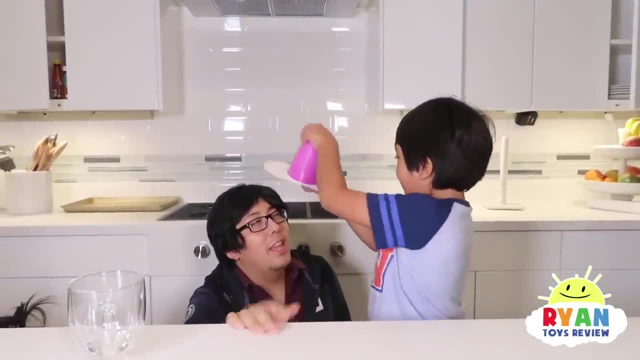 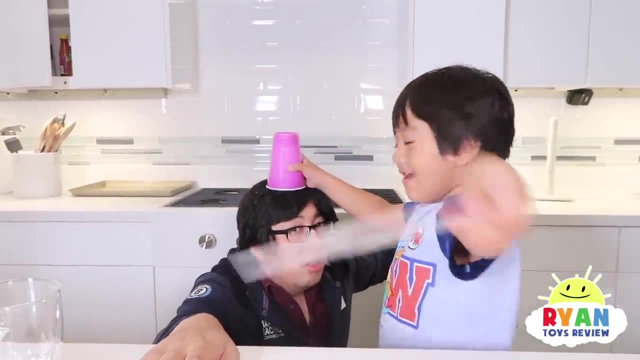 Do you trust Ryan? No, I don't trust Ryan. They're tripping already. Do you trust Ryan? No, I'm going to put my phone. I'm going to put my phone. Three, two, one, What Ryan? 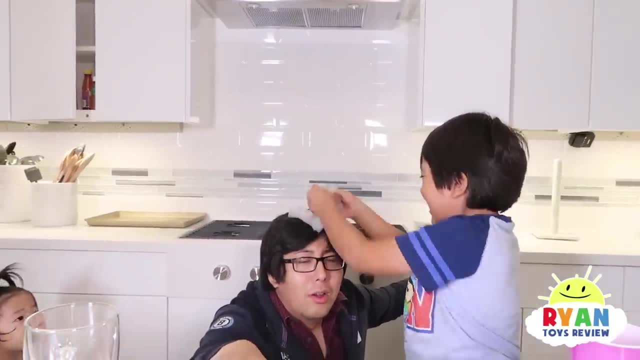 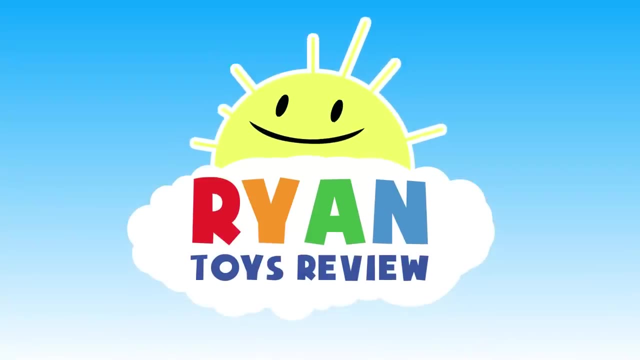 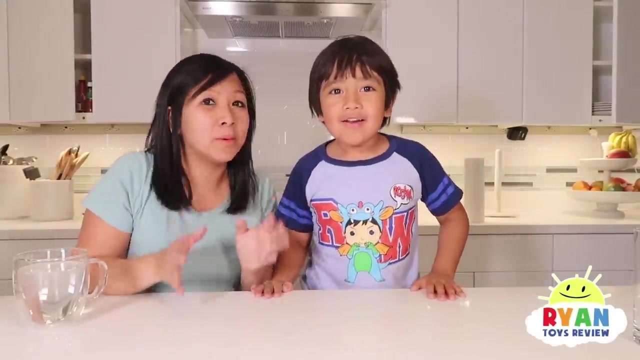 Ryan, Ryan, Welcome to Ryan's Toy Review. Hi everybody, welcome to Ryan's Toy Review. Today I'm going to show Ryan something really really cool. Are you ready? But can you trust me? Yes, it's your friend. 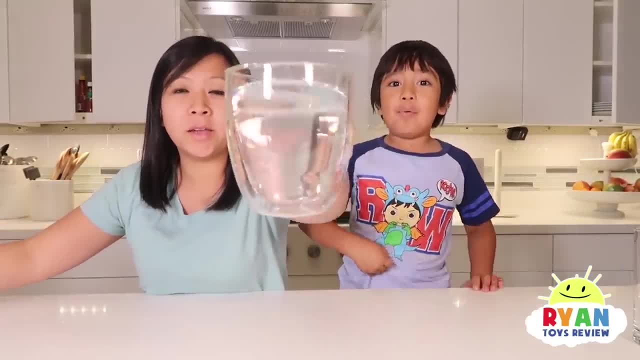 Alright, so here's what's going to happen. okay, I got a glass of water. You see a glass of water there, But it's from the sink. Yeah, so, sink, glass of water. I have a cup here. 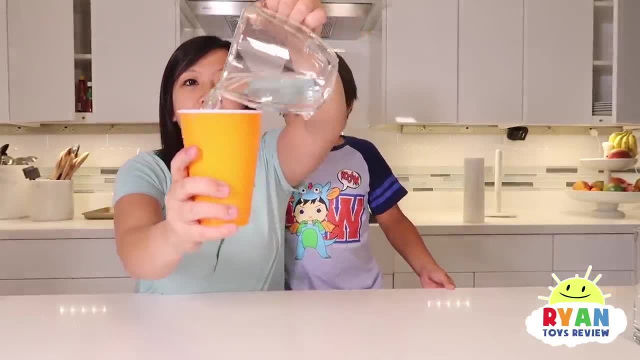 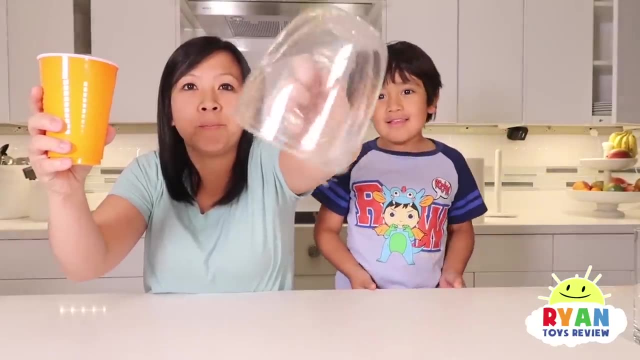 I'm going to pour this glass of water in the cup- Whoa without dripping. So the whole thing. Look at that No more. okay, Put the whole thing in there Now. the question is: does Ryan trust mommy? 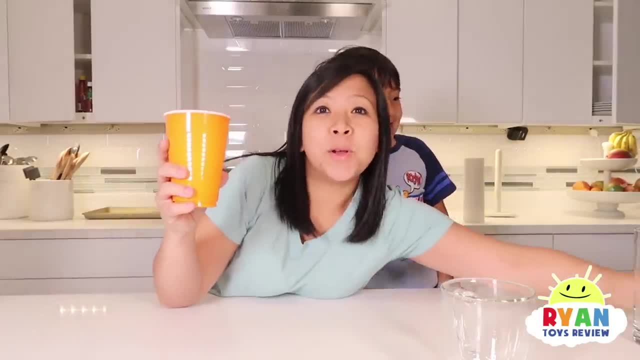 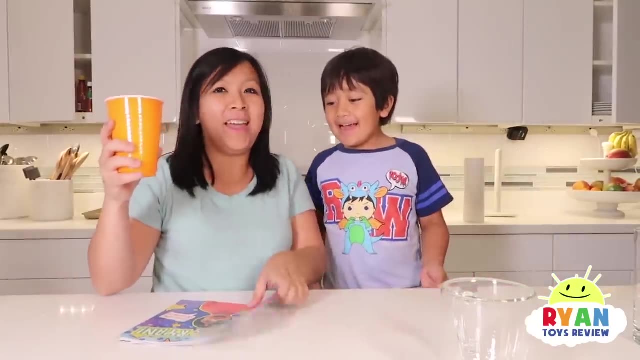 Do you trust me? Okay, so here's what we're going to do. Okay, you guys ready? Oh, no, no, no, Here's what we're going to do. You said you trust me. Okay, I'm going to use Ryan's book here. 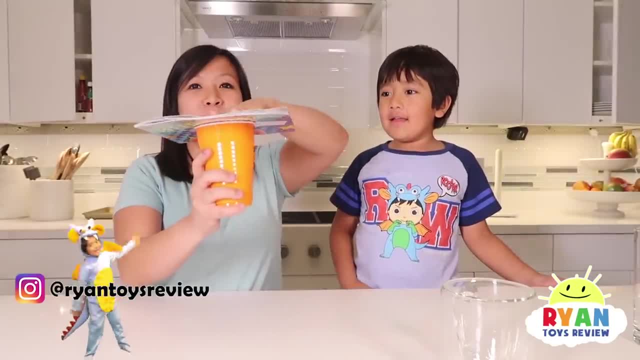 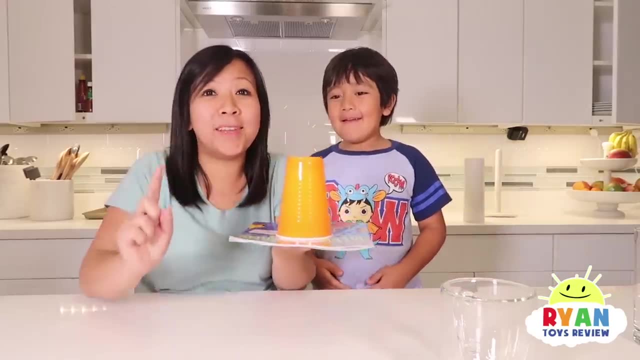 I'm going to cover this. Do you see? Flip it upside down. Oh no, Hold on, I'm not done. I'm going to put it on top of Ryan. Put it on top of Ryan's head. No, no, no. 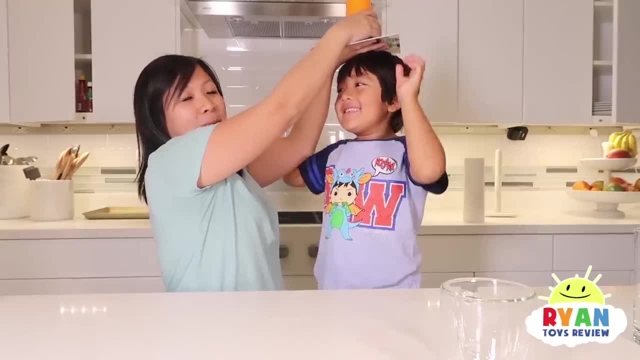 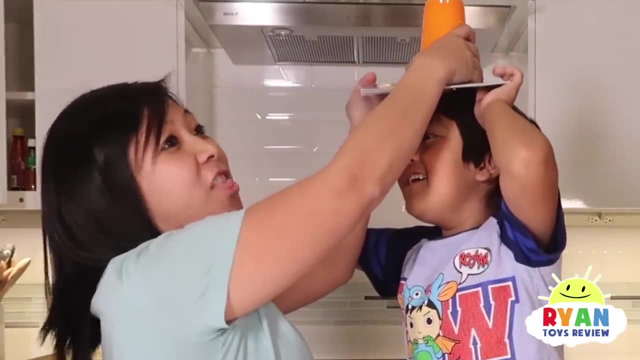 You said you trust me. Okay, alright, you guys see this on top of Ryan's head. Now here's what's going to happen. okay, No, no, no, I'm going to remove the book. No, no. 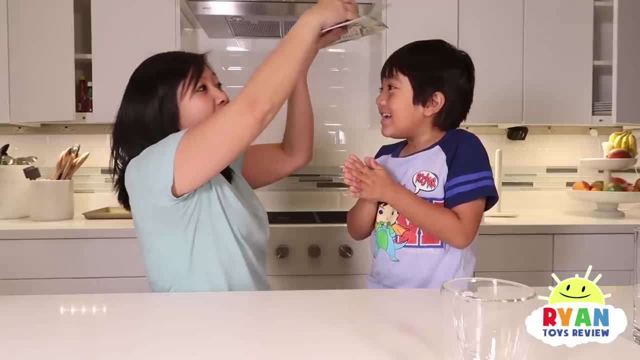 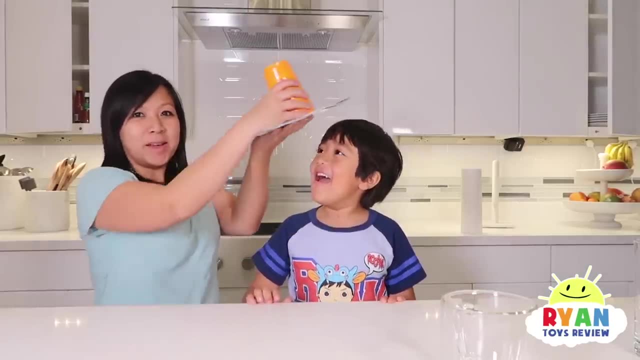 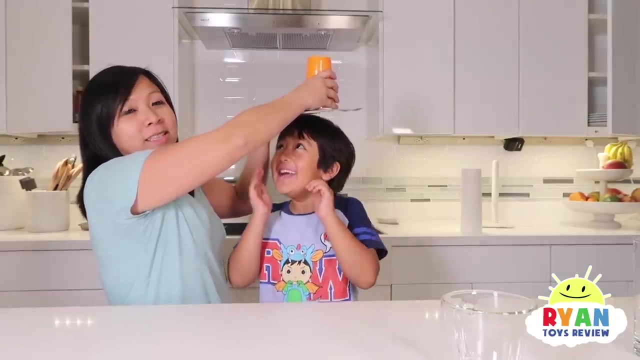 You said you trust me. It's just water. It's just water. How good Do you trust me? Yeah, I'm going to remove, It's just water. right, I'm going to remove the book. I'm so scared. 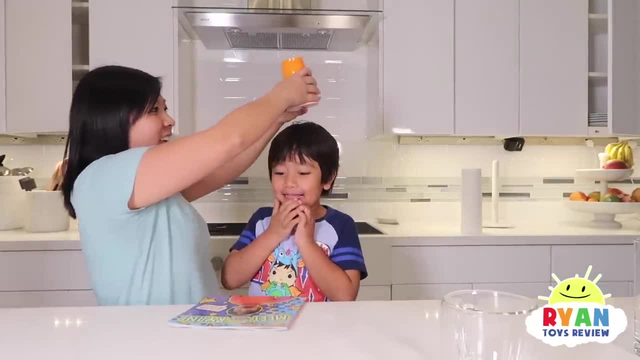 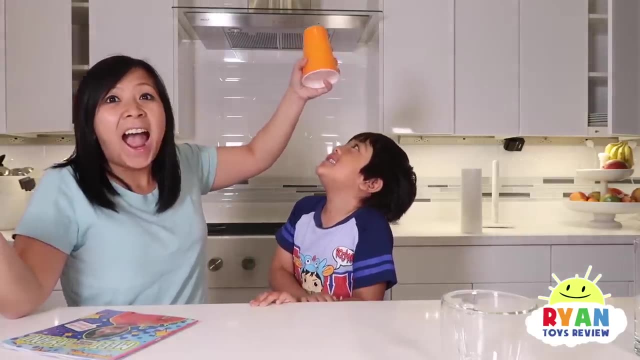 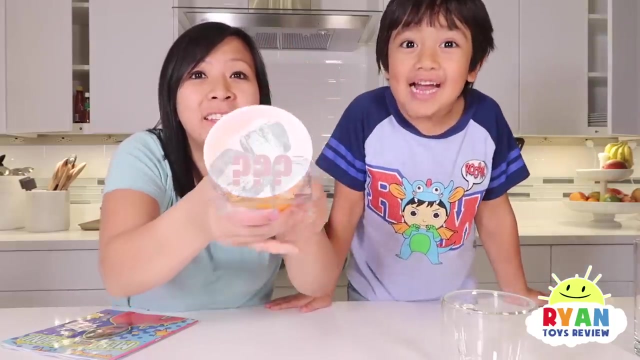 Look, Look, guys, look, See, See what happened. It didn't even fall, It turned to ice. Look what happened. So what's really going on? I don't know if you guys can see it, but it turned to ice. 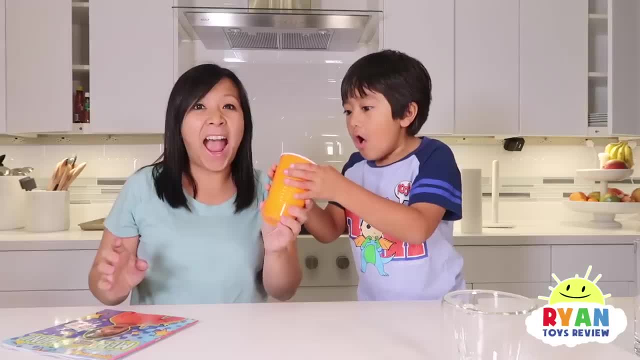 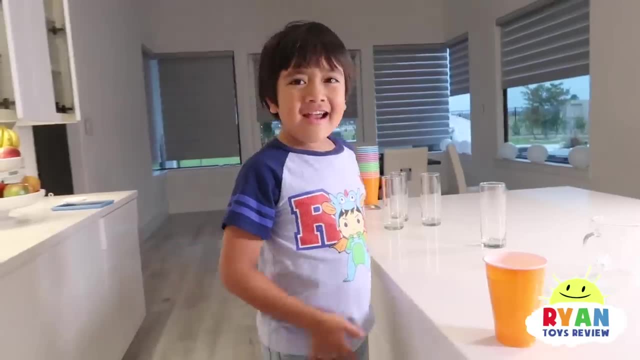 There's something in here. It turned into ice. you think, Yeah, Okay, now we're going to just dump it out. It's a squishy thing. It's something squishy, Alright, so we'll find out. 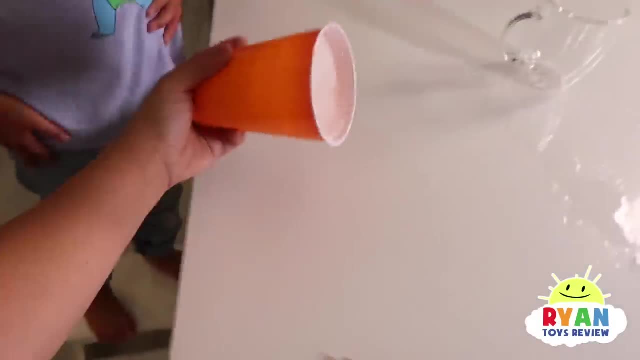 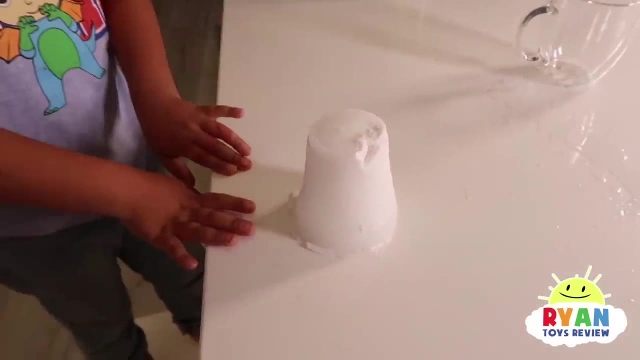 Okay. so if you look here, yeah, there's something. So look what you can do. You ready, You can go like this: Now you can just move it around, so it'll come out A little bit too much Mind blown. 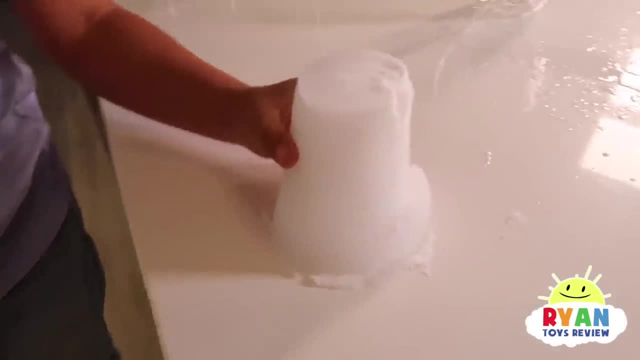 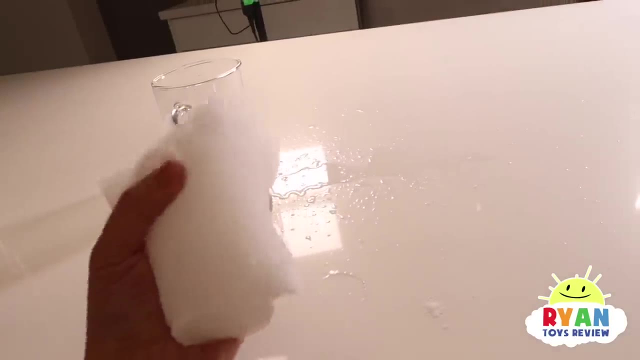 How Do you see that? How did you do that magic trick? So whatever I put inside absorbs the water, Do you see? You can just crush it up, But whatever it is absorbs the water, And that's why, Ryan. 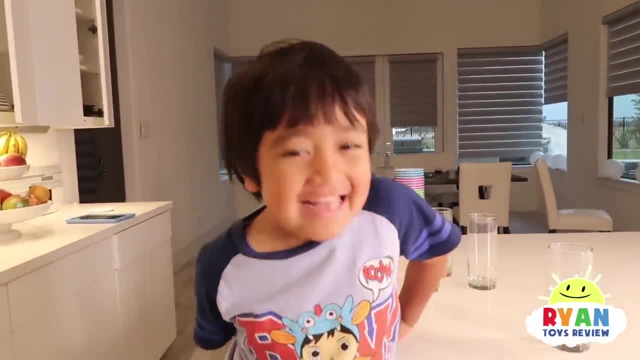 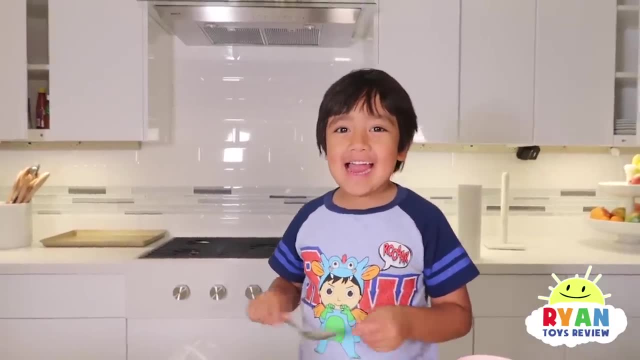 did not get wet. What do you think? What Do you like it? Cool, Yeah, How do you do that? You want to try it on Daddy later? Yeah, Okay, so you ready for the trick? Yeah, So what I used? 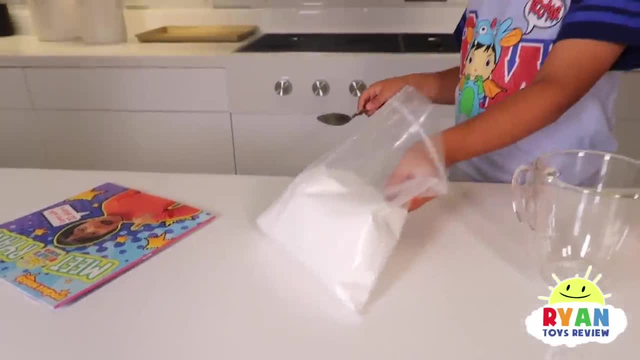 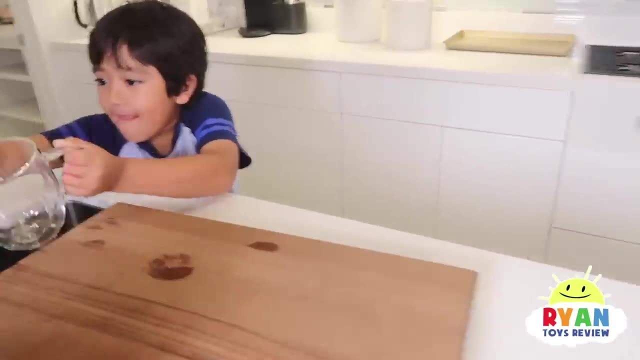 was this magical powder called water gel that I bought online. Okay, if you guys want to get it, I bought it from Steve's Spangler Science website. So first, Ryan's going to need some water, A lot more. The whole container. 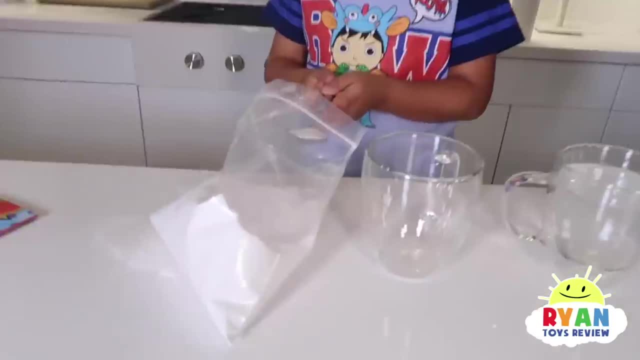 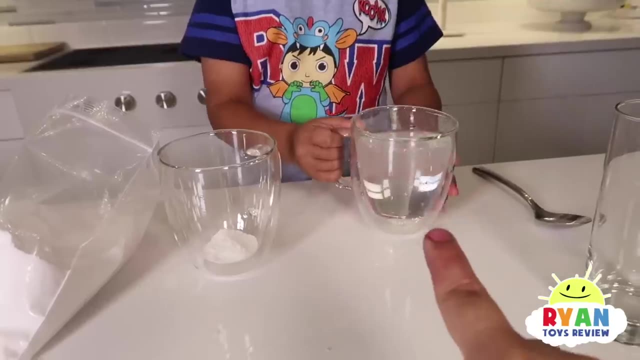 Just fill it up, Ryan. Fill it up. There you go, Take one spoon of that pour it in there. Okay, that's all you need. Now you can use that and pour it in there and see what happens. Are you ready? 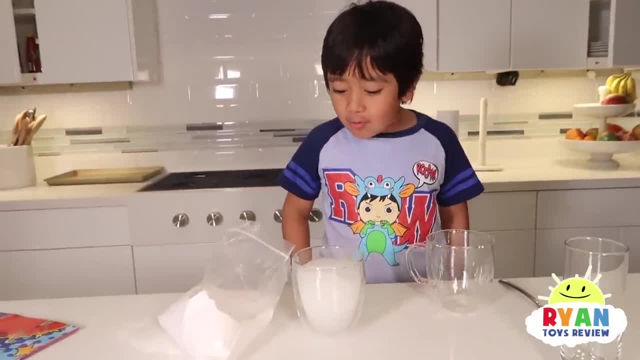 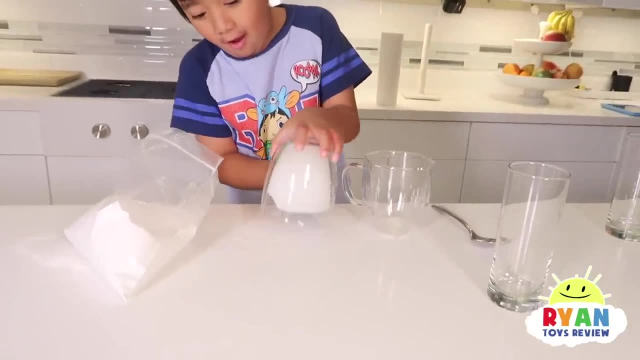 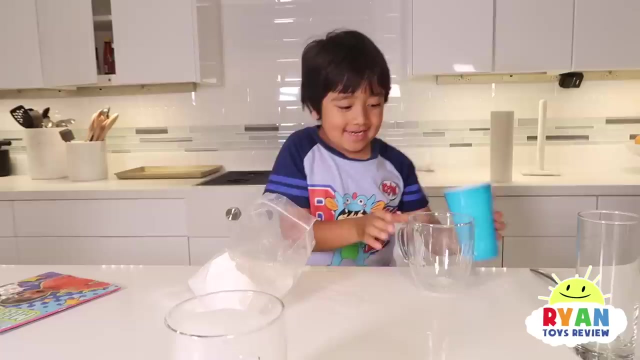 What happened? It just absorbed all the water, Exactly. Can I try to turn it over? You see It doesn't come out. What Mind blown. That is so cool. This is so cool It is. It's one of my favorite science experiments. 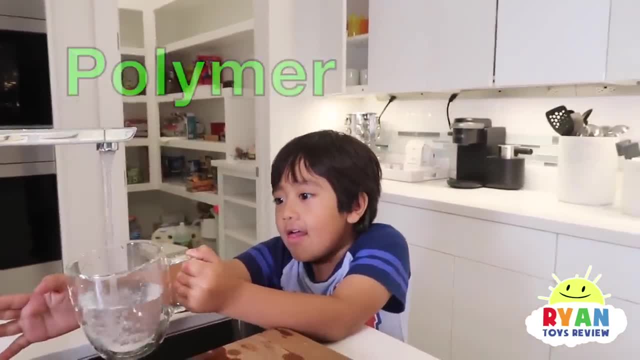 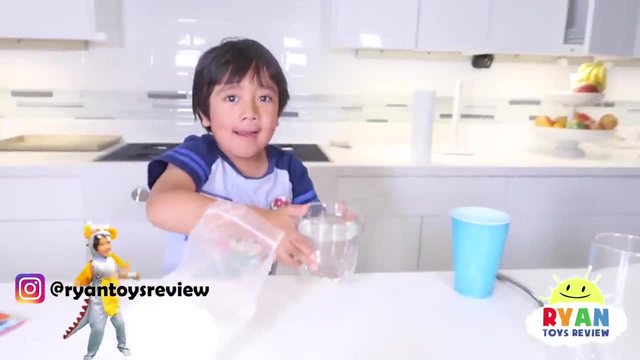 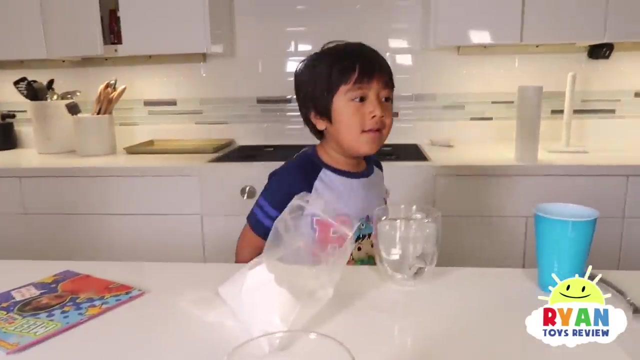 So these are called polymers and they're really really good at absorbing water. Wow, And do you know where you can find these? Where Do you want to guess A product that you see where this chemical could be very, very useful? Do you know? 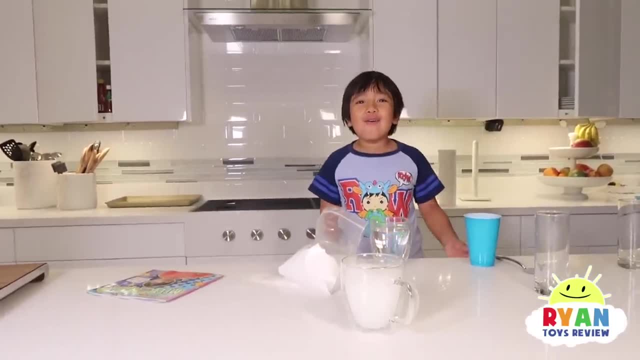 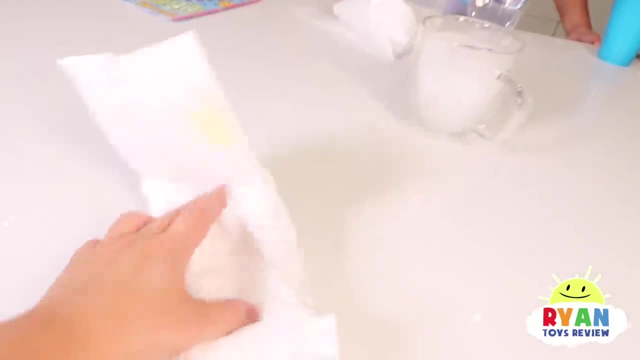 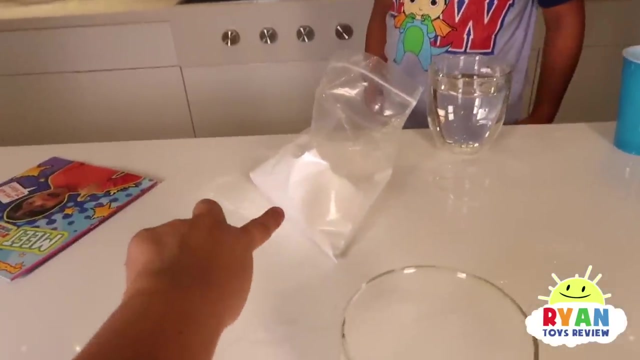 Alright, you want me to tell you That is actually also in diapers. That's what they use in diapers. So, like, if you cut this open, what you see inside the diaper is actually these powder or something similar to this powder. 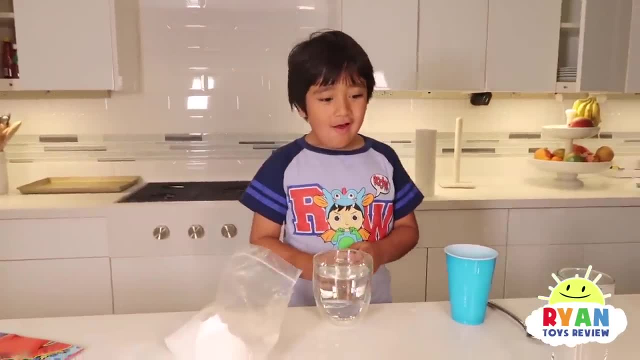 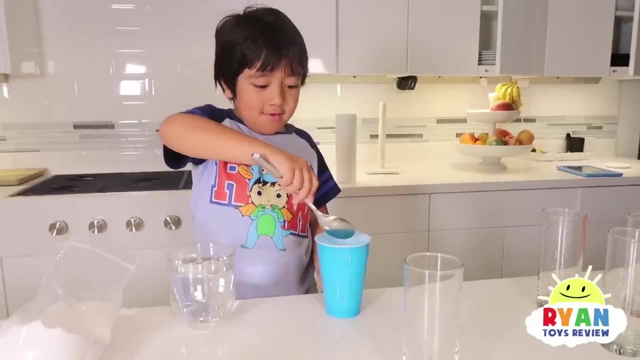 That's why it's good, right. That's why you can- you know you can- use the diaper and it absorbs a lot of water in here. What You know, what would be fun? Let's try to make a color version. 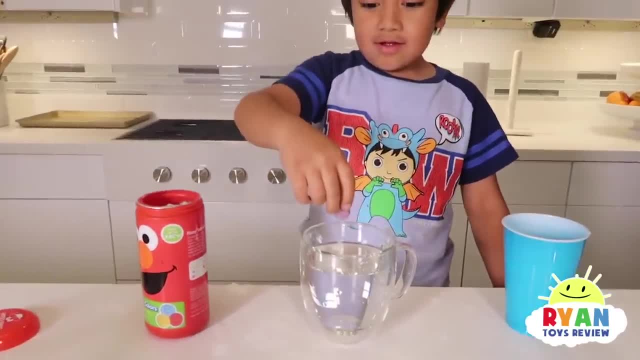 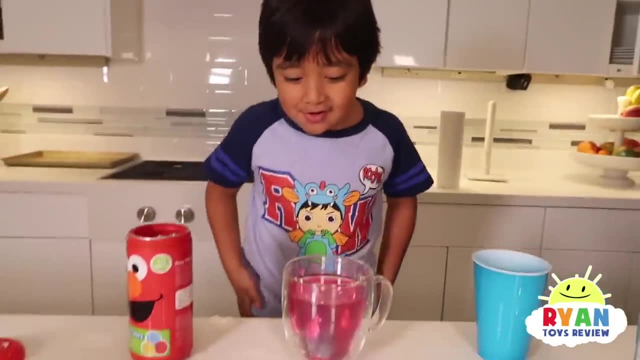 Let's do it. We're going to use Elmo's scissors here to see if it works. Alright, we're going to change the color to red. It's actually purple, but it looks pinkish. Yeah, Abracadabra, Abracadabra. 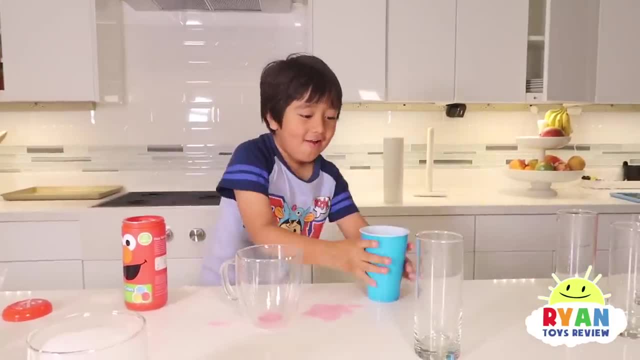 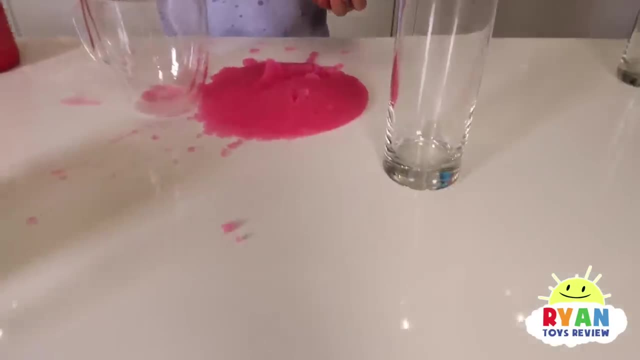 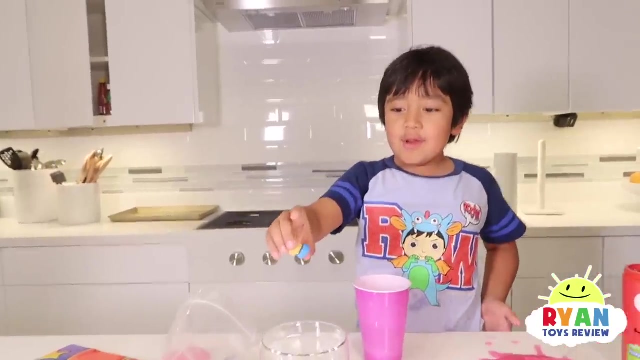 Abracadabra, Make my water disappear. Let's see if we can take it out Ryan. So Ryan splatted, so it broke. I guess we're going to try again. I think it's going to make green, or it might just make it. 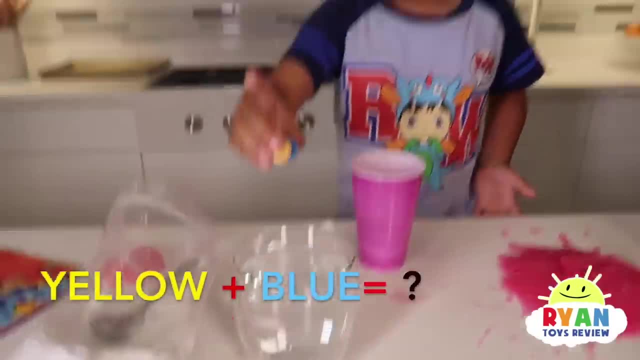 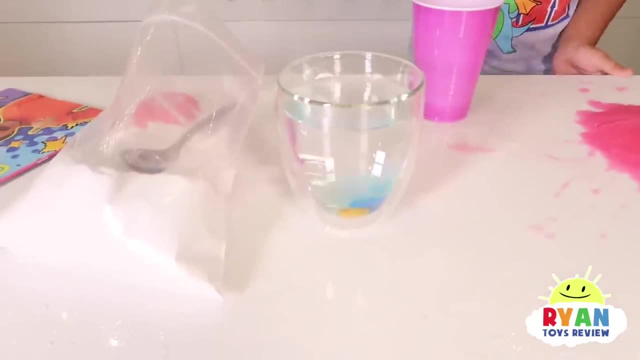 Yellow and blue. You guys know what color it's going to make. It's going to make green, or which color do you think is going to go over the other color? I think if blue is going to go over yellow, or they make green. 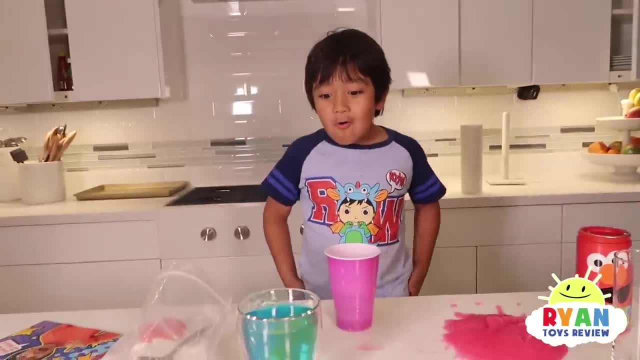 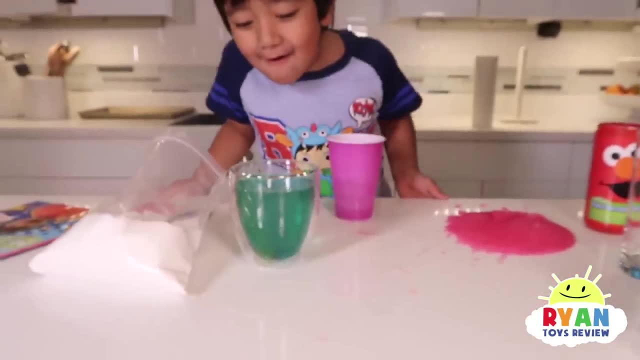 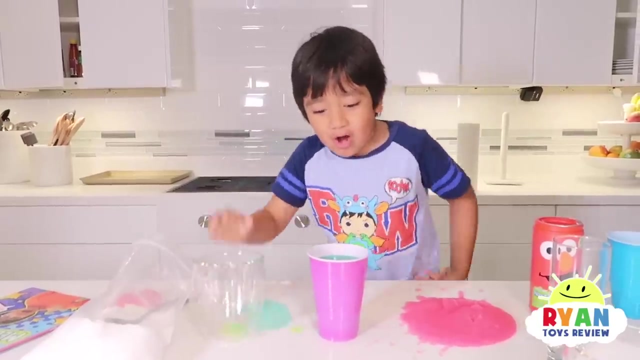 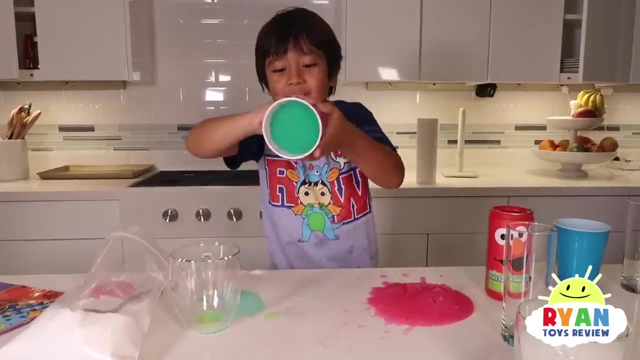 Let's see. Wait, they're making green. That's so cool, huh Whoa, It's so green. now, Yeah, One, Two, One, Abracadabra, Abracadabra, Make my water disappear. Oh Ryan, Oh scary. 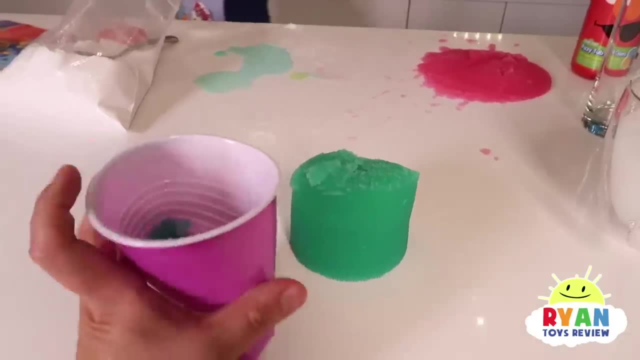 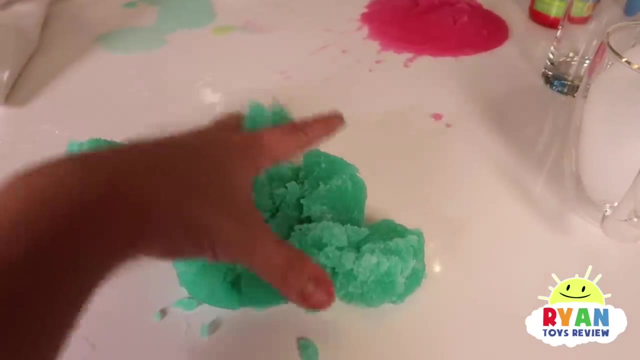 Whoa, it broke inside. We must have squeezed it. Oh yeah, Okay, it's still inside here. You guys see it. It almost feels like a like a slushy, doesn't it Feels like a slushy? 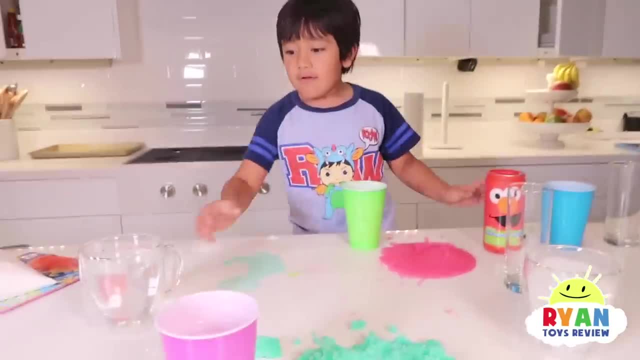 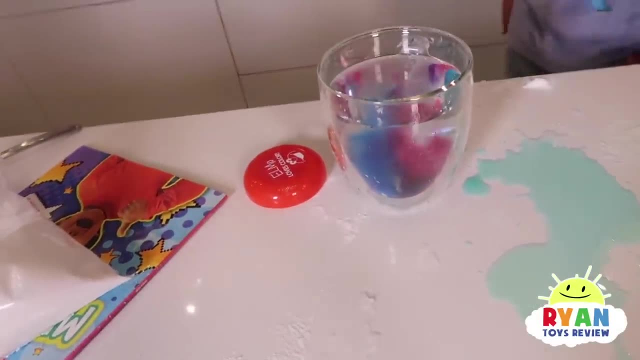 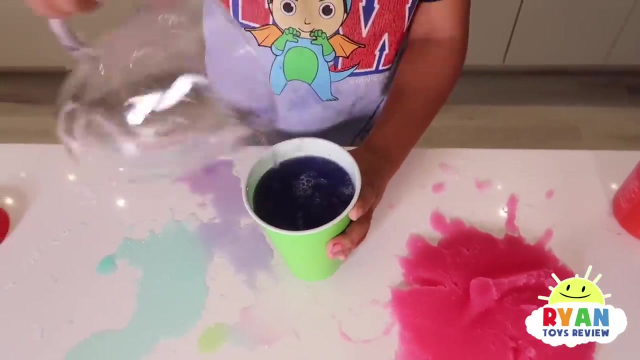 Slushy. Alright. third time's a charm. We're going to get this right. Third time's a charm. Three, two, one. Four in Three, two, one, Abracadabra, Abracadabra, Alright. so there it is. I'm going to see if I can. 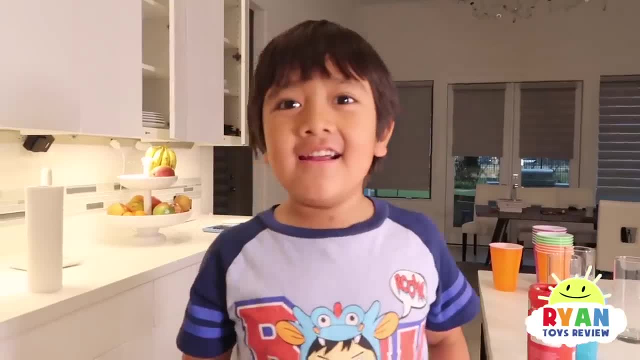 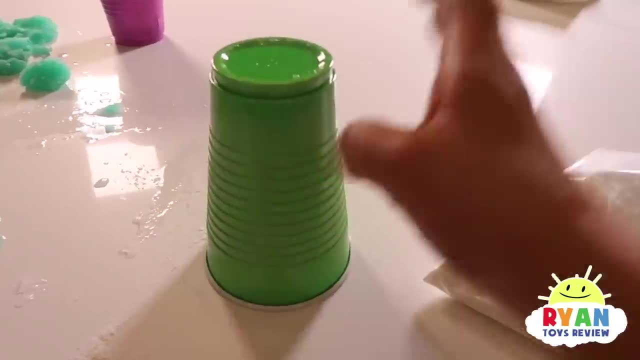 pour it out. Look at our mess, Super messy, huh, But it's okay, It's fun, It's really good to learn, Okay. So super water absorbent. Okay, just go like that, Squeeze it a little bit. 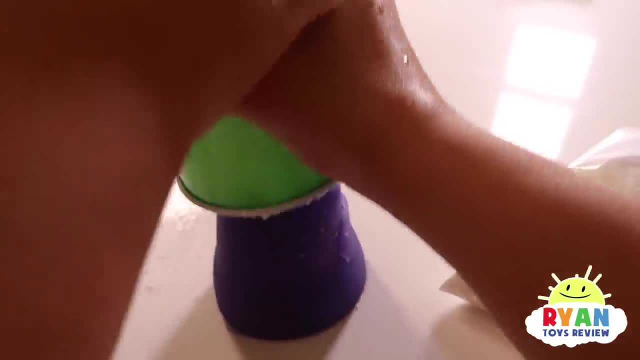 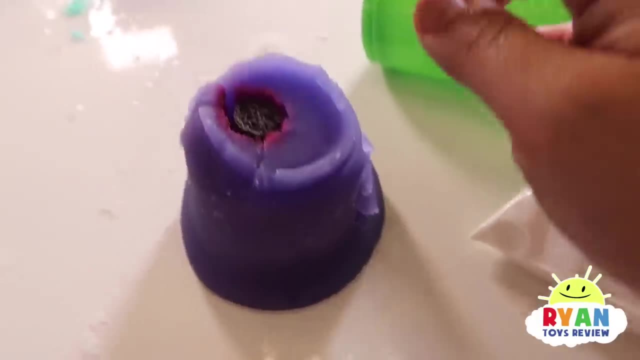 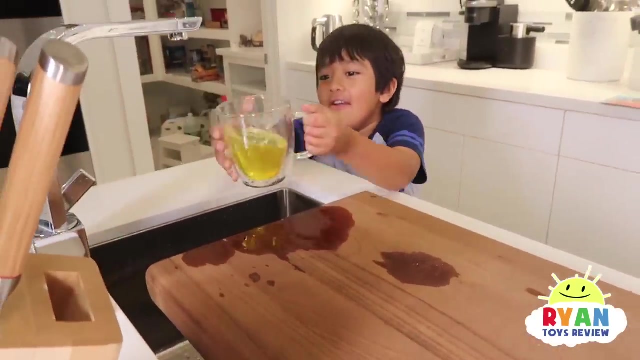 There you go. Alright, let's see if we can just shake it Almost. So close, So close. You see it right there. Yeah, so close. The little fizzer thing that's on here, The little bath thing, Magic yellow water. 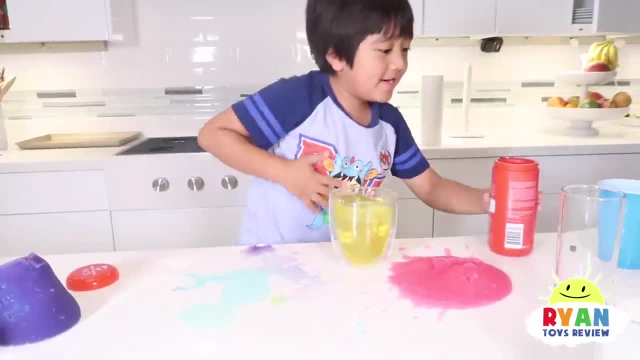 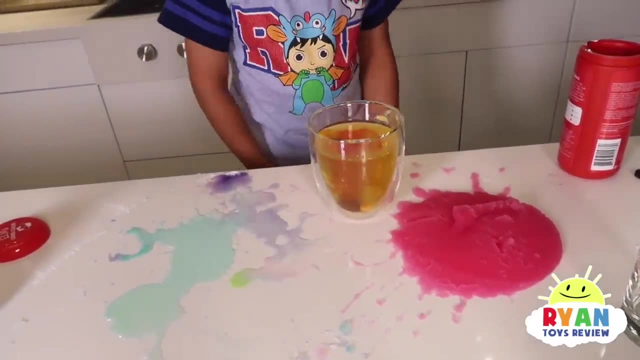 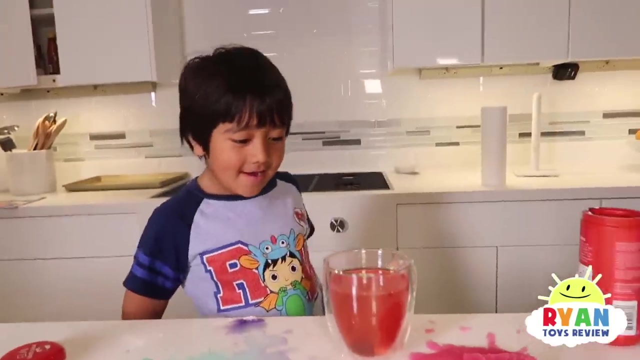 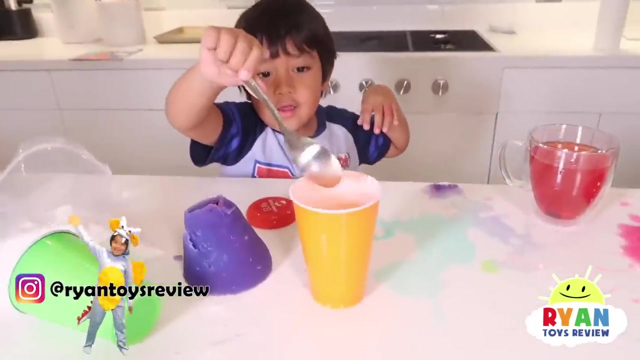 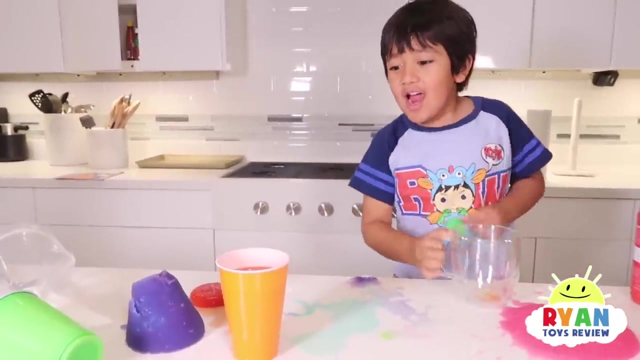 Magic yellow, I didn't do anything. Yellow and purple, maybe, Or red, Yellow and red Orange, You should know right, Yeah, Mixin' mixin', mixin' mixin' Magical gel. So cool, Abracadabra. I like how the bubbles. 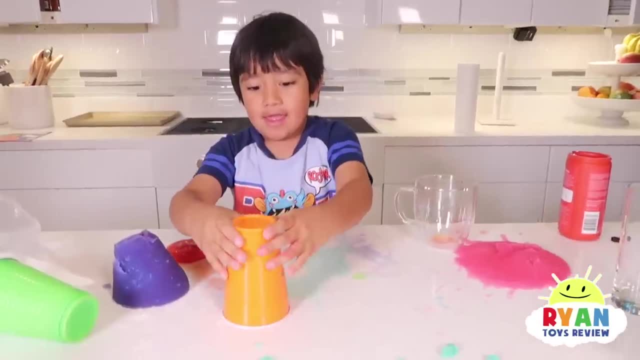 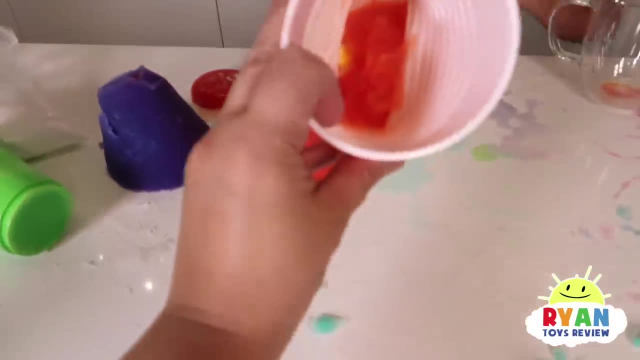 are still there. Let me see. Well, they all pop. Here we go, Don't worry, Come on. It broke, But it's okay, It was so much fun. Alright, guys, We're going to clean all this up and we're going to get ready. 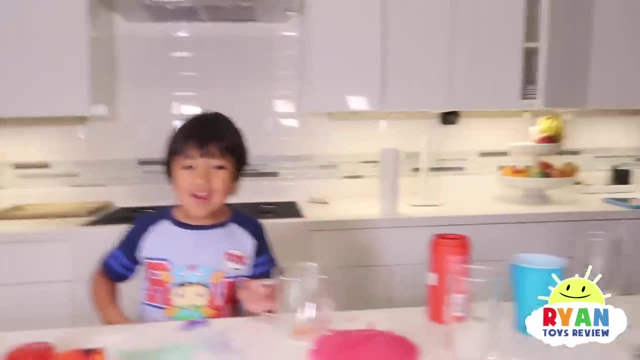 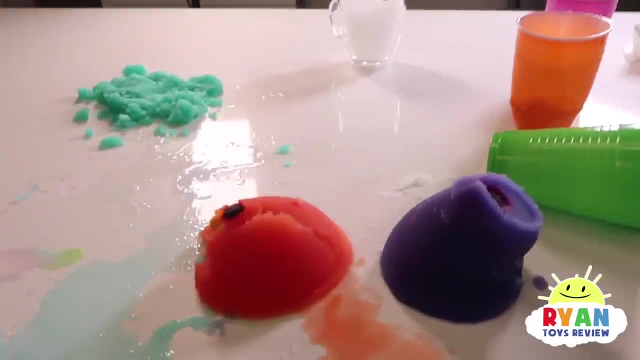 because Daddy's about to come home. We're going to prank Daddy, Make it look like we're spilling water on top of his head. Are you ready? Yeah, Okay, so I'm having to clean up, but I just want to show you guys. 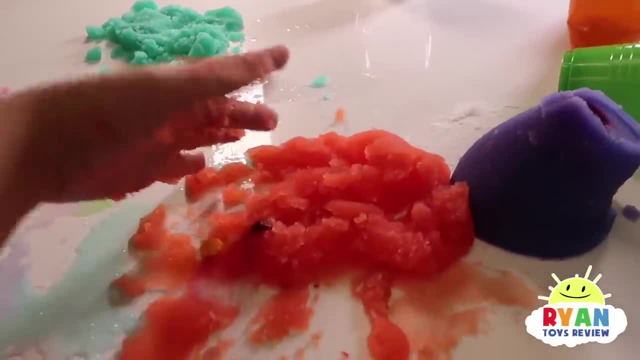 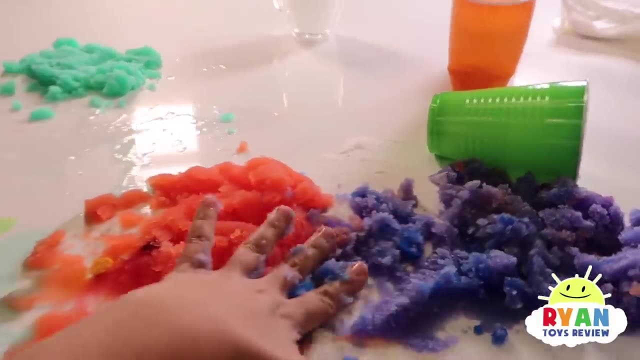 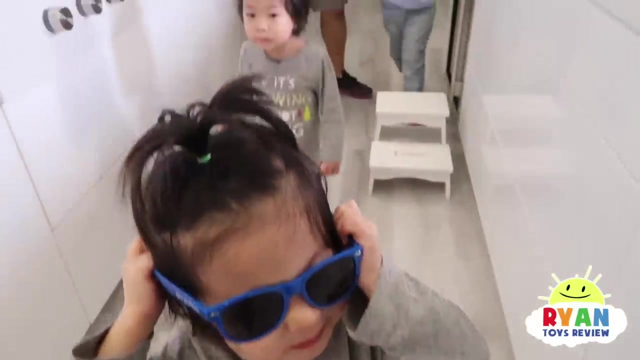 it's so fun just to smush it. So look at this. Can you believe these are the things that's in diaper Absorbing the water? That is so cool. Alright, cleaning up time and then pranking Daddy Hi Glasses. Yeah, so Emma. 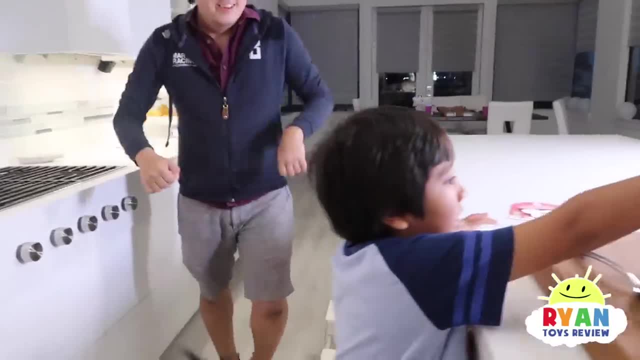 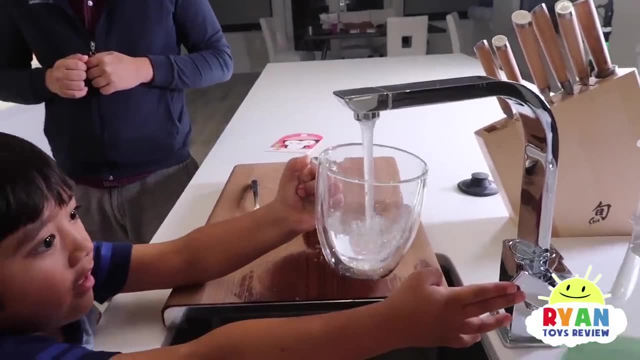 and Kate and we're on Daddy's home. Hey guys, Alright, Ryan's going to show you something. Okay, Oh, is it the magic trick? Yes, Ryan's going to just put water in here, so you know. you know that it's just regular water from the sink. 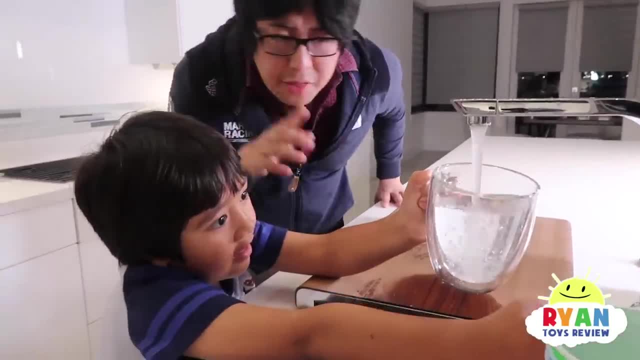 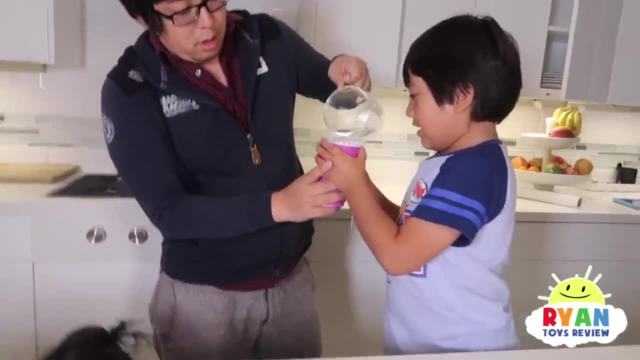 Okay, You can fill it up. Fill it up from to the top. Yeah, I don't see any tricks or anything. Okay, We're going to put water into the cup there, The whole thing. Okay, Alright, don't let. 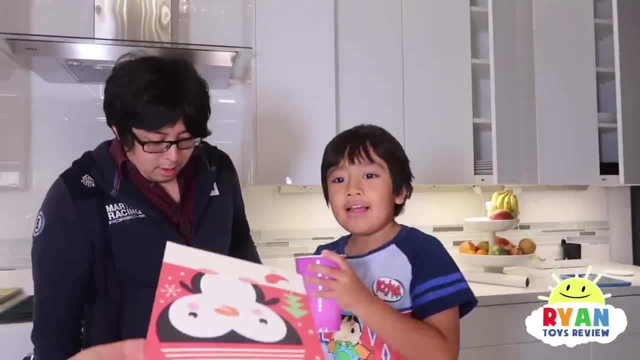 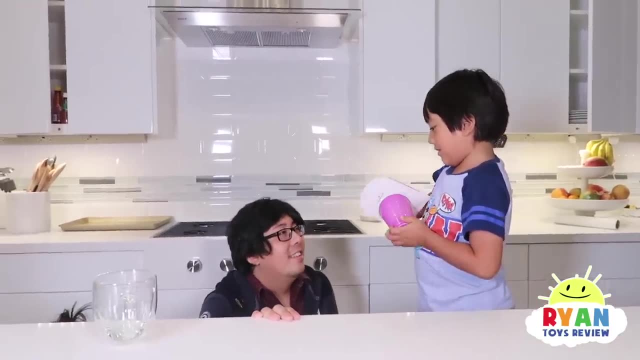 Daddy. look, Ryan. Alright, Ryan's going to cover it up with this, Okay. So, Daddy, you're a little tall, so can you bend down. Do you trust Ryan? Wow, What are you doing? Do you trust Ryan? 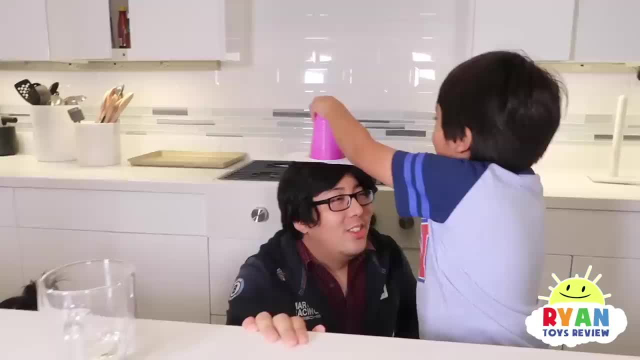 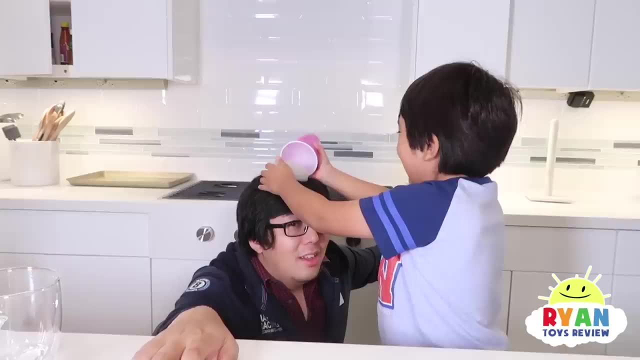 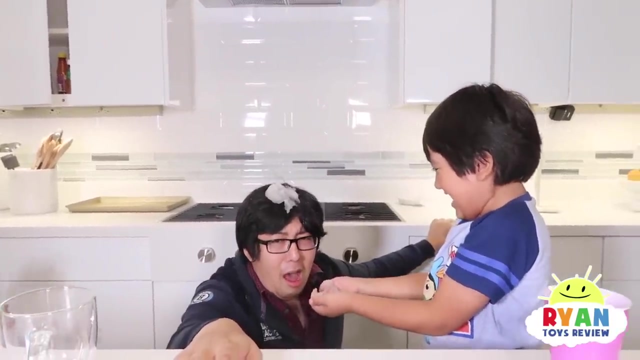 No, I don't trust Ryan. They're dripping already. Do you trust Ryan? No, I'm going to put my phone. Three, two, one, What What? Ryan, Ryan, Ryan, Ryan, Okay, so Ryan. 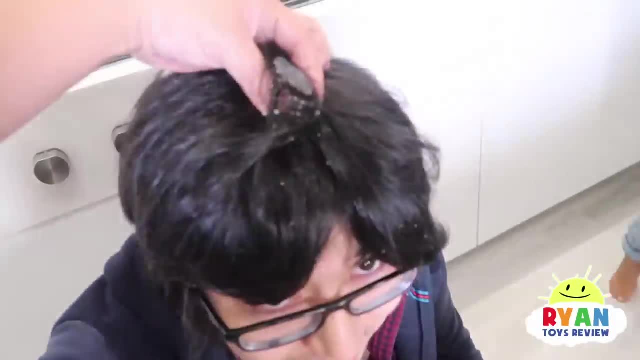 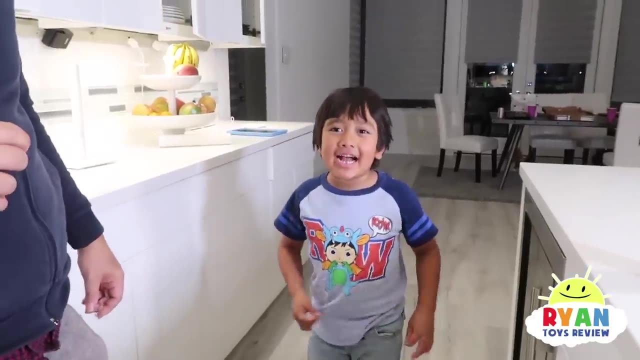 So now Daddy's really dirty with the stuff, so sorry about that. It was close, though, Mommy. Thank you so much for watching guys. Bye, Bye, We're going to practice a little bit more before we try another trick. 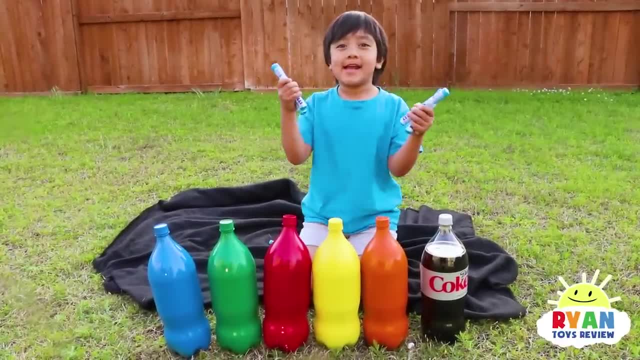 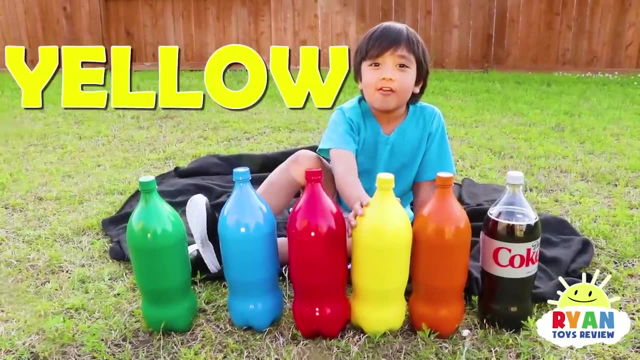 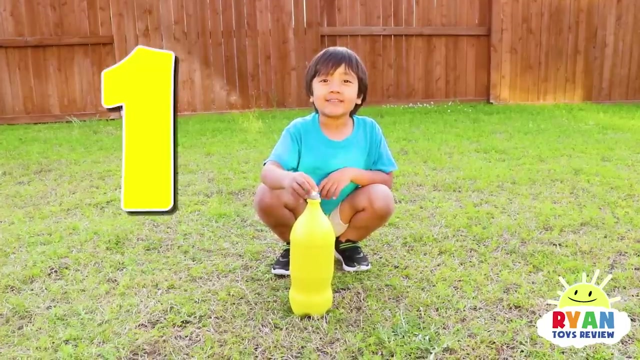 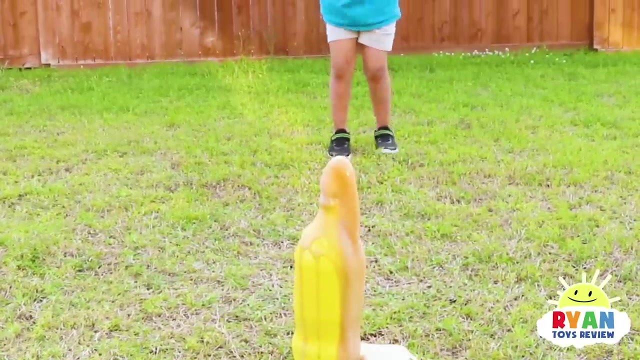 Today we're going to do the Mentos and Diet Coke experiment And learn colors. We have green, we have blue, we have red, we have yellow, we have orange and regular One Mentos and yellow So big. 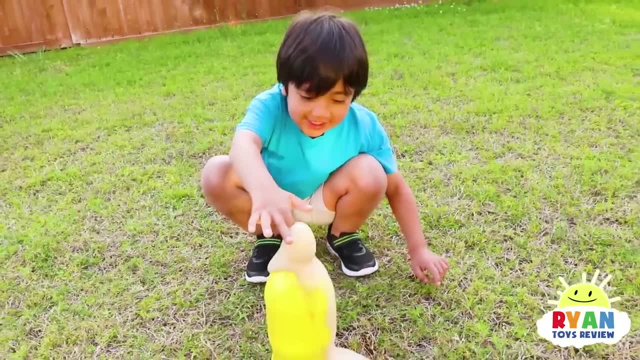 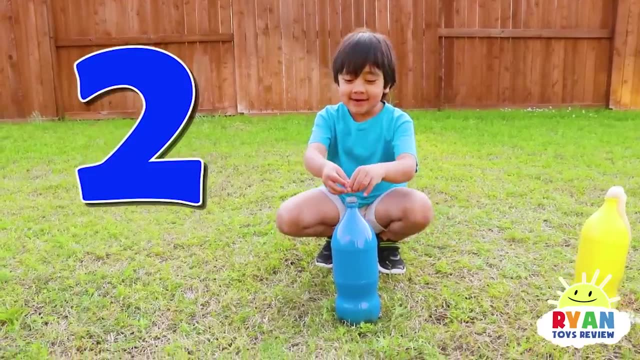 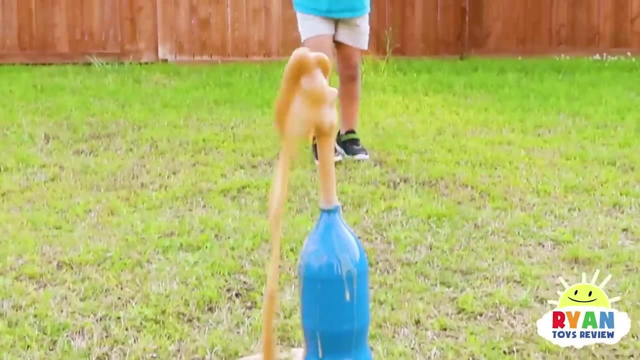 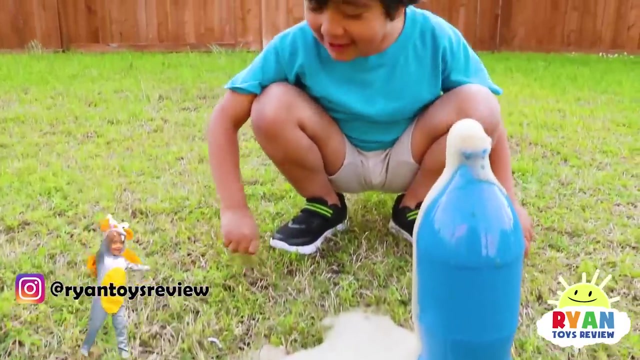 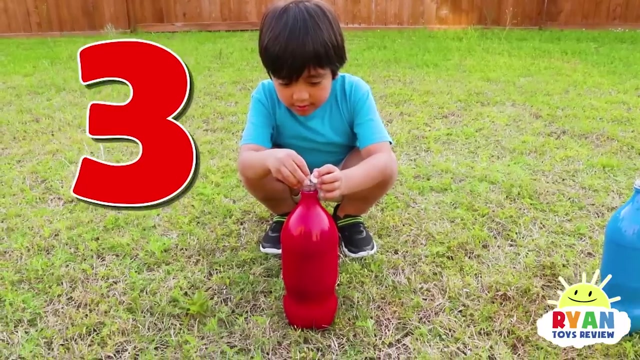 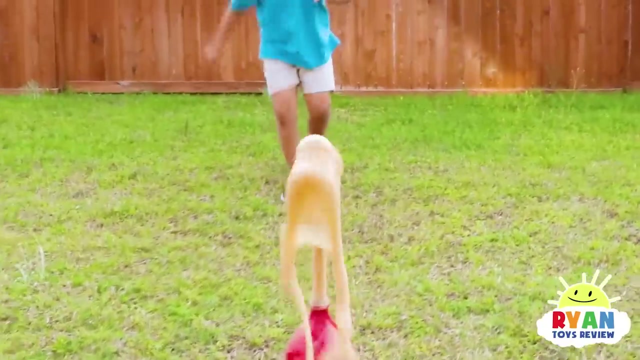 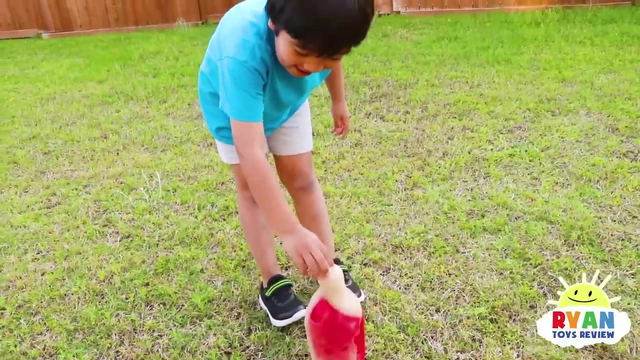 It's disappearing, Still going, It's going faster. Two Mentos and blue. Two Mentos and blue. Whoa, It's disappearing. Three Mentos and red. Oh, Oh, it's so big, Yeah, Yeah. Four Mentos and orange. 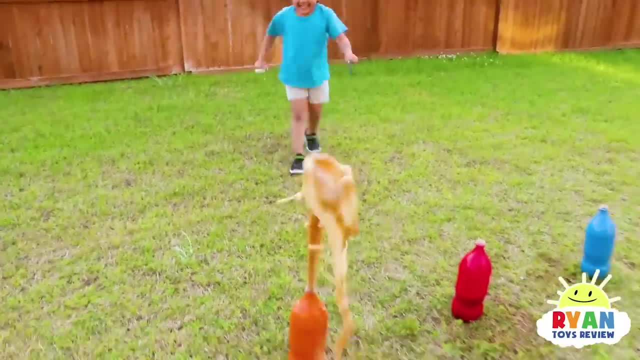 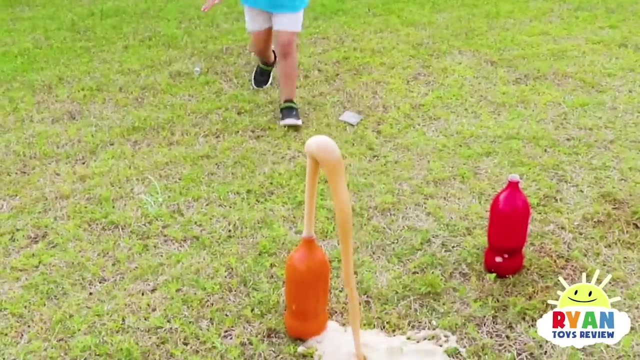 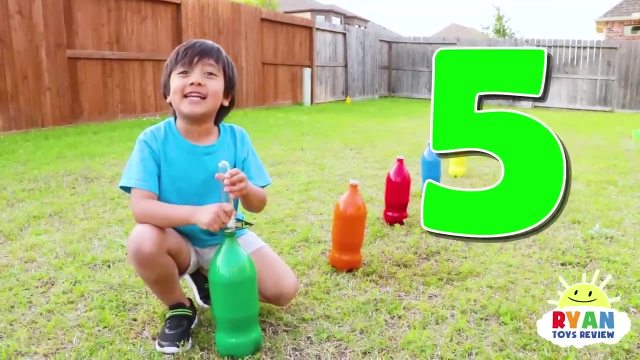 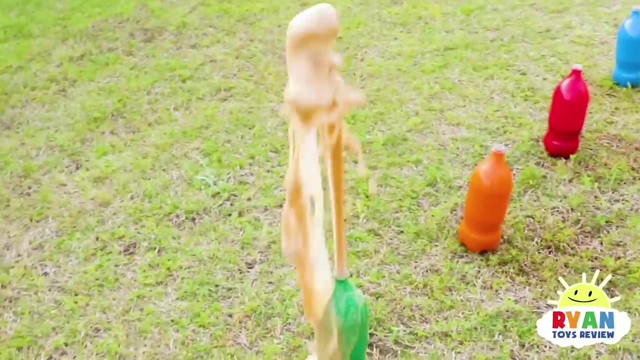 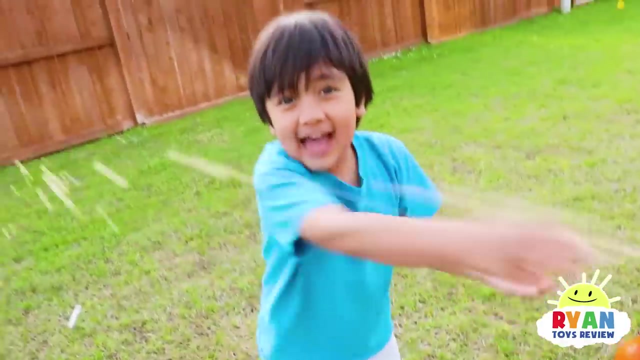 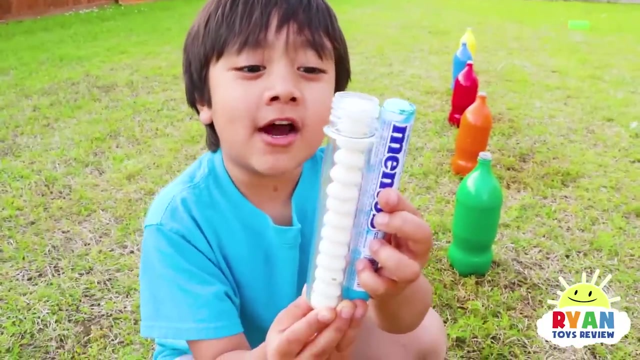 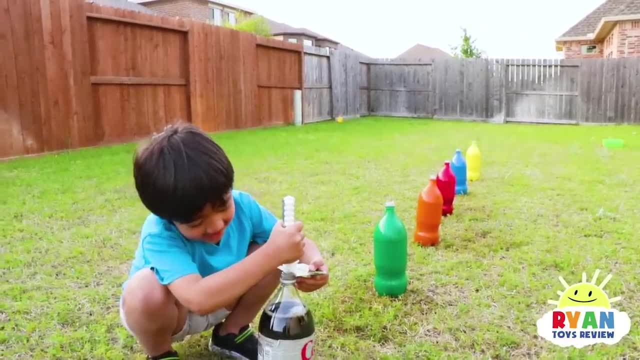 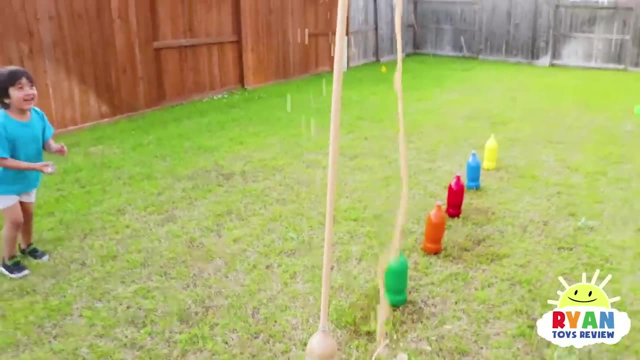 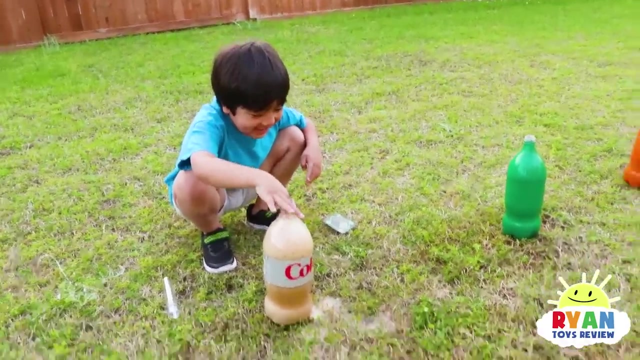 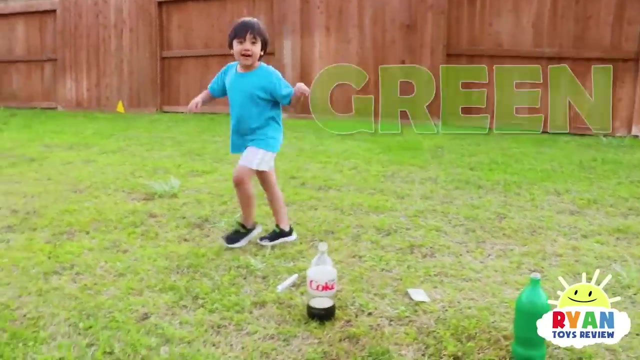 and the regular fat Coke. Are you ready? Boom, boom, boom, Whoa, Whoa, So giant. One more time We have yellow, blue, red, orange, green and regular. Yeah, Yeah, Yeah, Blah, Blah. 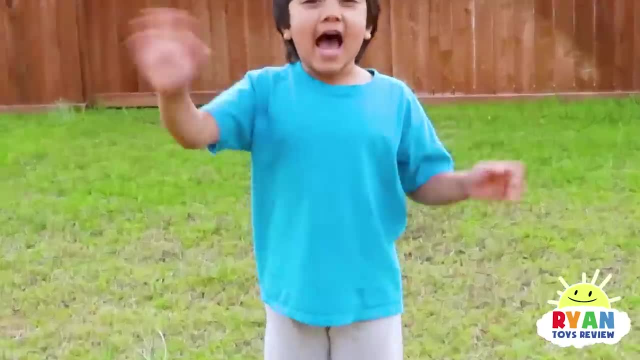 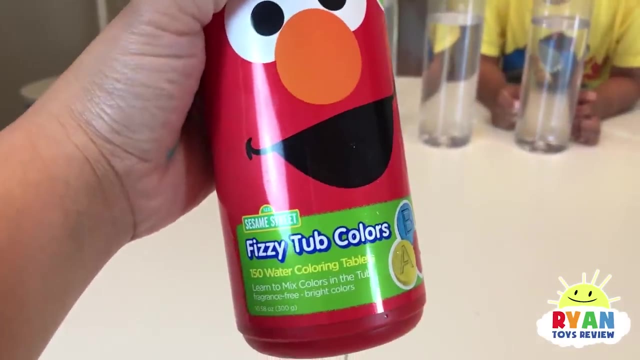 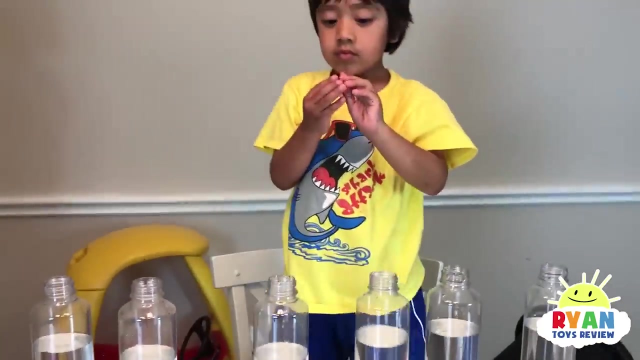 Thank you for watching my Diet Coke and Mentos experiment. Bye Today. let's learn colors with Ryan. Yeah, So we have these awesome Sesame Street Elmo Fuzz Ball colors And they're ABC. Let's try Yellow, Yellow. 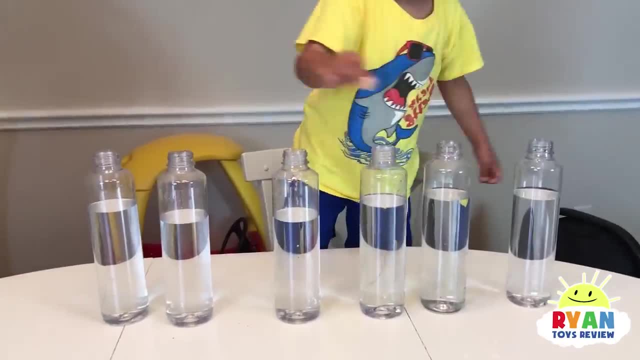 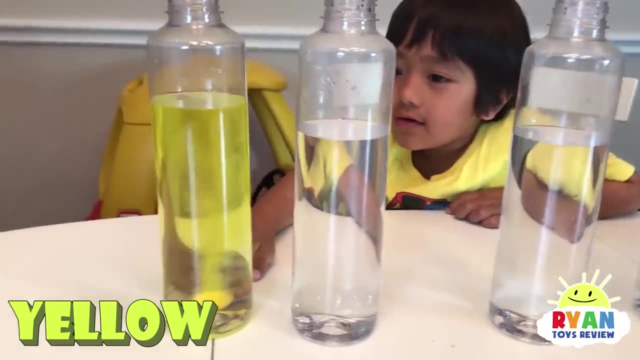 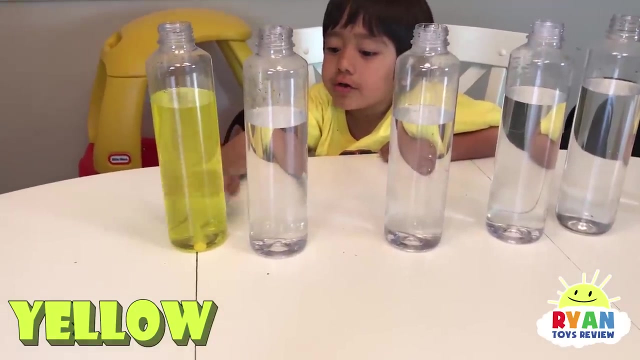 Let's try. And it's V. Whoa, It's yellow. That's right, I can see it in there. It's yellow. Oh, How come it's not moving? How does the water take the color from that? I don't know. 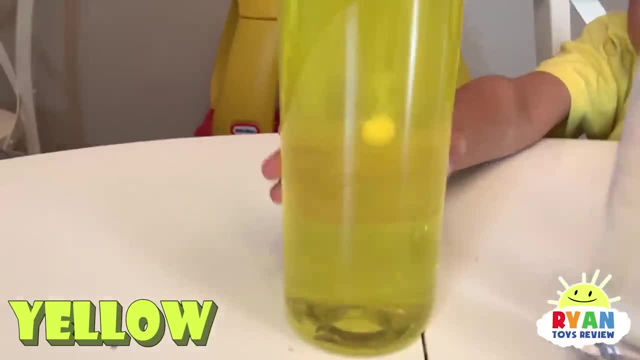 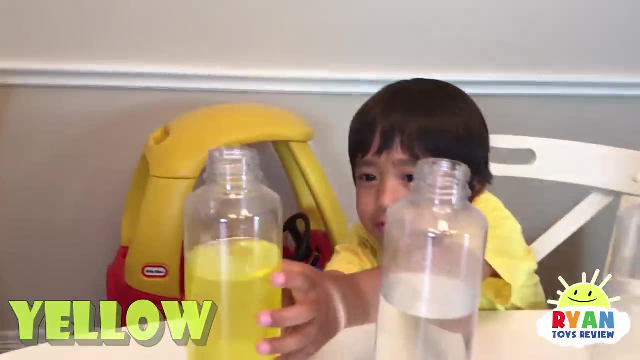 What It's gone. It disappeared, Disappeared. Oh, it got smaller. Oh, he's rising. Oh yeah, it's right. Look it's right here. Alright, here's the next color. What color is that one? 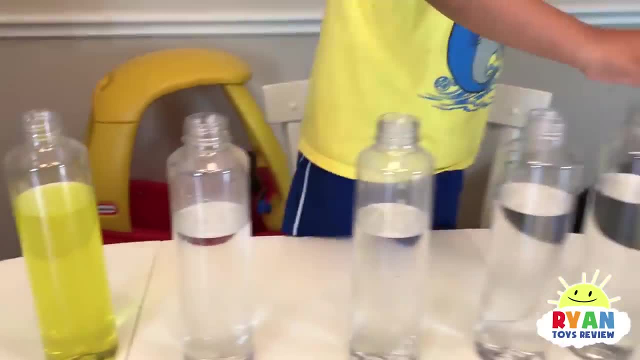 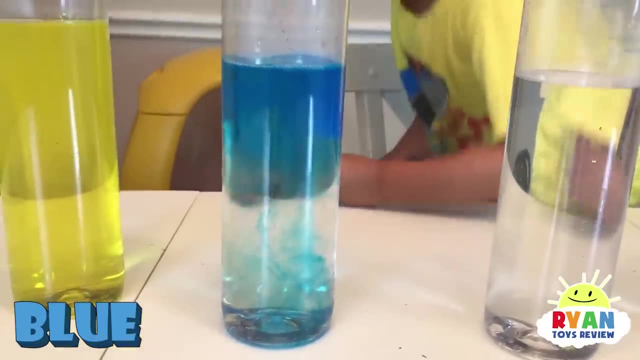 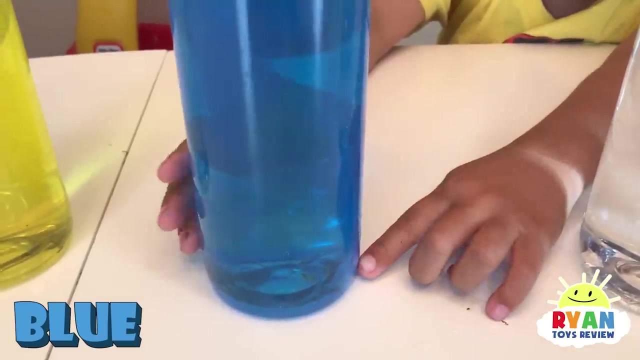 Blue and B Blue, B Do-do-do-do-do-do-do-do-do-do-do-do-do- There it is Blue. Oh, I can see it blasting down there. Yeah, Do you know why it's not gonna fly up? Why? 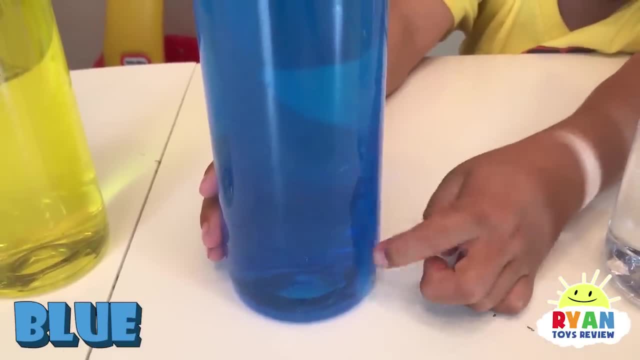 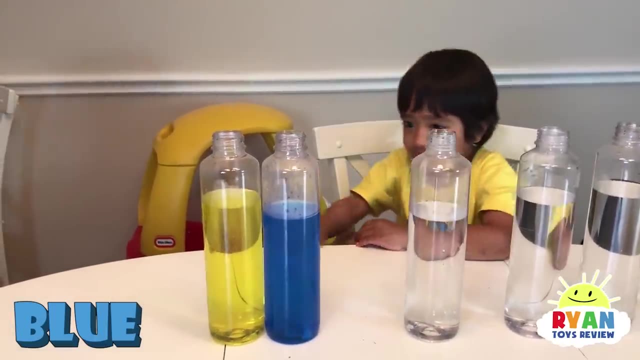 Because all the colors are coming out, So it's kind of like blue fire, Oh nice. So that's why. Oh wait, Look, The yellow's higher than the blue. Okay, Ryan, This one looks like purple, but it's gonna come out red. 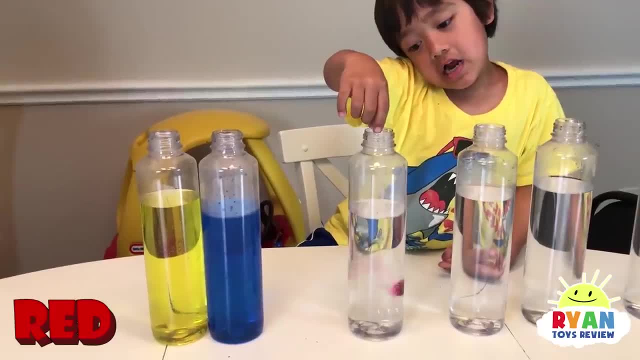 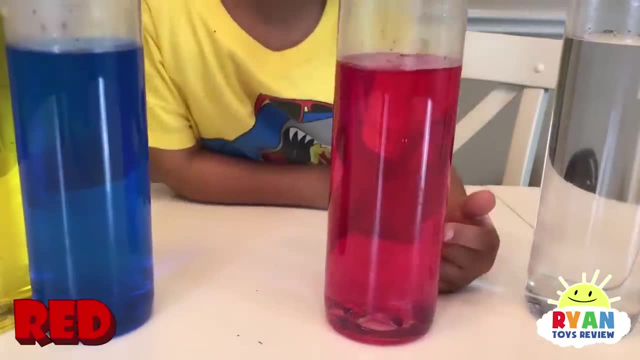 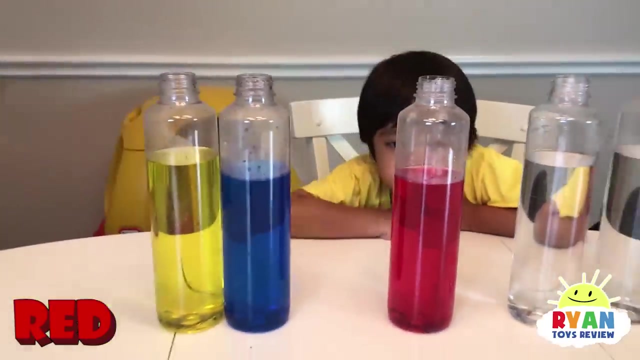 What? Yeah, Okay, go ahead. Oh, it's blasting pink. Yeah, this is red, Acid Red. It looks like pink, That's true, It's like in one of the pinker colors. Okay, so, in order to make different colors, 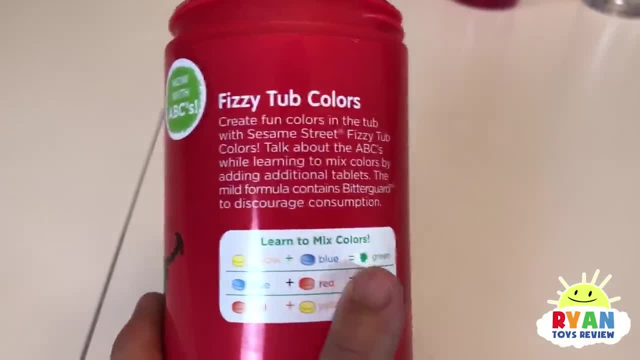 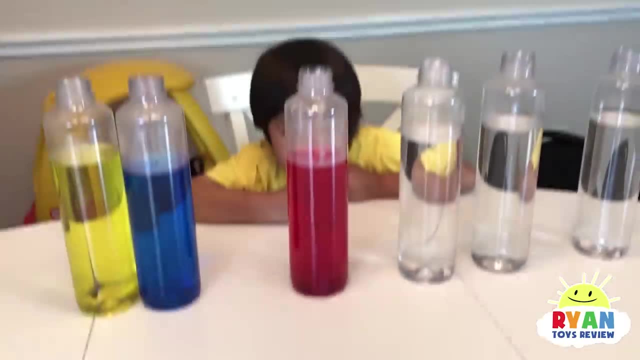 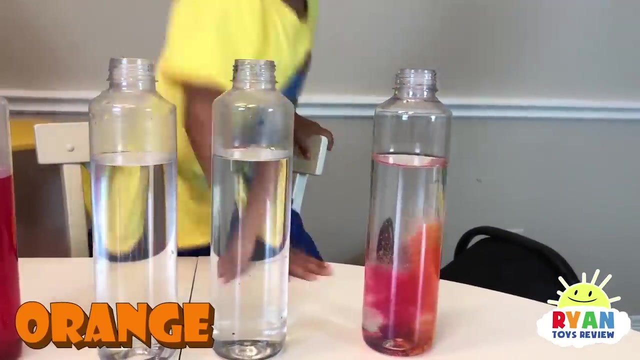 you have to combine them. So yellow plus blue equals green, Blue plus red equals purple. Red plus yellow equals orange. So what color do you want to do next? Red plus yellow, So orange, Red and yellow Blast. Oh, I can see orange. 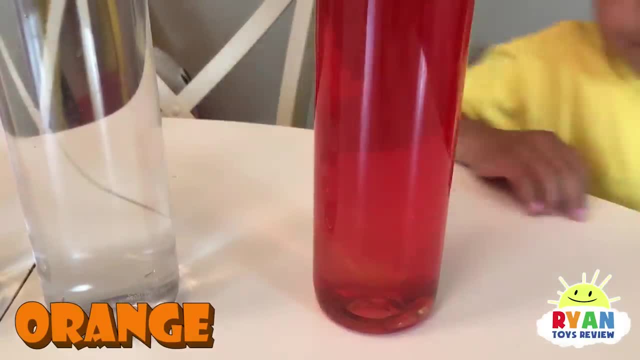 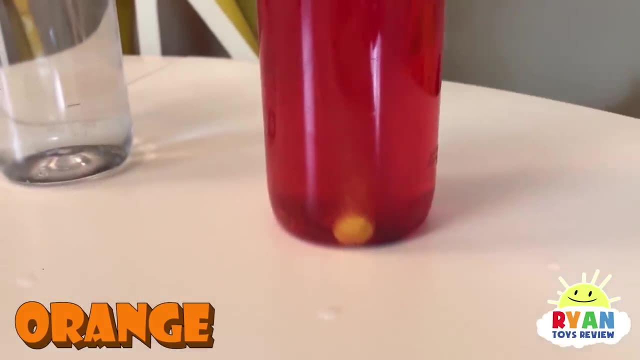 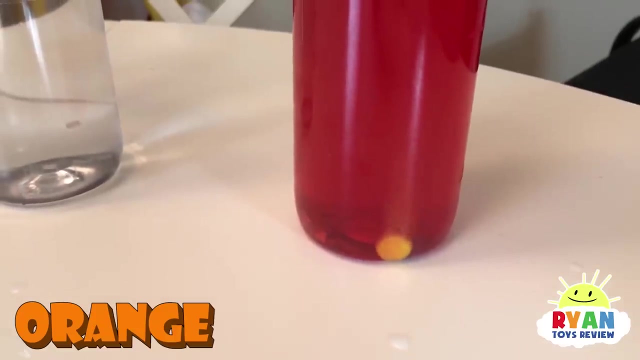 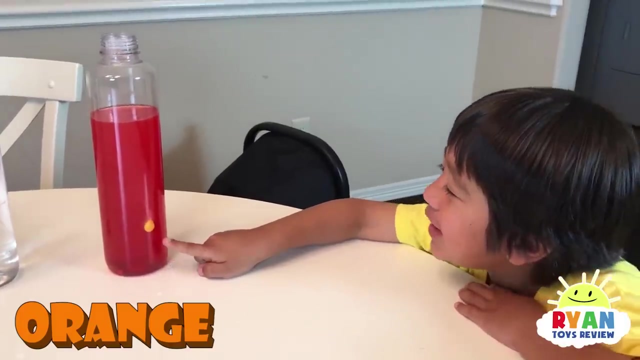 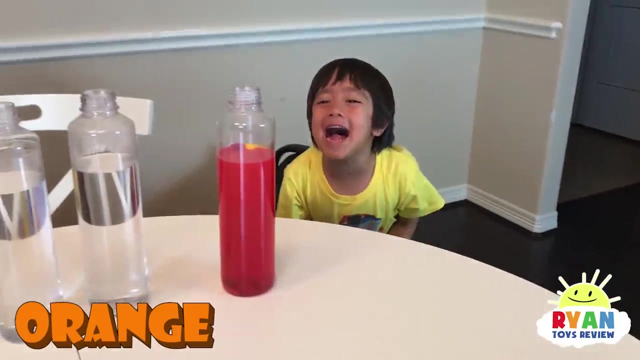 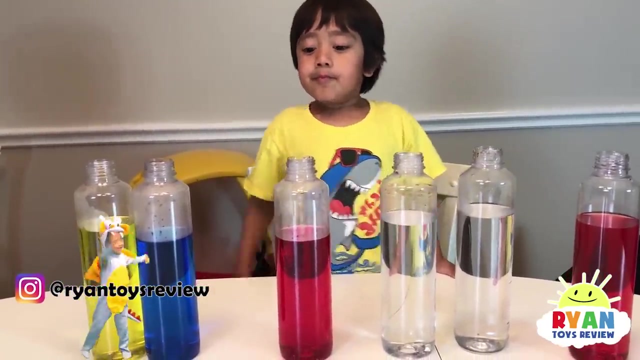 Well, orange, I can see both of them right here. Sure Which one's gonna blow it out first? It's trying to blast down there like yellow fire. Now I want to make purple. How do you make purple? Blue and red? 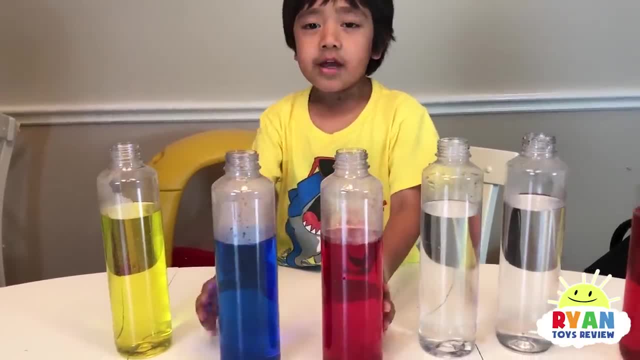 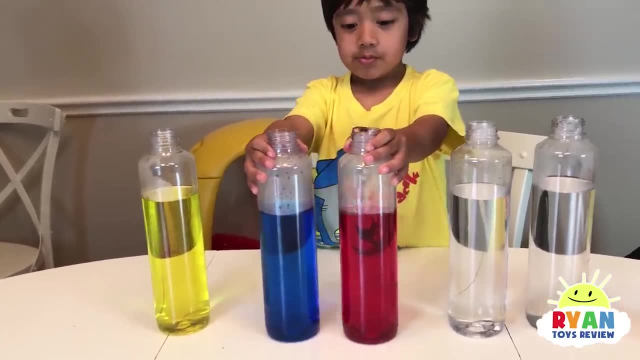 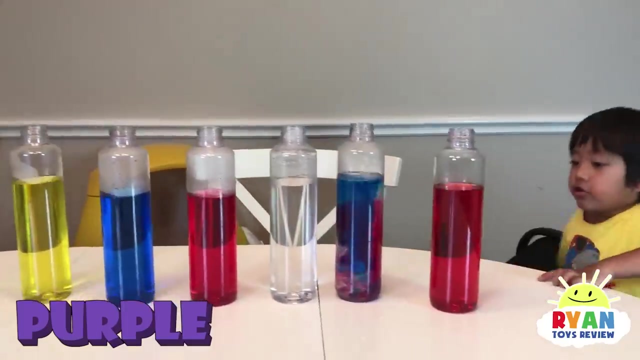 Blue and red. That's right. If we get a big bucket and pour this into the big bucket, it'll be purple. That's true. Red, Blue and red makes purple. You wanna see the color stuff? This one's awesome. 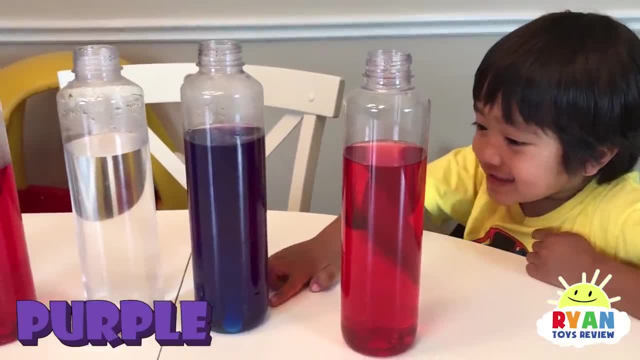 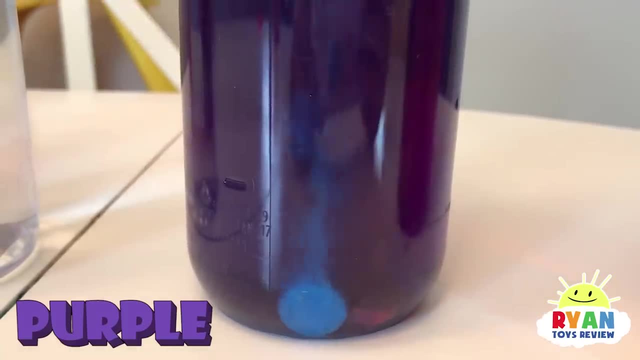 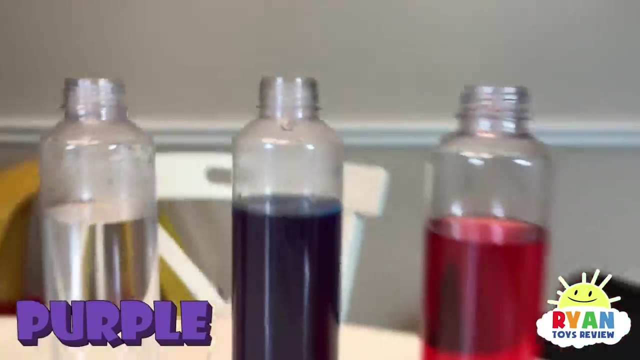 Whoa, It's so oily. I can see a little bit. Wow, there it is Blue and red makes purple. It's actually, It's actually. It's floating up. It's like blue fire, but then blue fire doesn't work. It's floating up. 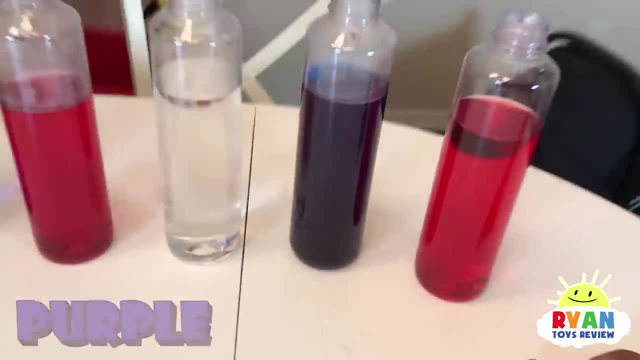 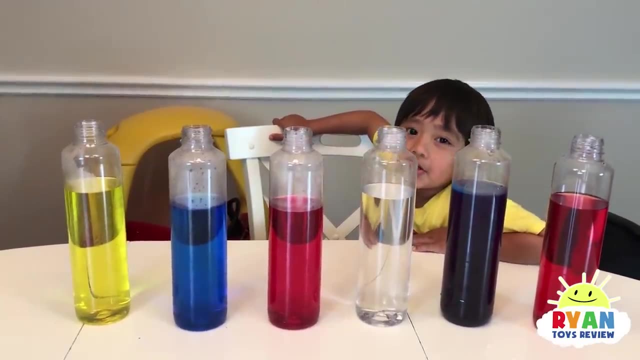 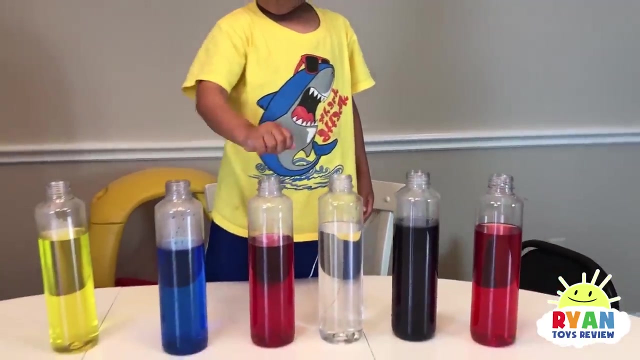 The big one's floating up. I'm not strong enough. What color are we missing? We're missing orange. I mean not orange. What's your favorite color? You're missing it. Green, Yellow and blue makes green. Maybe later. 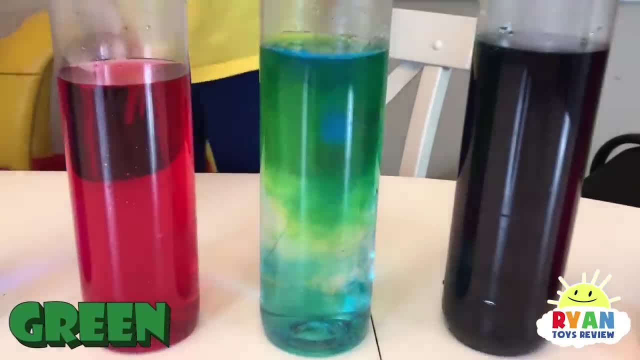 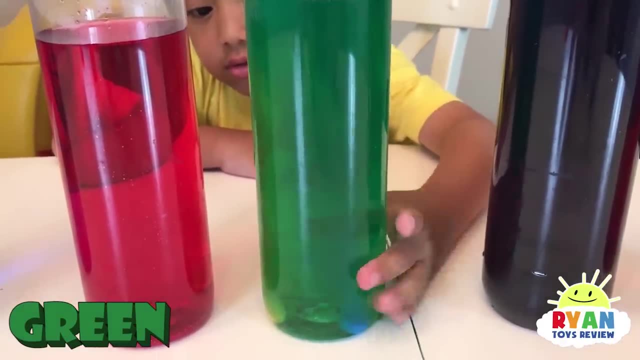 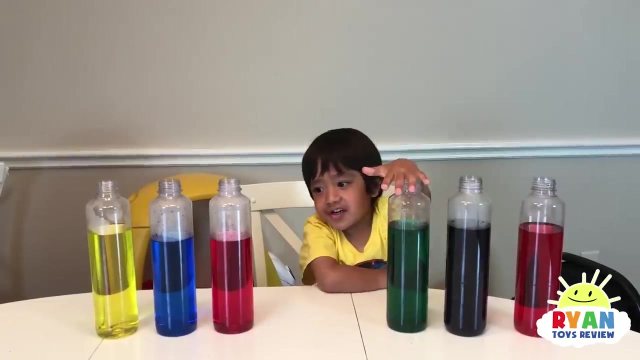 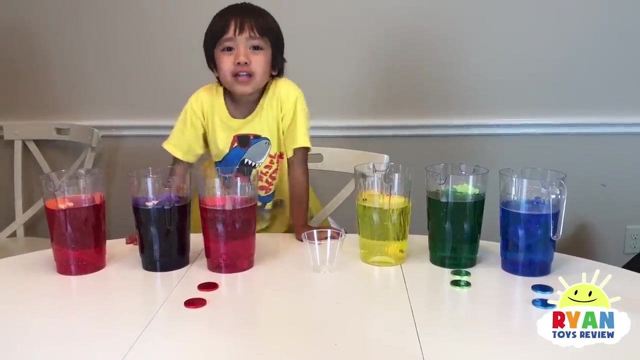 we can put the other ones in like: Yeah, There it is Yellow and blue makes green. Do you see the blue, Cool, Orange, purple, green, red, blue, yellow, Nice, Let's take out surprise toys and the colors. 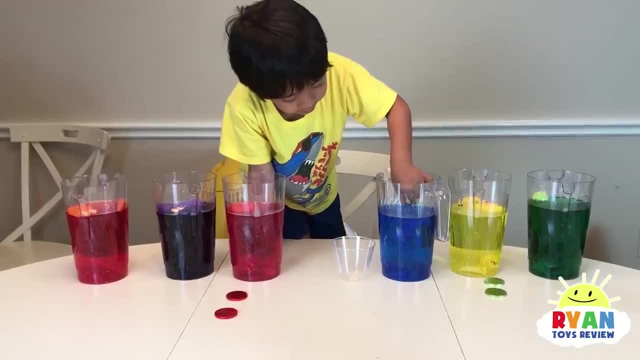 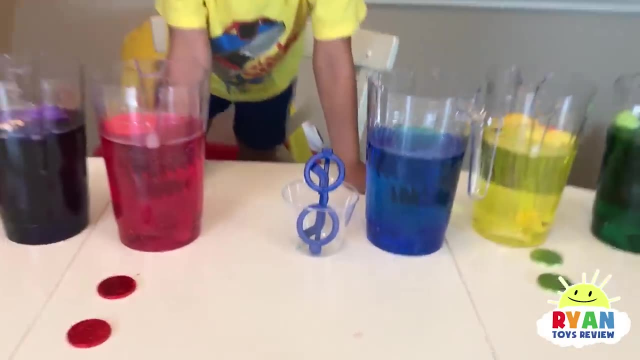 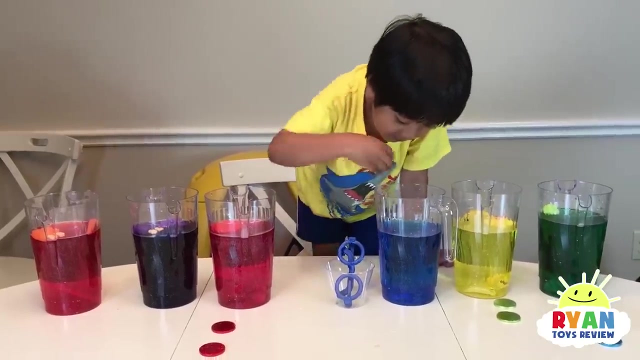 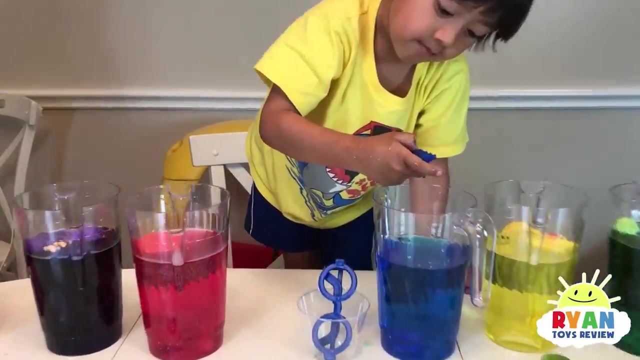 Let's see the things that are blue. What are blue? Blue glasses. That's so weird that blue glasses are blue Because there's different glasses. What else that are blue? Blue boat- A blue boat- Are they all blue? that would not. 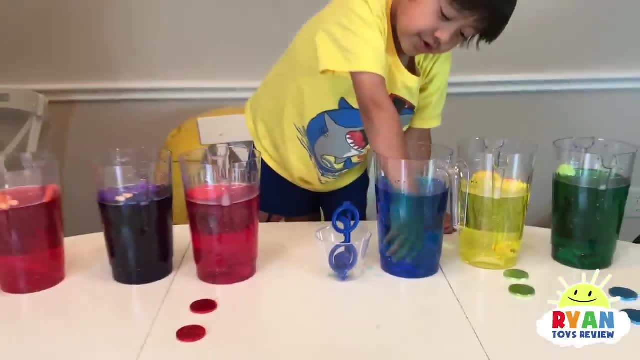 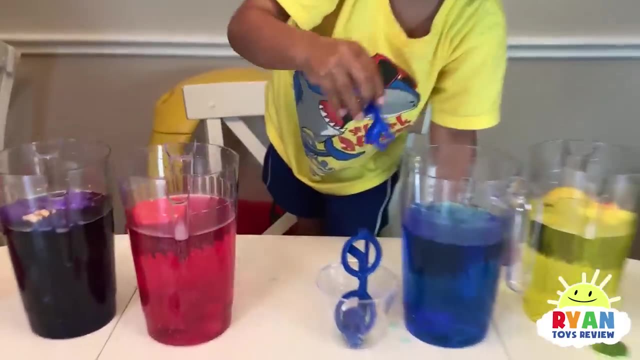 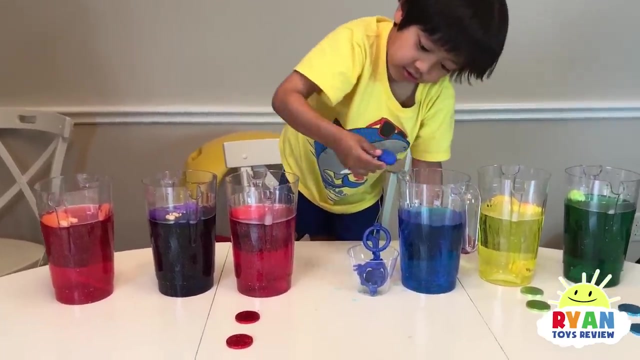 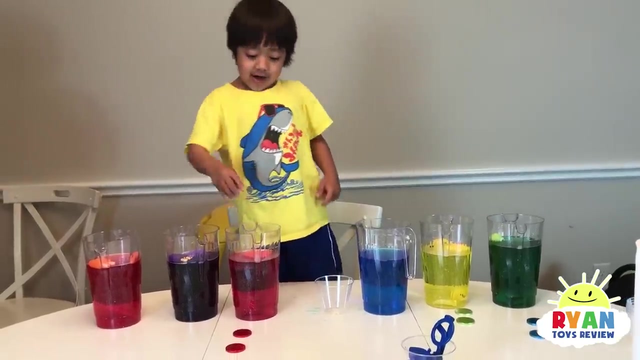 look cool What else. And Oh, this is so weird. What A blue reindeer, Oh a blue reindeer, That's so weird. And a blue backpack- Nice, A blue Blue backpack. Let's see what are red. 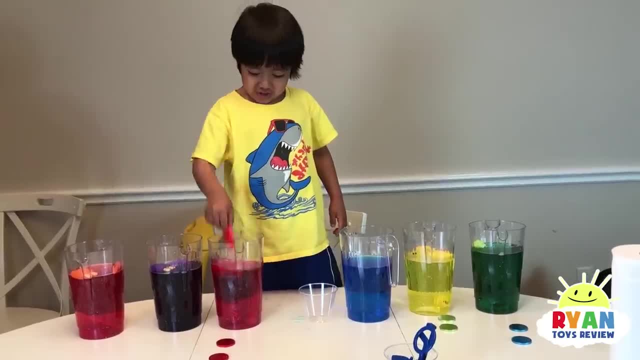 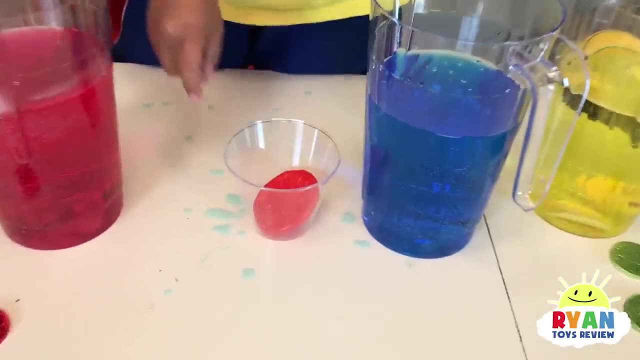 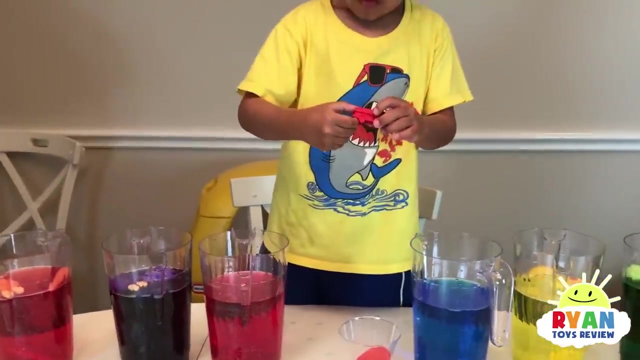 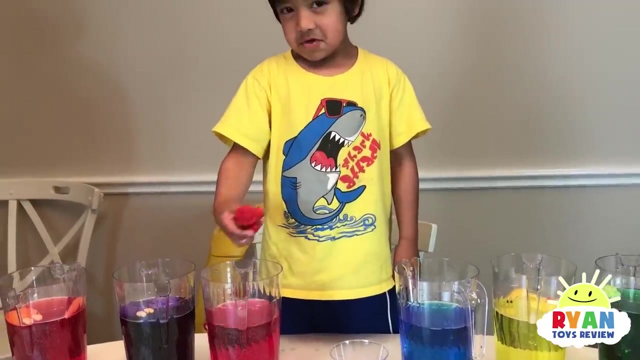 I'm floating on a boat. I'm floating on a boat For the money. I forgot this. Oh duh, I forgot this: Tomato, Tomato and fire truck. So tomato and fire truck, And fire, I mean Fire hydrant. 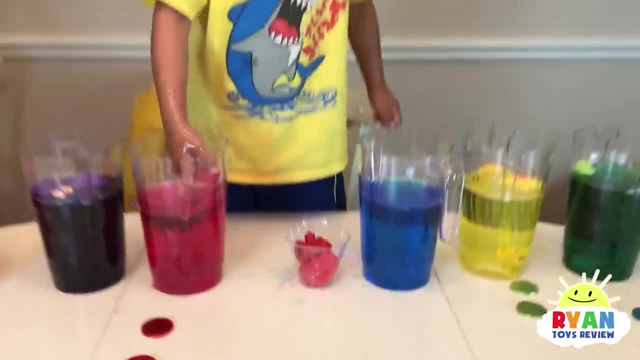 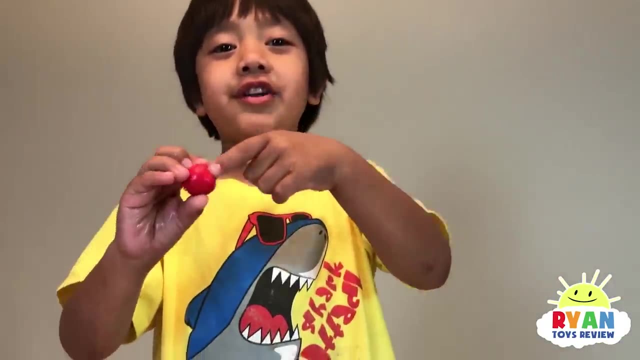 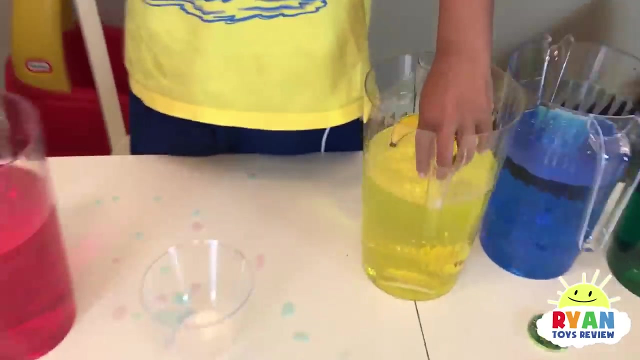 Yeah, Fire hydrant and an apple. That's so weird. The top is supposed to be brown and then there's supposed to be green leaves And an apple. Let's see what things are: yellow, Floating on a star, Floating on a super star. 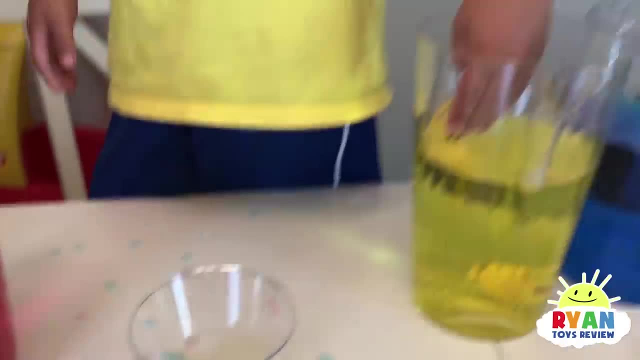 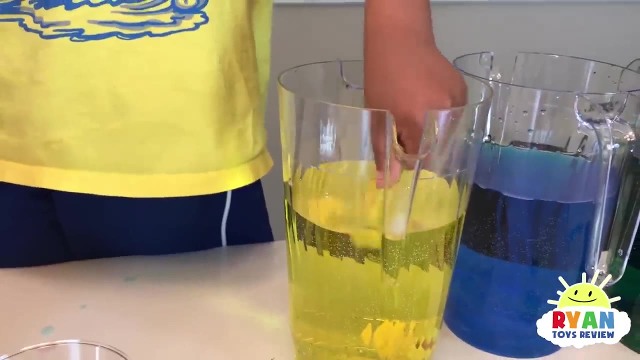 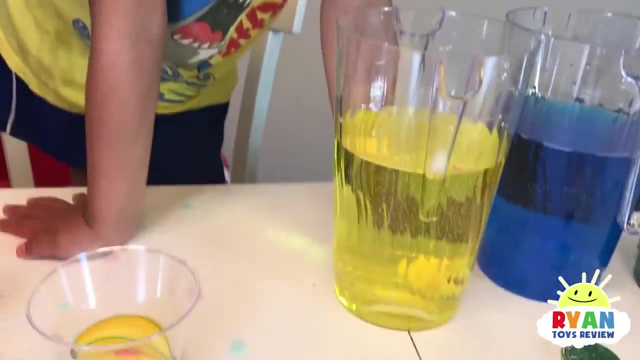 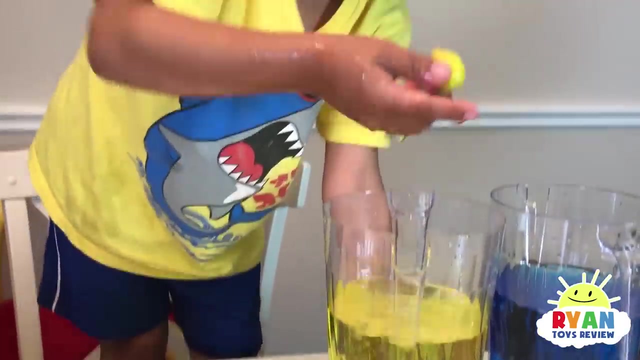 We have a star And a star: Banana. Banana Floating on a banana Floating on a sushi. Banana Chips. Get this super, duper fast. Kids Dah, dah, dah dah. What is this Lemon Weirdo? 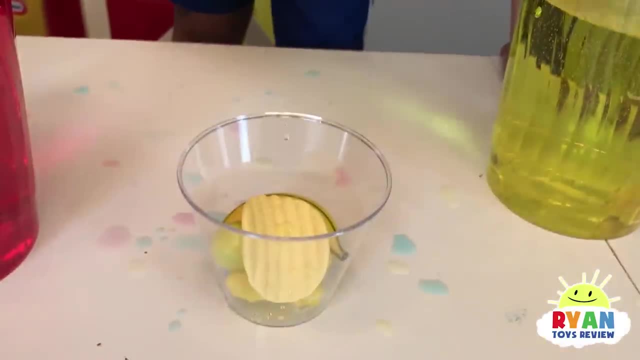 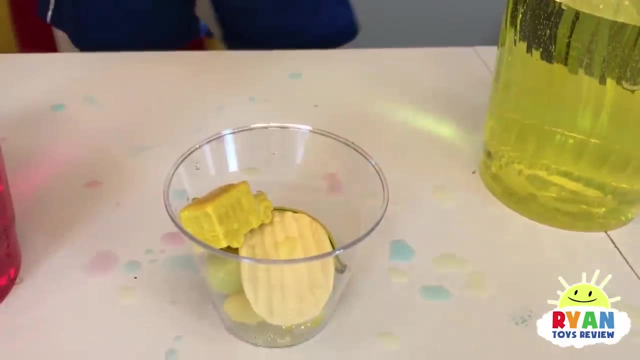 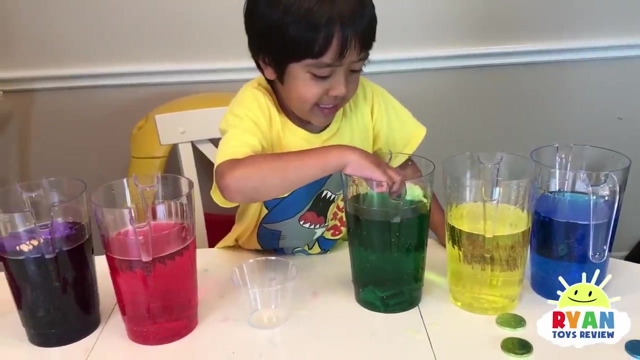 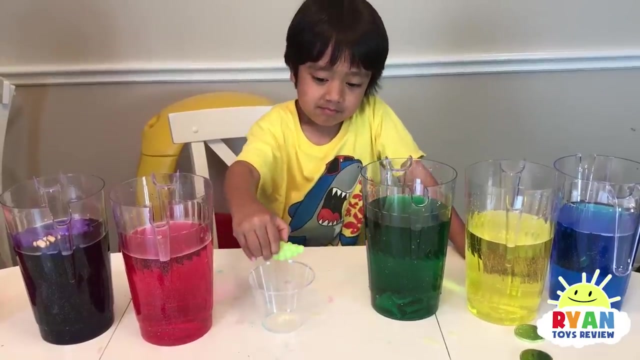 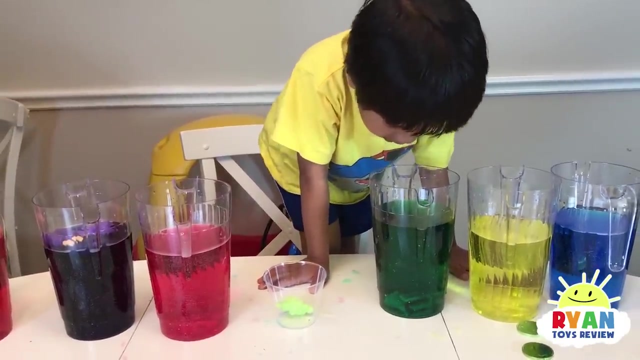 Dah Chips, Potato chips. School bus. Why is everything yellow? Yellow school bus. Let's see what things are green, Just floating on a sail ship. Green Crepes, Green grapes- Let me see some Christmas tree. We get a super fast. 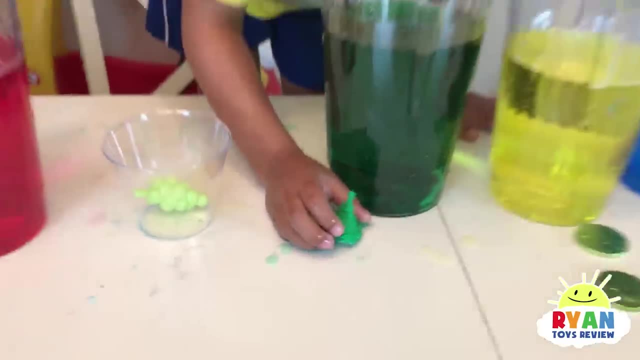 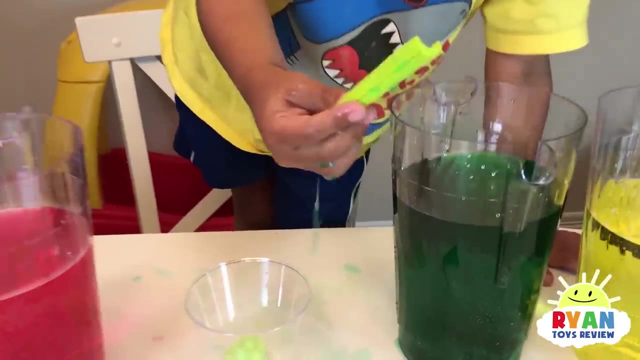 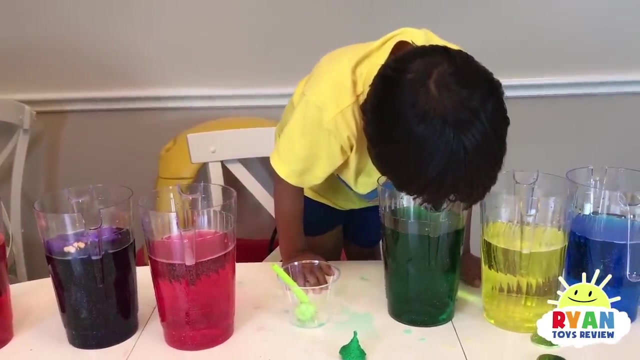 I think the Christmas tree Something needs tree. Is that a green? What else are green? Okay, Scallop, Scallop. It's real. Boiling A roach? No, I don't think so. Cockroach A roach. 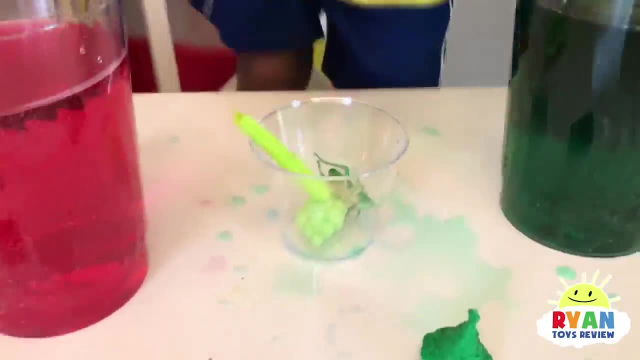 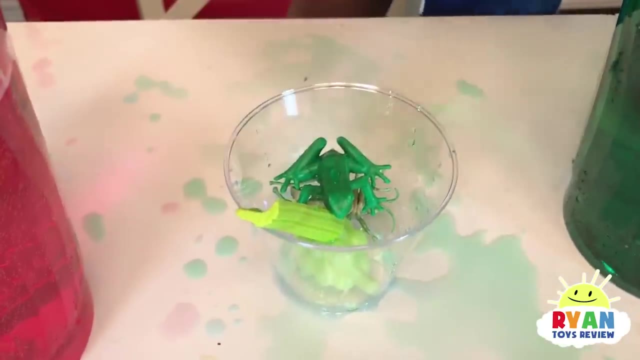 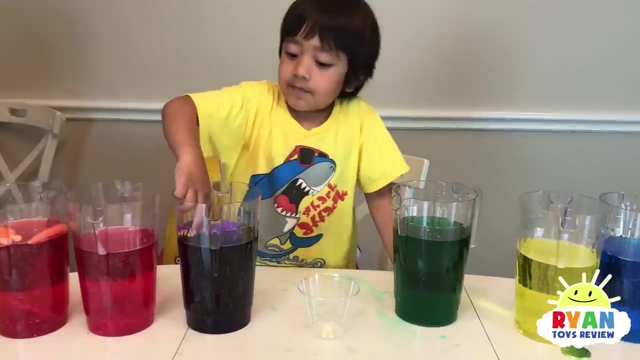 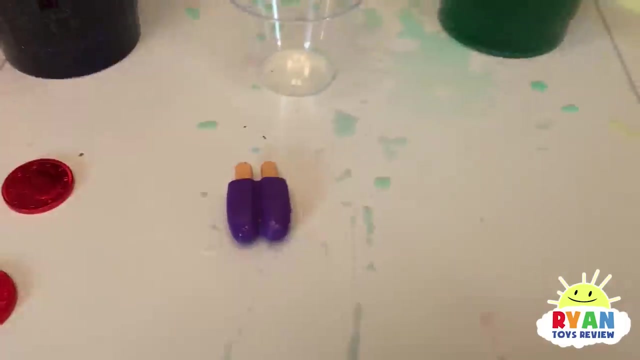 That's a cricket, Cricket, Cricket And frog. I think there's one with a, I'm not sure Let's do purple. Everything floating, What is that? one Popsicle And there's another Purple popsicle. 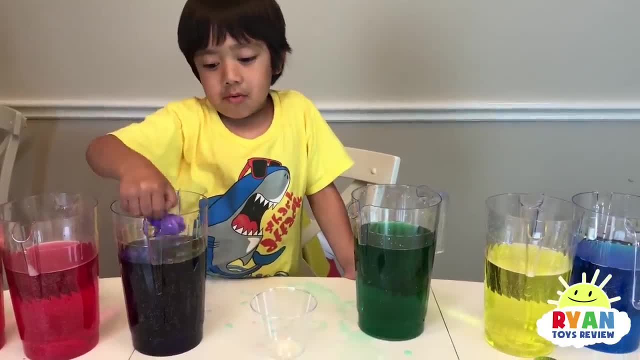 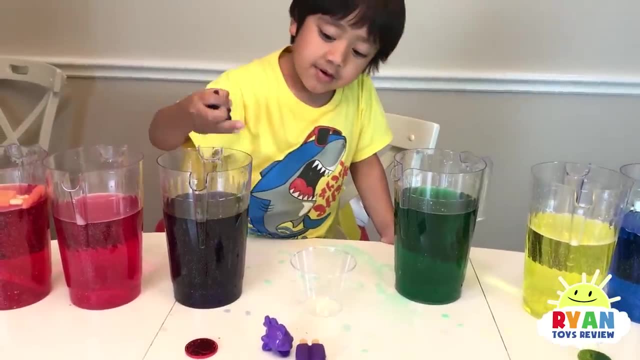 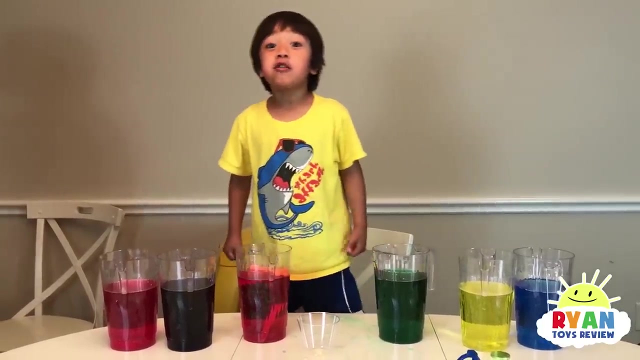 There's also another popsicle in there: Purple fish. Ah, Purple fish And Purple something. Crepes, Purple grapes. Let's see what things that are: orange Flooding, Flooding on the sailboat With super duper fast fire. 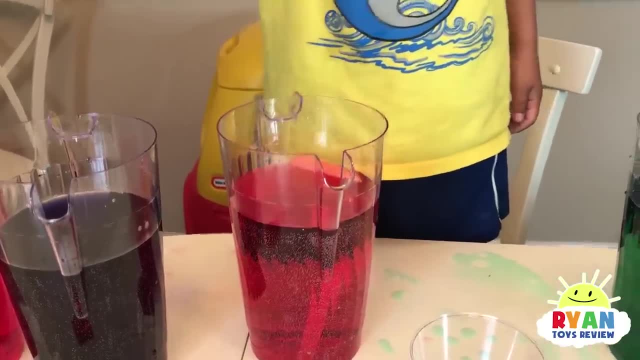 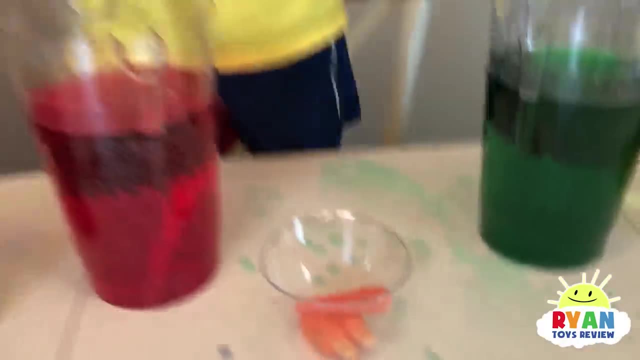 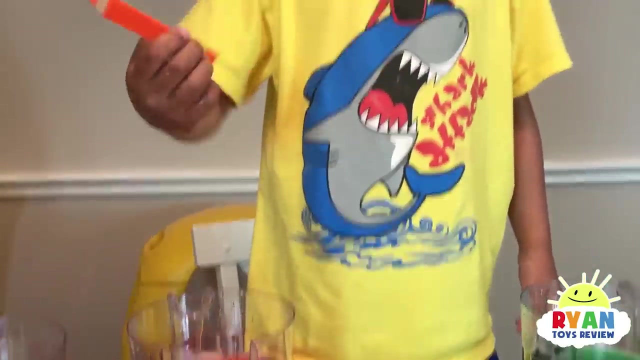 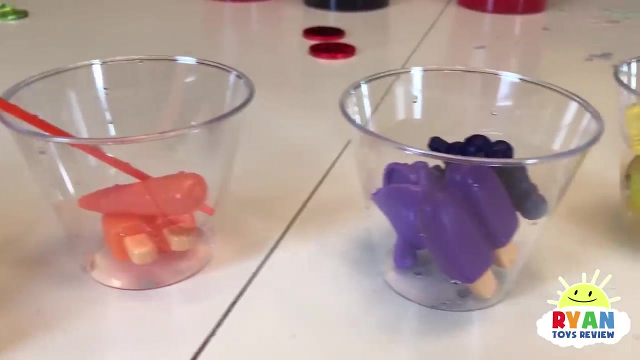 Ah, Popsicle Orange, popsicle Carrot, Orange carrot, Let me get the super duper fast. There's one more. Ah, What is that? one Crayon Orange, crayon Orange, Yellow, Yellow. 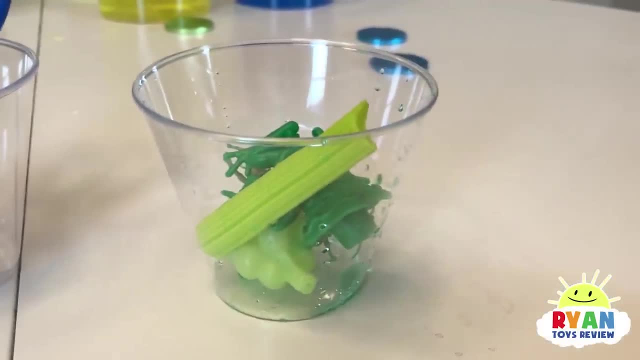 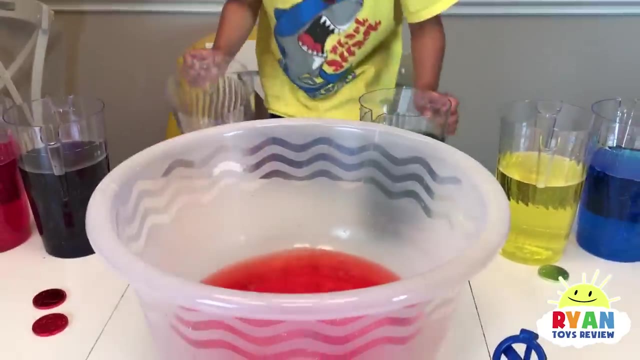 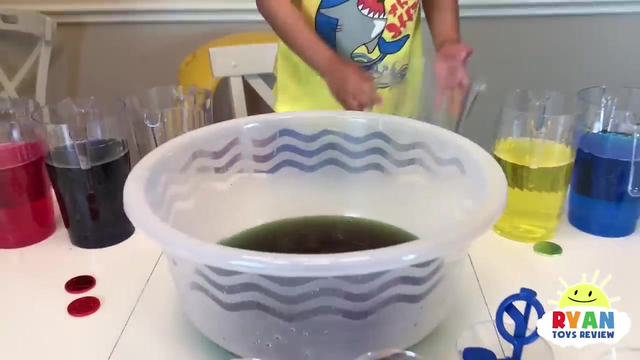 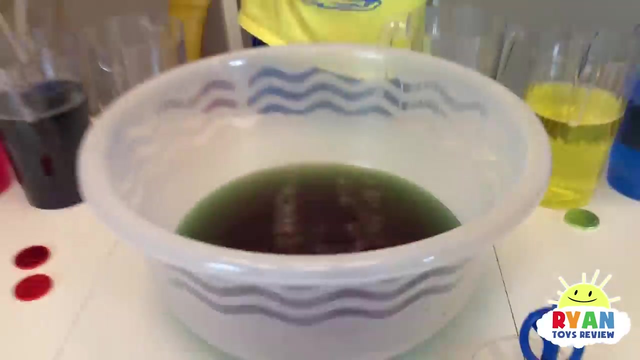 Red, Blue And green. Put in all the colors, I become white. Let's see if green is a stronger color. Green, Oh wait, Orange and green. Orange and green makes like rainbow. Alright, Here comes purple. Oh, it doesn't change the color. 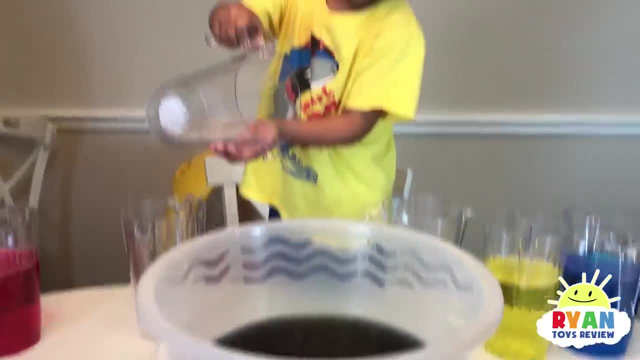 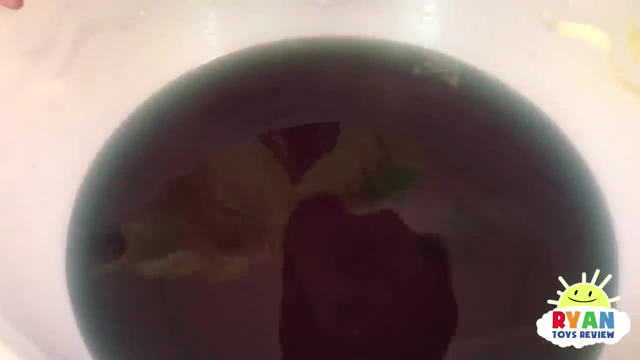 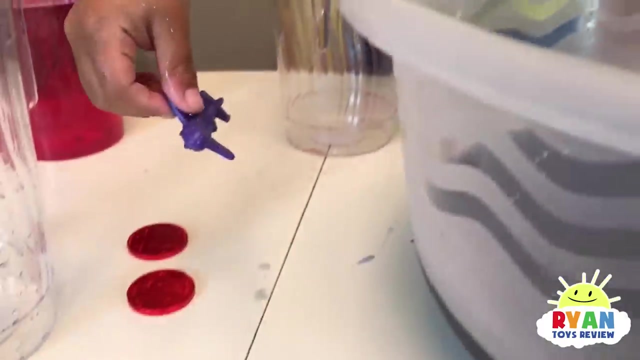 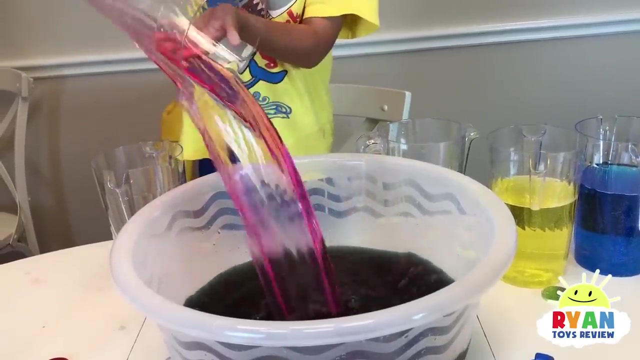 Purple doesn't. What just happened? I don't know, Maybe we missed a surprise toy. I see We missed something. Oh, what is that? Purple airplane, Purple airplane. we missed it. Red. Yeah, Oh, I see a surprise. 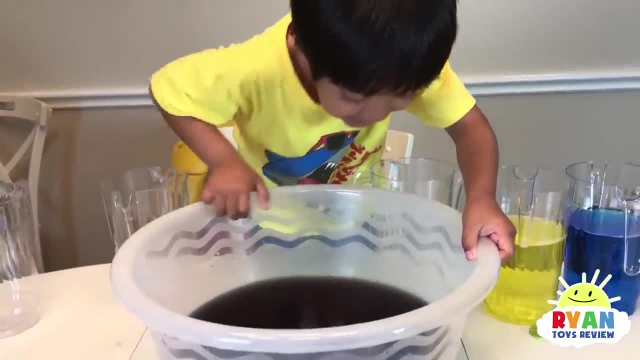 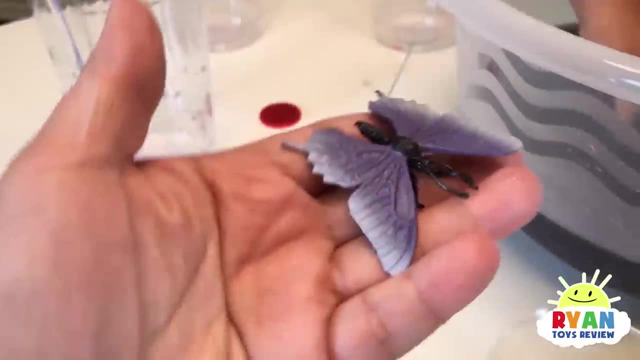 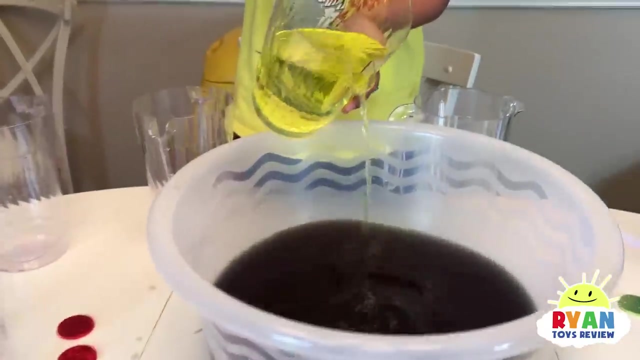 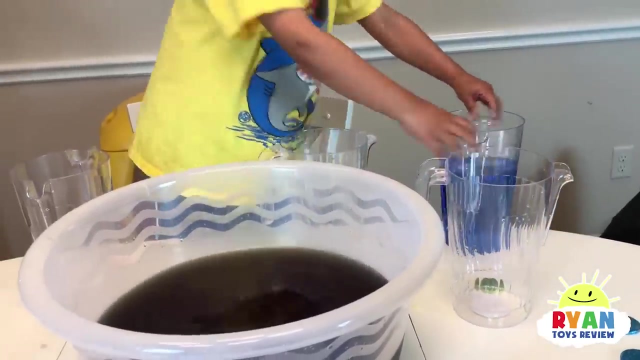 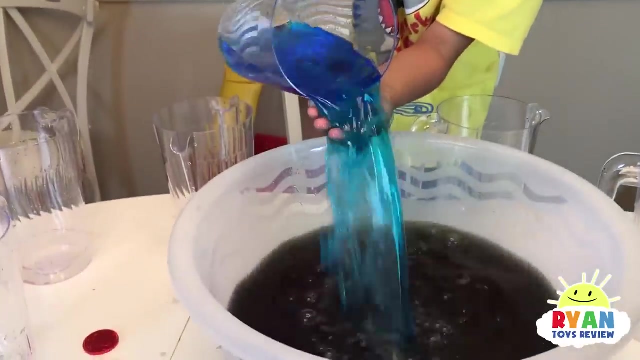 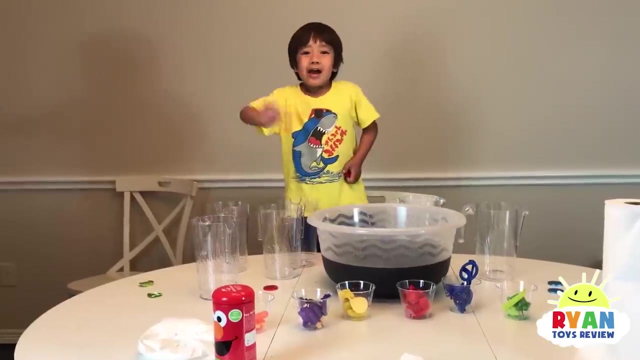 Oh, really, We missed another one. Oh, Butterfly, A butterfly, Purple butterfly, How pretty Yellow. Yeah, Looks like it. And last color is Blue, Blue Bye. Don't forget to subscribe, like and share this video with your friends. 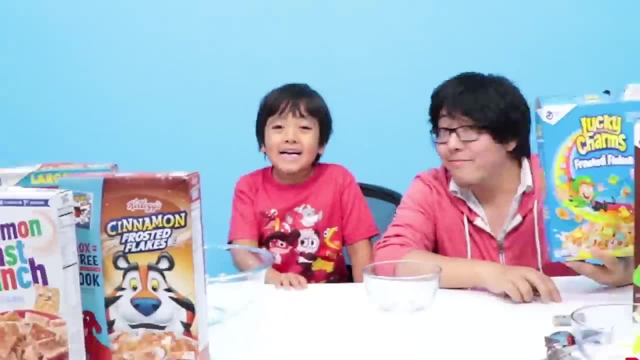 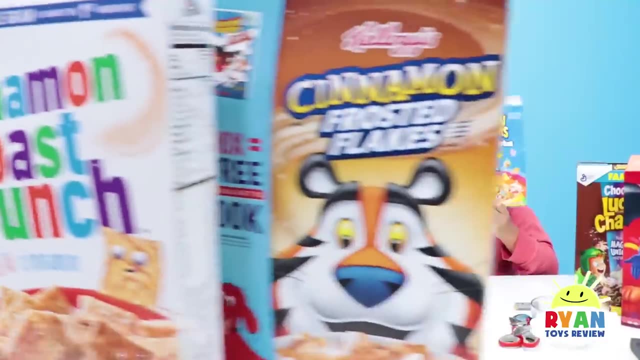 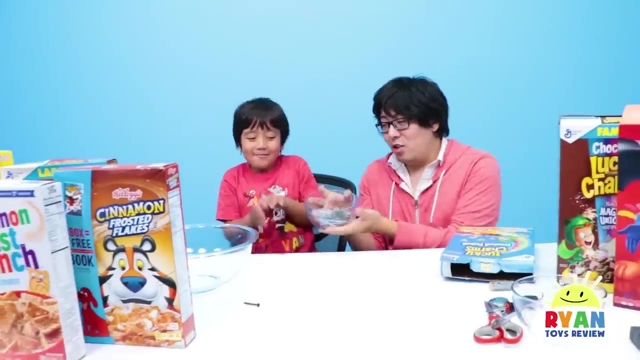 If you want more color videos, and I promise you. bye. Hi guys, today we are doing a science experiment with cereal. Did you know? cereal has iron inside, So we eat nails for practice breakfast. here's our new cereal. just kidding, yeah, we don't actually have nails in our breakfast, but 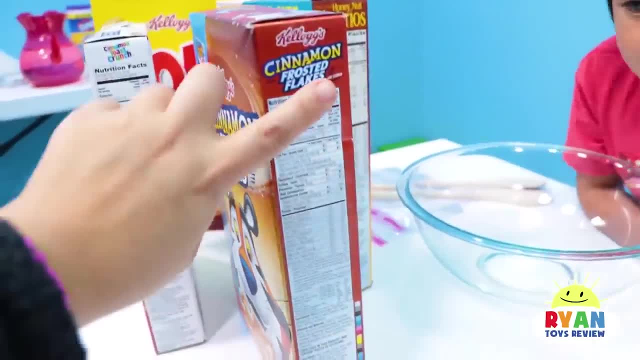 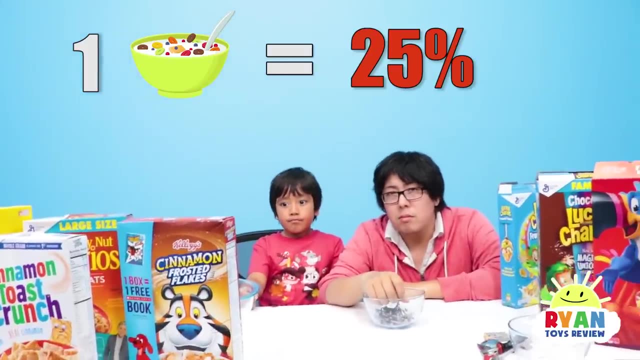 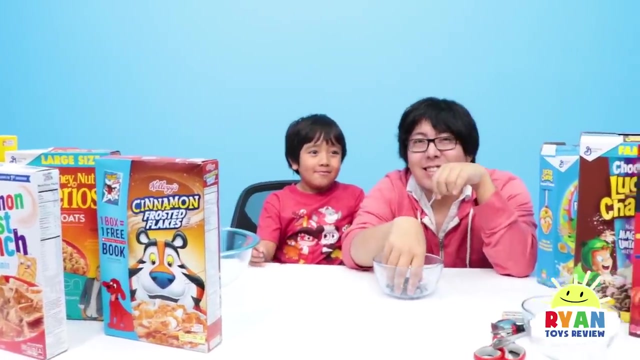 we do have iron in our our breakfast here. so if you look on the side it says 25. so that means if you eat one serving of the cereal, that you completed 25 of iron that you're supposed to eat for the day. so we're supposed to be a hundred percent of iron. yeah, you know why iron is important. 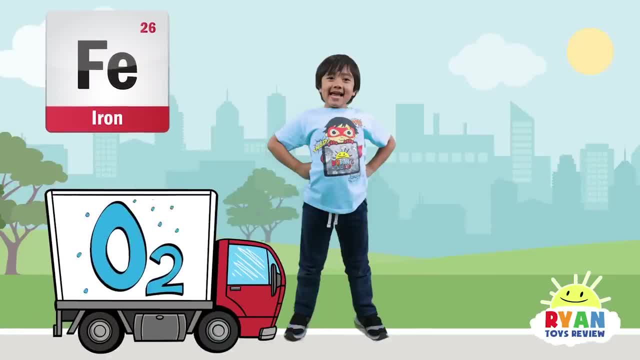 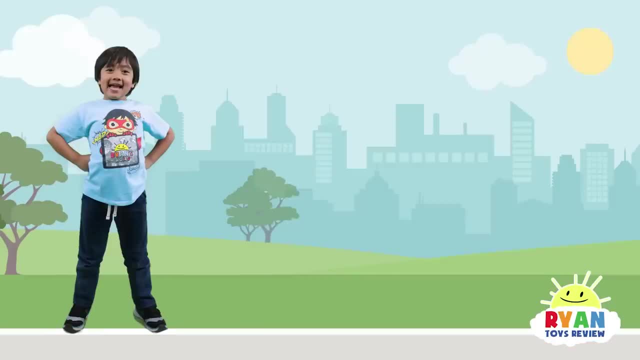 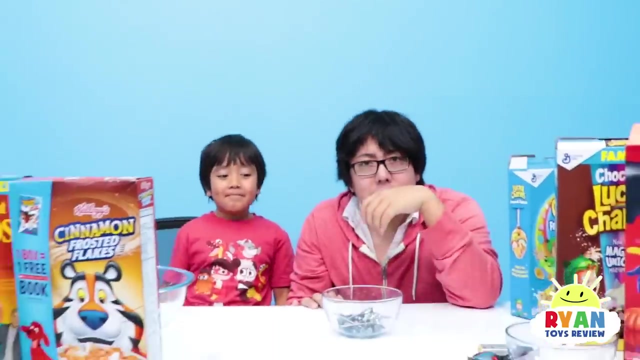 ryan, why iron helps transport oxygen all over your body? ah, the red blood cells. and why do you need oxygen? uh, to breathe. iron also help your body get rid of carbon dioxide. do you know who needs carbon dioxide to survive? plants exactly. carbon dioxide is coming out of my mouth. are you ready to test? 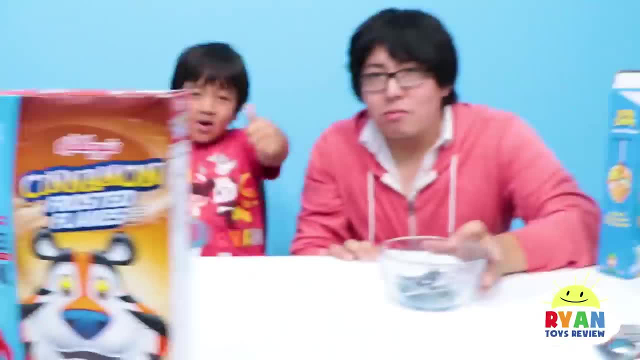 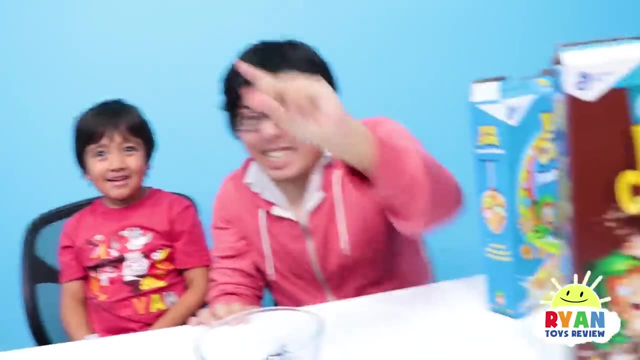 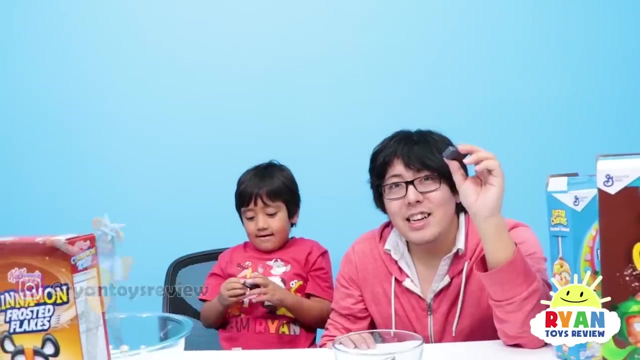 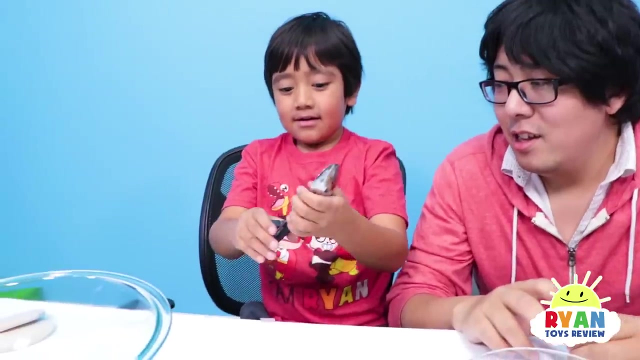 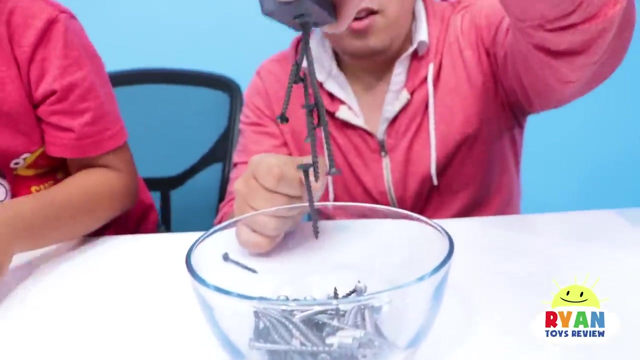 oh yeah, and find iron in your cereal boxes and you know how we're going to test, how you can pick up things that are metal with magnets, for example, so you can pick up those nails. i'm not holding it, look at that. here's some other things that are metal, like your batteries. 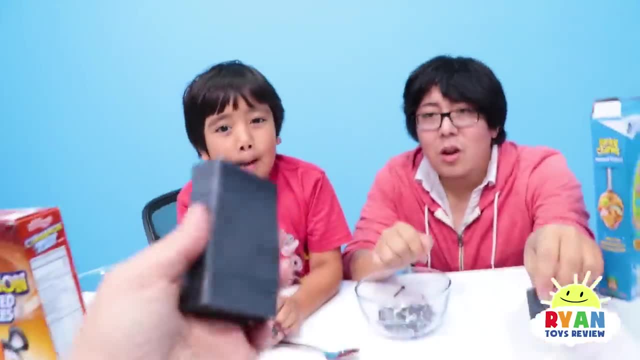 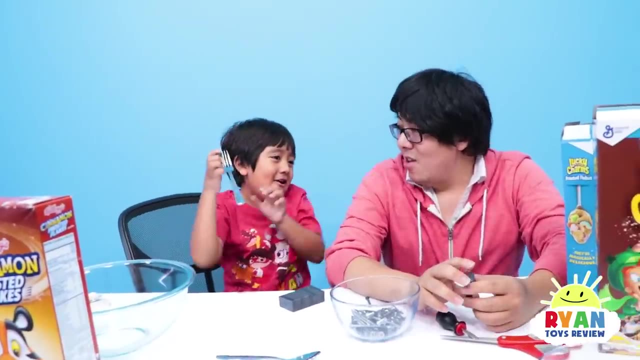 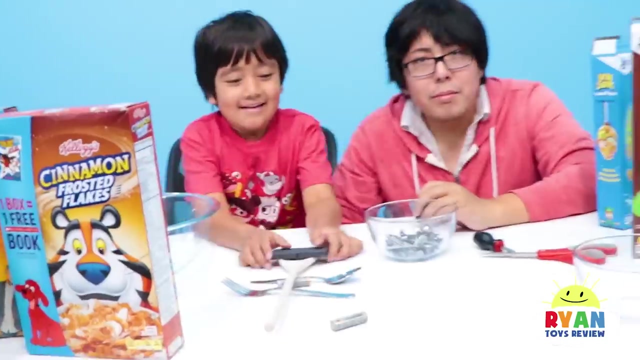 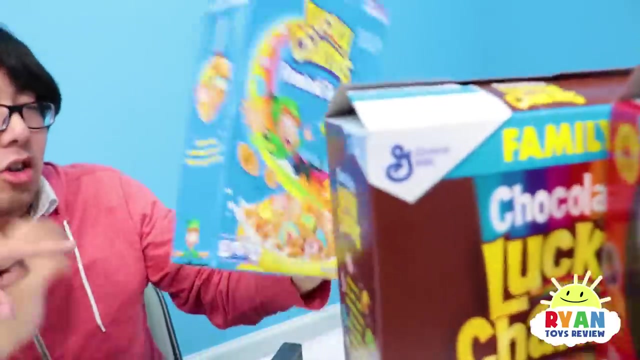 my batteries. so it's fun just to go around the house with a magnet and see which one's metal would a magnet pick up? this wooden spoon pick it up? no, no, it just falls. are you ready to see if there's iron in your cereal? yeah, which cereal you want to try? lucky, lucky charms, it is. 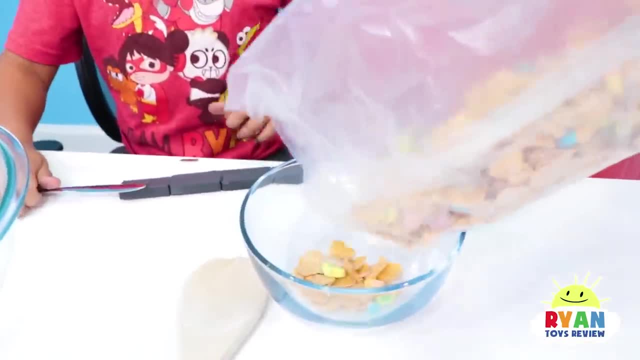 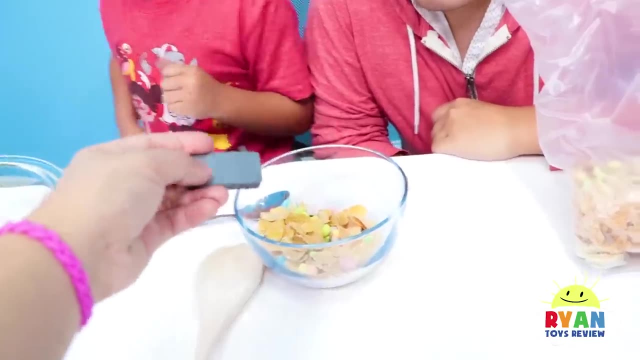 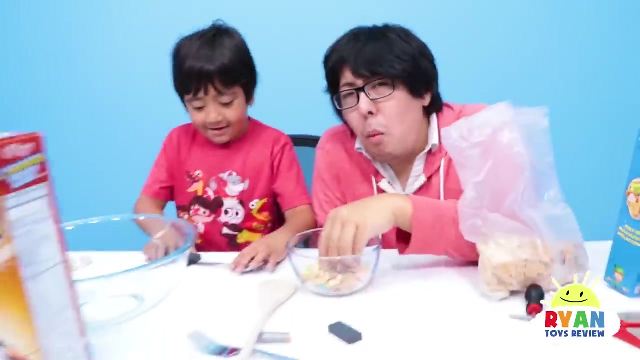 lucky charms. let me test one thing. the magnet here you can try, but it doesn't pick up the flakes. you know, other things are dissolved into this plate, but we're gonna have to mix it together with water. we actually gotta smash it. okay, three, two, one. this is a bun. 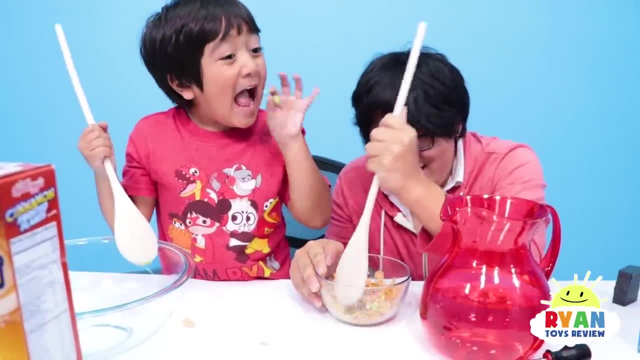 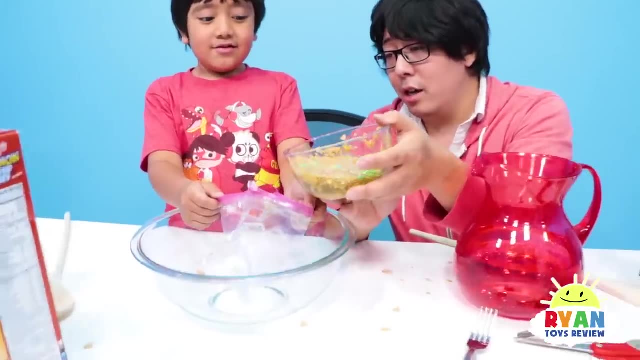 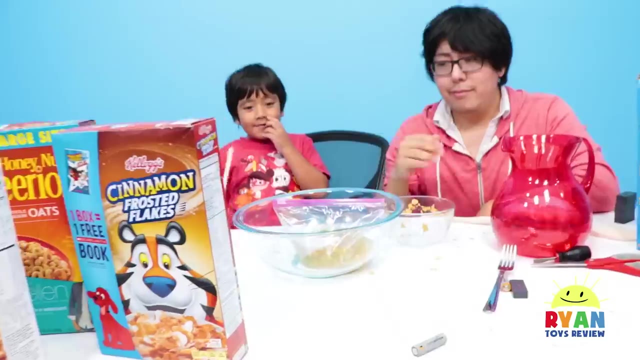 yeah, all right, eating it. look at iron. i'm going to pour this into the zip lock. looks cool. i'm going to try not to spill it. sorry if i get on your hair on here. good, zip it up. so now we have our bag here, so we're going to just mix it. 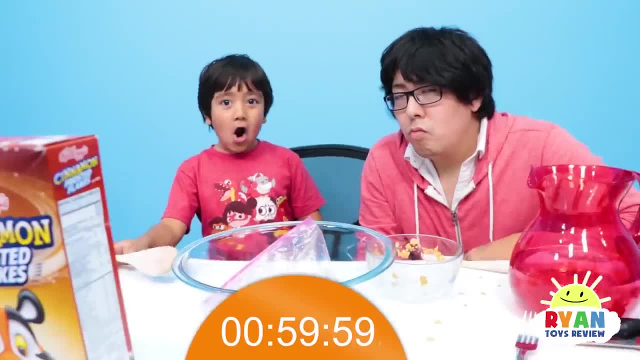 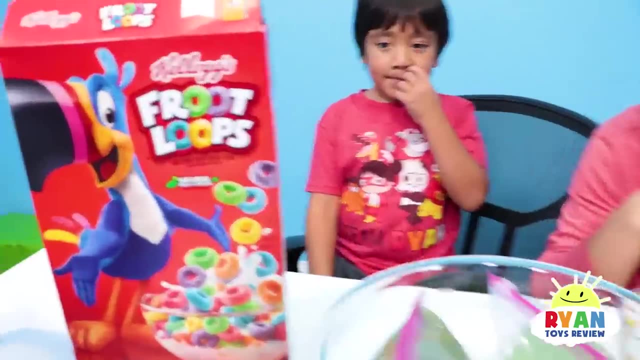 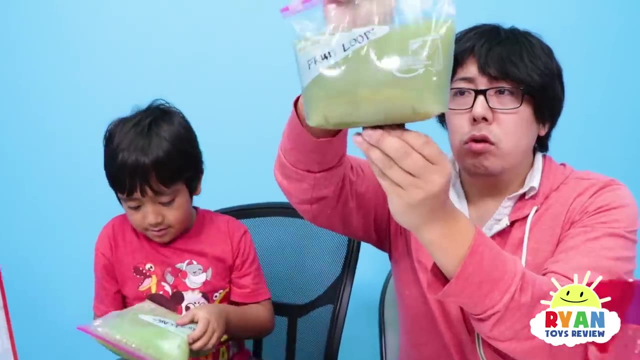 and dissolve it, and we're going to wait about one hour and then we can test for iron. you guys have been one hour and while we wait, we actually did another one with fruit loops and then after one, where there it is, you got your magnet magnet. so you actually have to hold the magnet at the bottom. 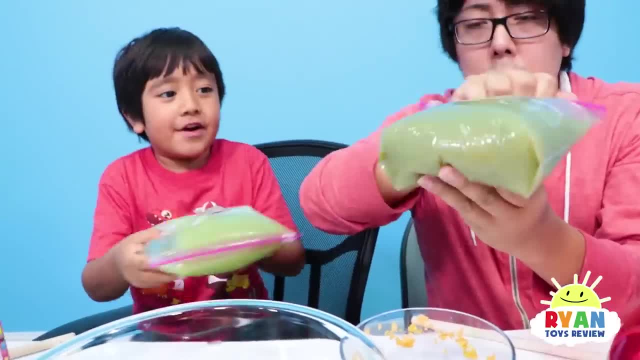 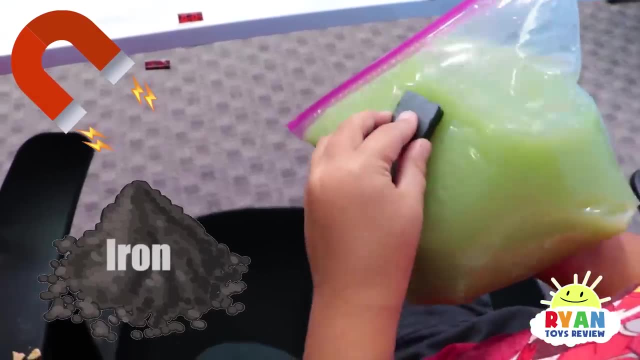 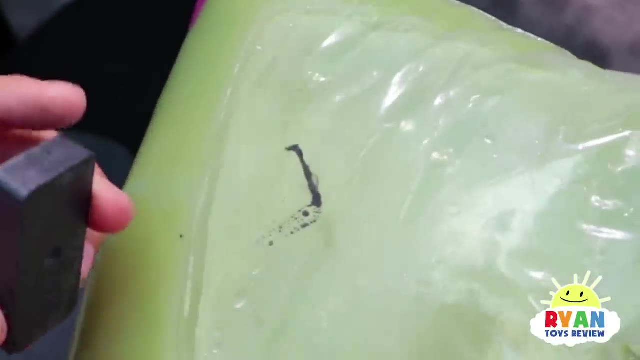 that way, all the magnets can collect together. do it for like 30 to 20 seconds and then do you see the iron. let's see whoa see it. oh yeah, i saw it. i saw it come back. whoa, there's iron right there. whoa, you see what goes around. yeah, you got all the iron to separate. 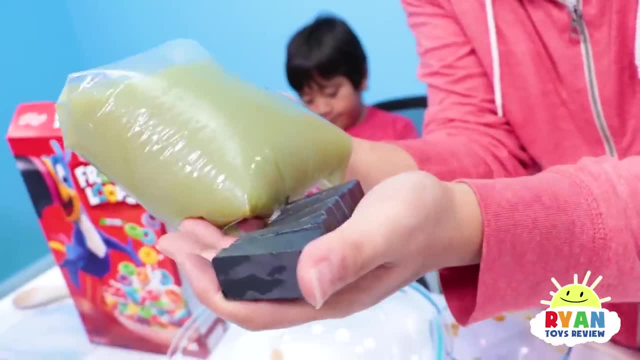 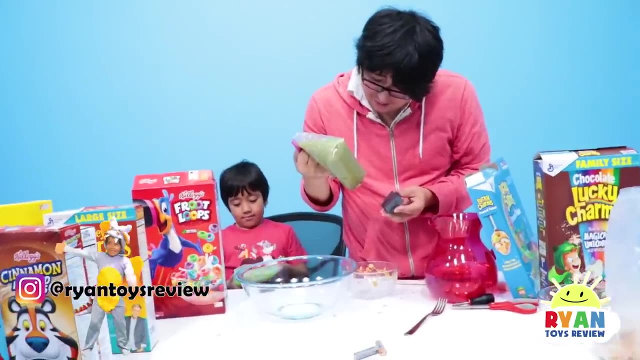 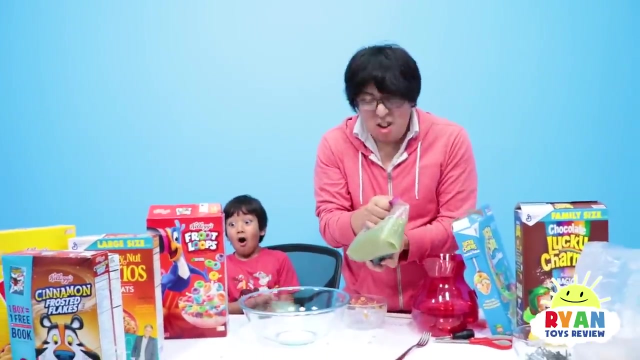 did you see it? no, i swear, i saw it. hopefully you guys try this experiment at home and there's actually some cereal that has a lot more than others. i've seen cereal that sounds like a hundred percent iron. yeah, if you guys try that experiment out, let us know. thank you so much for watching. 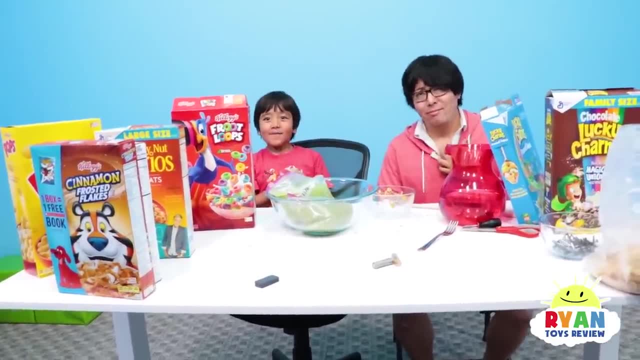 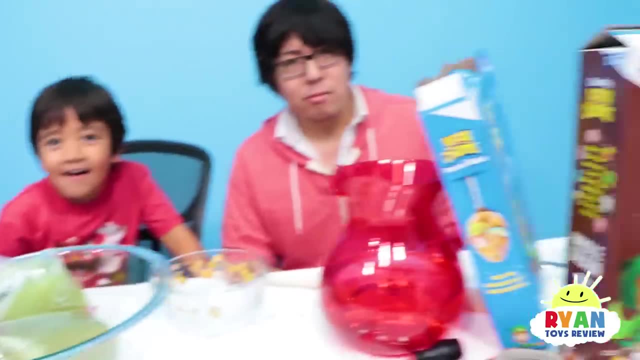 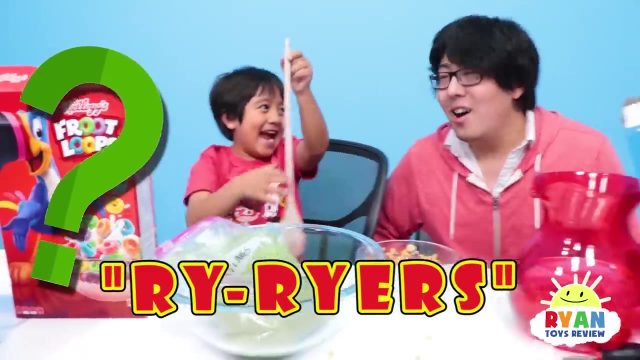 bye guys. let us know if you try this fun science experiment and let us know what other science experiment we should do and let us know what other cereal you guys try. that we didn't try. and ryan actually has a new nickname for his fans: right, right here, right, ryers. yeah, right, ryers. yes, you guys are rye. 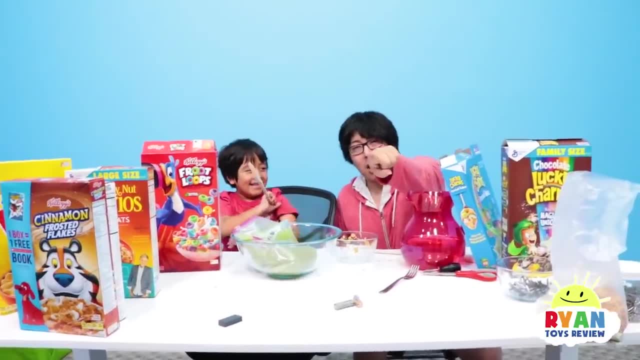 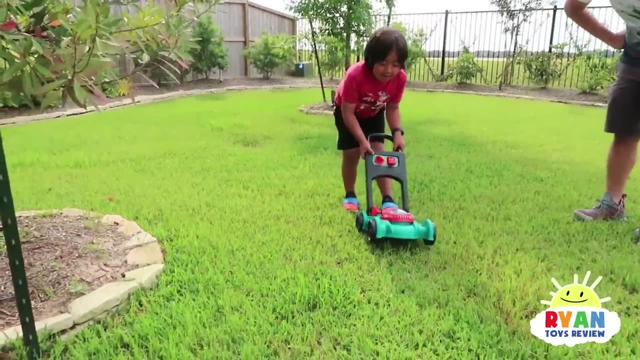 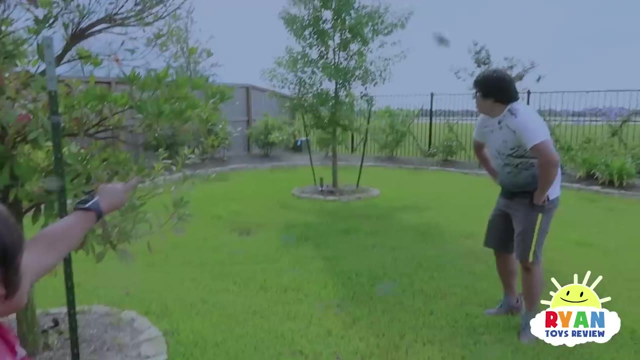 ryers, let us know if you like that name. please leave it comment below. thank you for watching for now. bye, bye, bye. hi guys, i'm mowing the lawn today. oh, thank you, ryan, you're a good helper. oh wait, daddy, there's your cereal tornado. 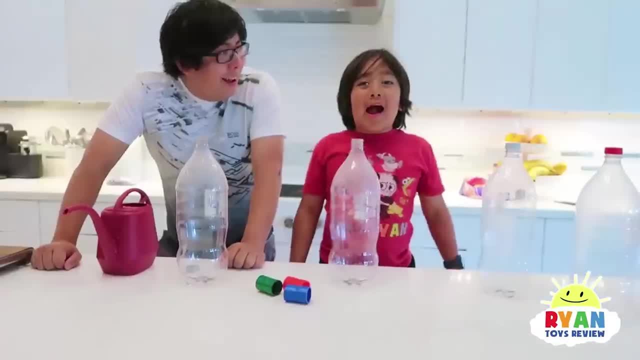 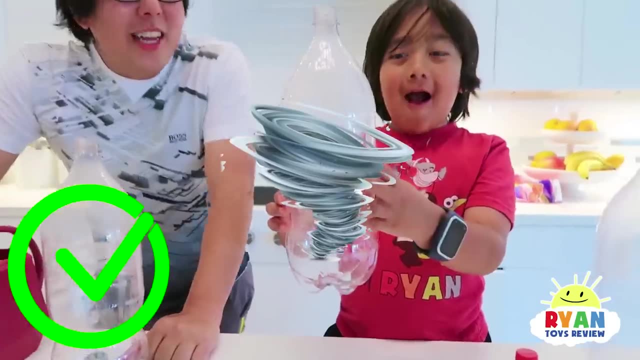 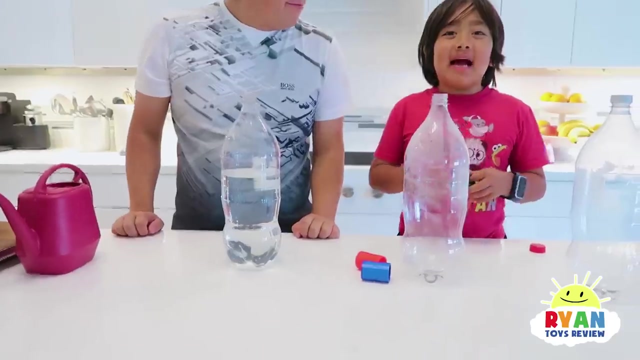 go back inside the house. wow, i can't believe that was a real tornado. but what if we make our own tornado in a bottle? well, that's a good idea, ryan. all right, good. good job, ryan. i think that's enough. next i'm gonna put on a connector. all right, okay. 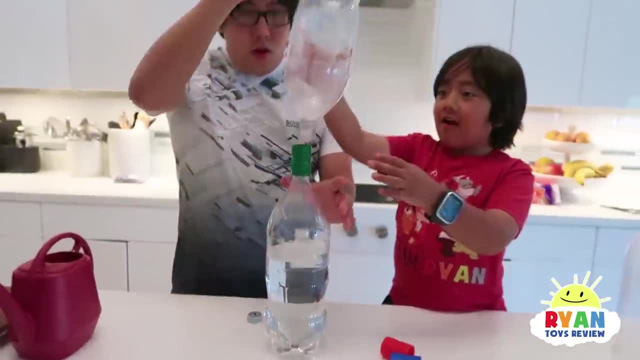 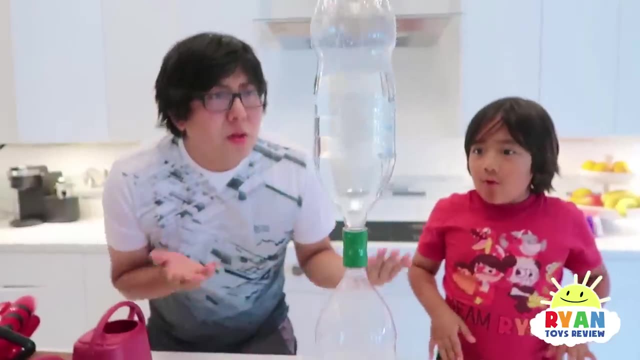 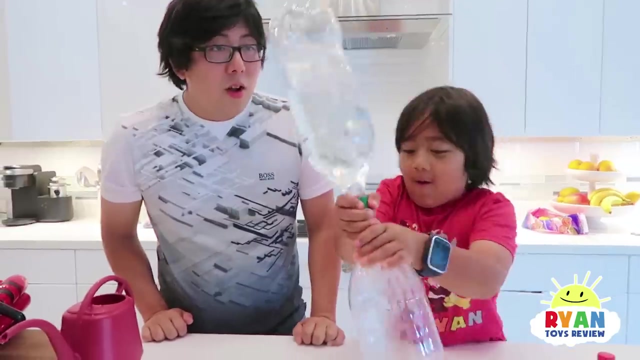 twist, twist, twist. good, this here, wow, it's so cool, it's connected now. now we do this, there's no tornado ryan, nothing's happening. maybe we twirl it. this part is hard, so i'll do it for you. okay, twirl it, twirl it. 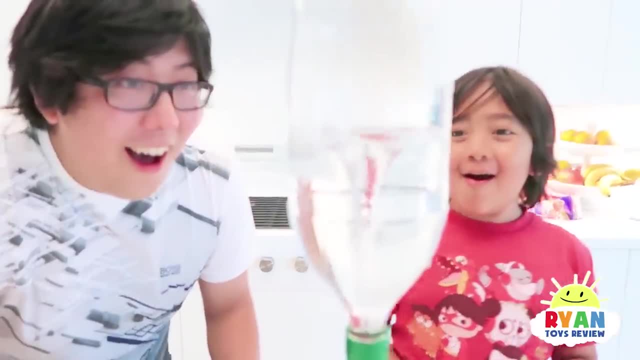 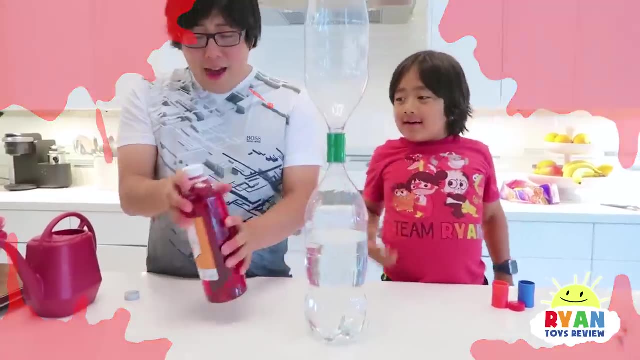 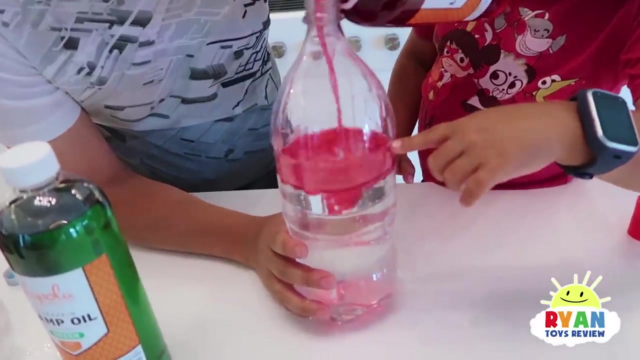 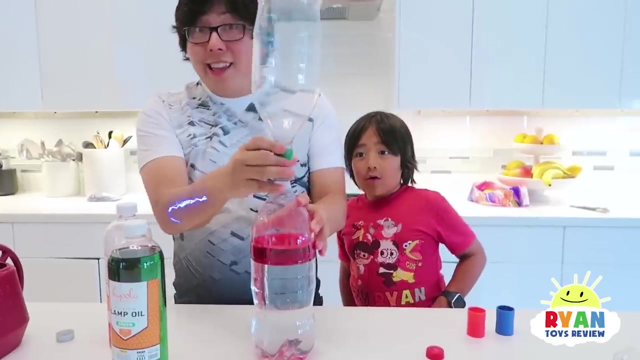 there you go guys. look, look, look, oh, wow, so cool. look at that, dad. what about us? oh, we add some color. yeah, we can use this lamp oil first. we're going to try red. here we go. that's good. kept going almost there done. now connect it again. 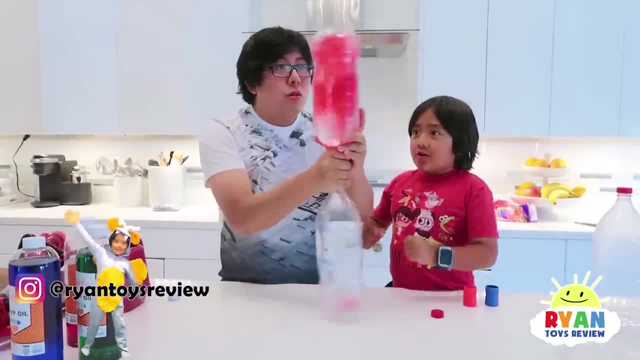 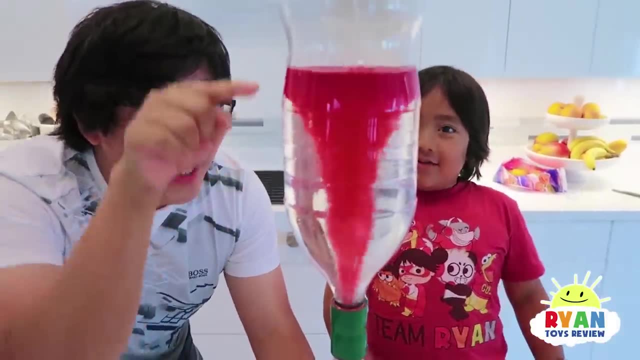 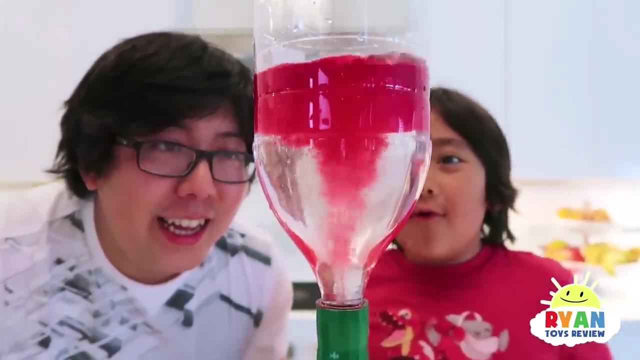 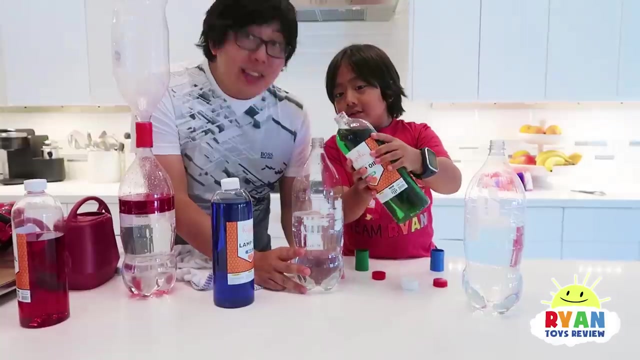 what happens. are you ready? whoa, wow, look at that tornado so you can see the tornado part is a lot better. So the center of the tornado is called vortex and that's what you see in red. You see that spinning around. Let's start with a green one first. This time Ryan's gonna do it. See if you can put the green oil in there. 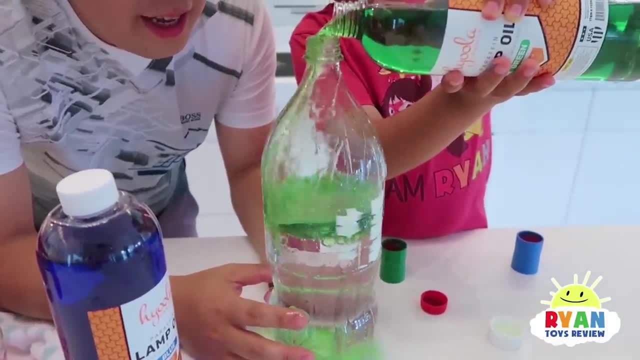 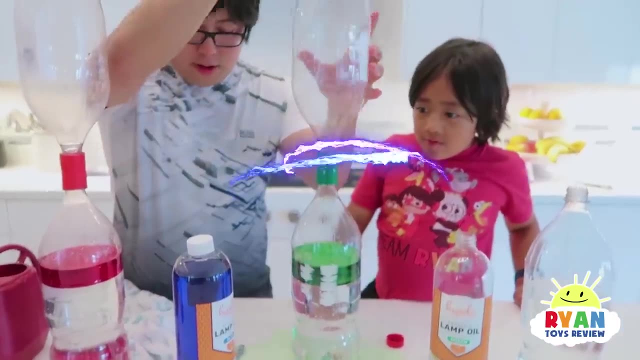 Steady, steady, steady. Ah, you're spilling it, He's spilling it. Alright, good, good, Put the cap on. Hey, give me the yellow one, Put it on and done. Nice, Now let's do the blue one. 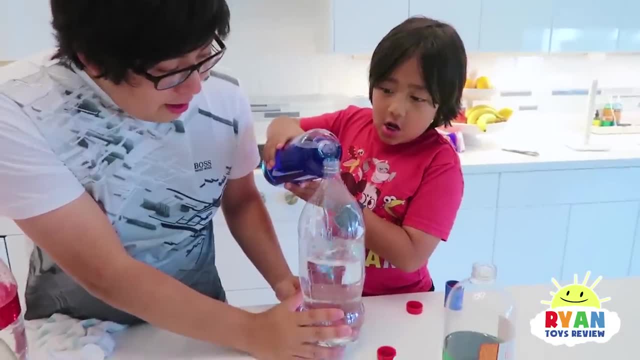 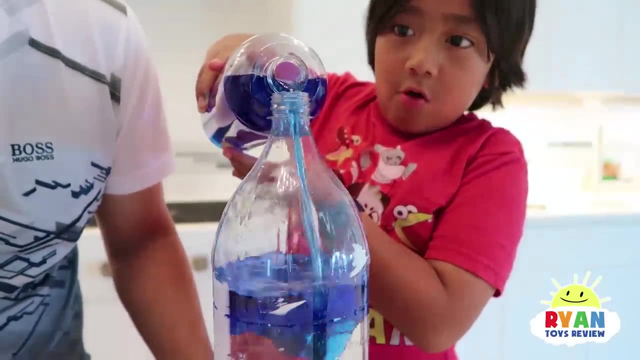 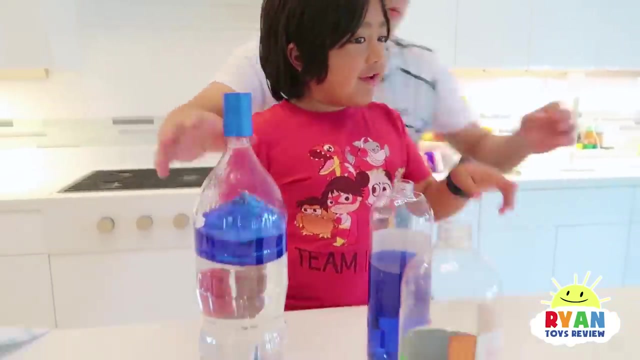 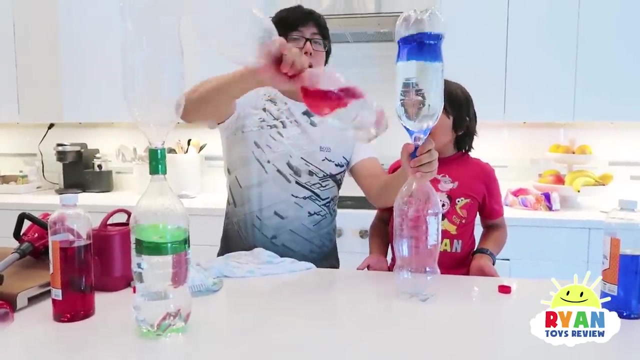 Alright, here we go, Doing good so far. Keep going. I think that's good. Alright, good job. Let's put the blue cap This Done with the other one Done. Flip it first This. Are you guys ready? 3,, 2,, 1, go. 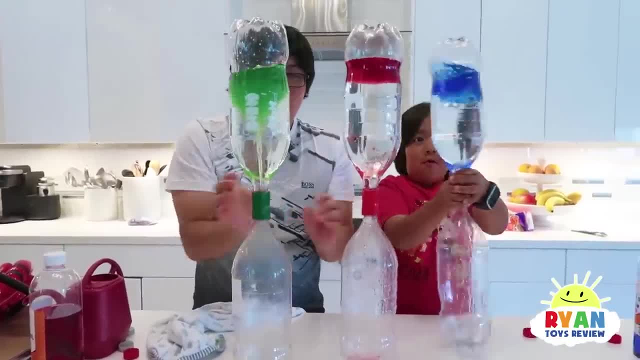 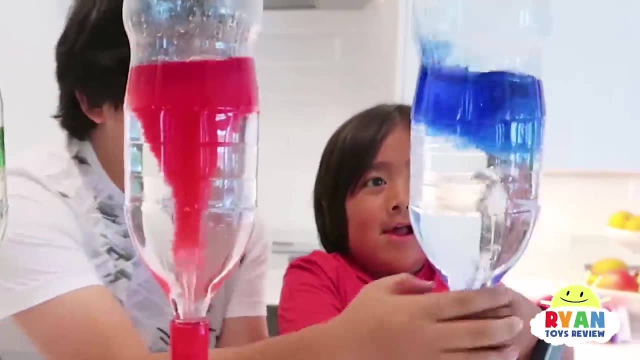 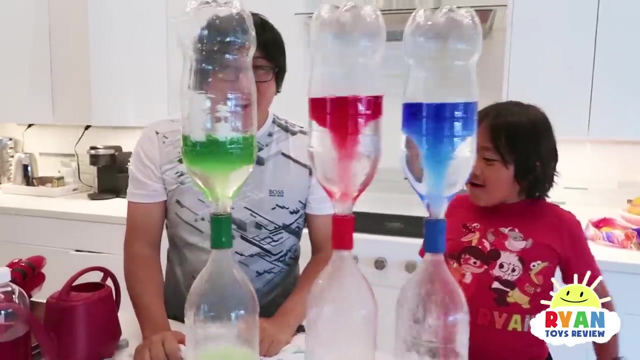 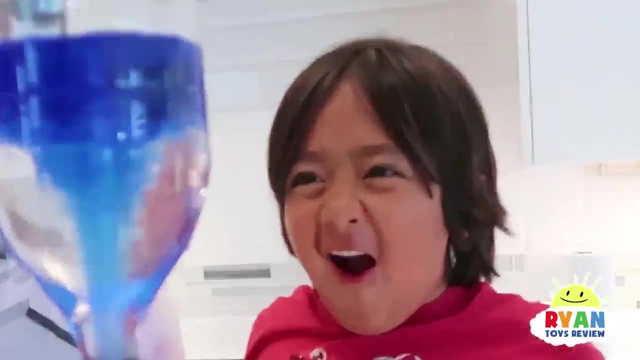 Alright, here we go. There you go. Look at that So cool, Here we go. Wow, So cool. Nice Green, red and blue- All different colors. That was so much fun. Thank you for making tornadoes. 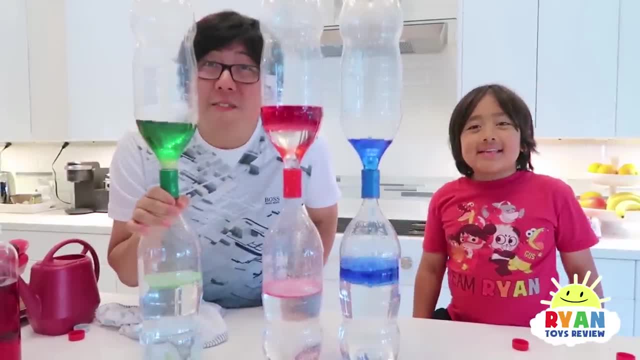 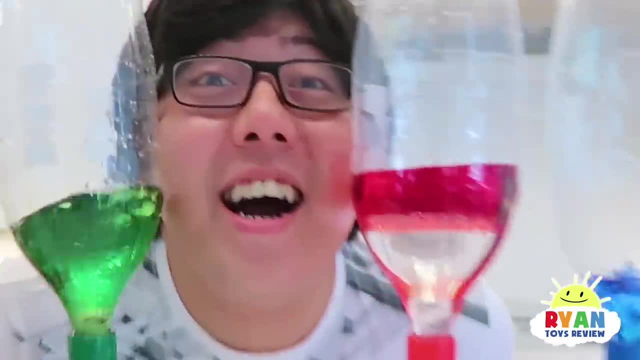 Thank you for making tornadoes with me, Daddy. Yeah, thank you, Ryan. I hope you guys have a fun time And remember always: stay happy and rise up. Bye, Stay healthy, Bye. Ah, Yuck, Yuck. 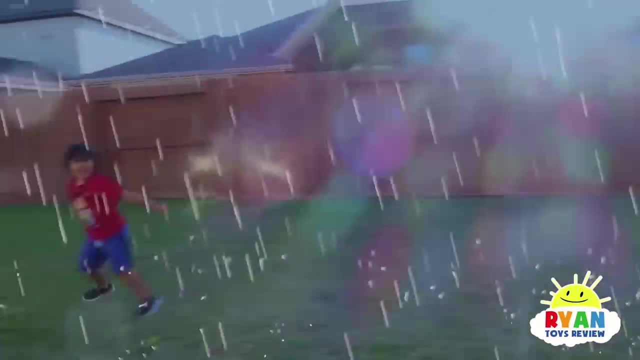 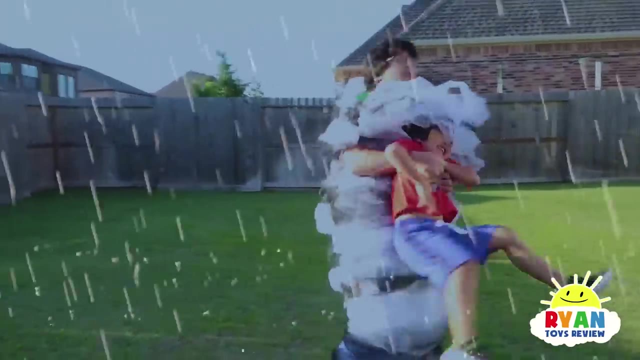 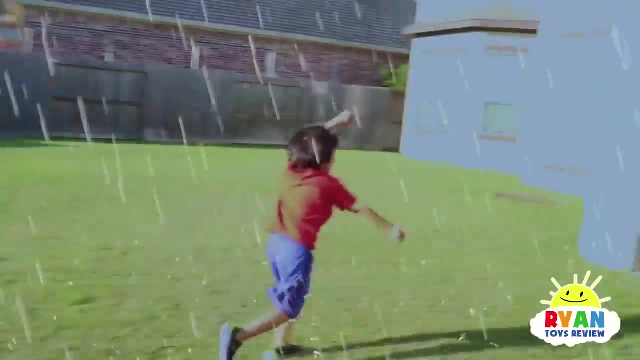 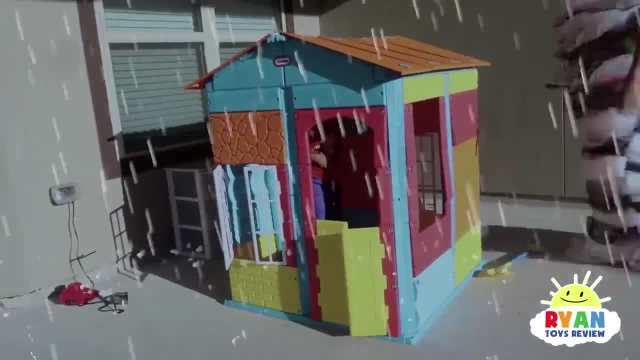 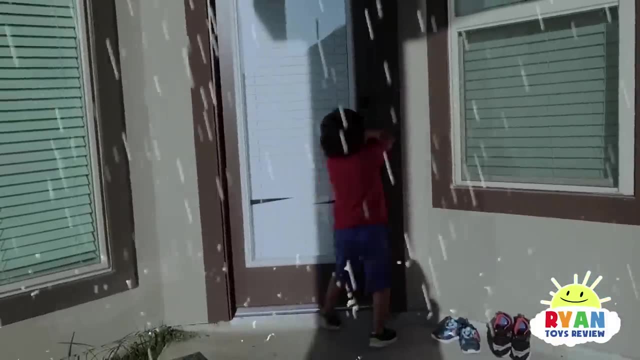 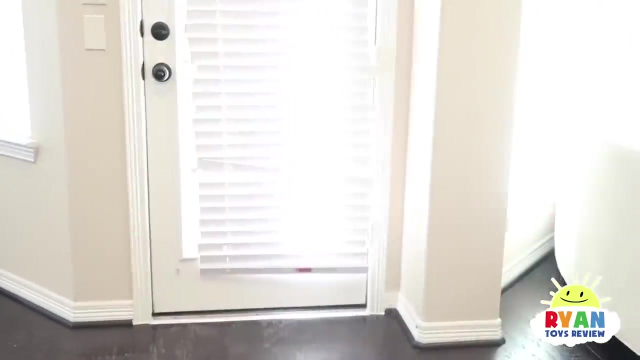 Ooh Ooh, I'm the boy you're waiting for. Ooh, Ooh, Wait, wait, wait, wait. Oh, Ah, Tornado. Yeah, Mommy, What happened? There's a tornado out there. 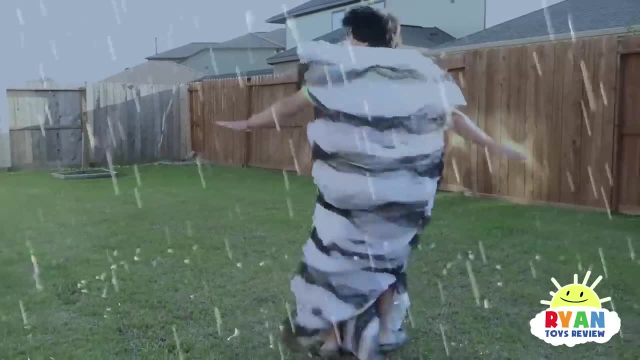 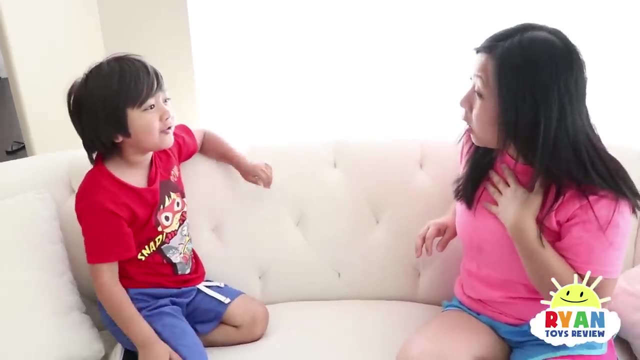 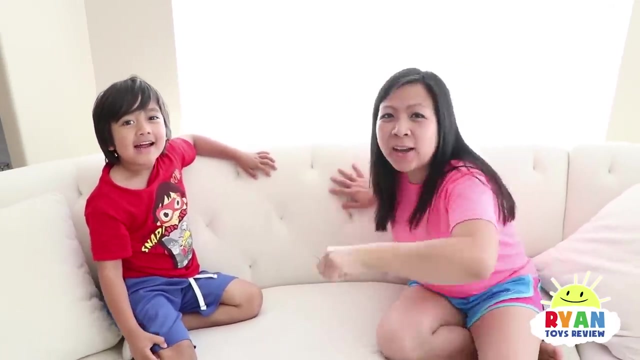 Tornado out there, Yeah, Whoa, You see. Oh, wow, Mommy, how do tornadoes form? Good question: How do tornadoes form? I'll be right back. Wow, Where did Mommy go? Ooh. 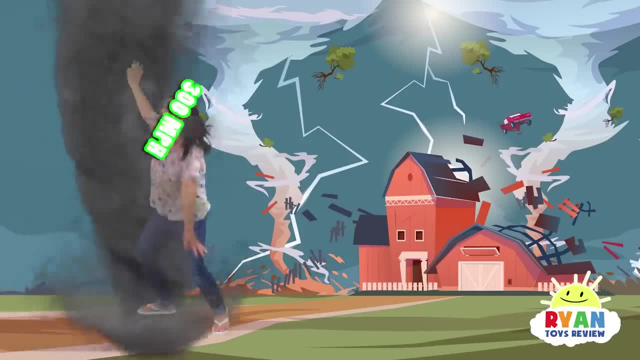 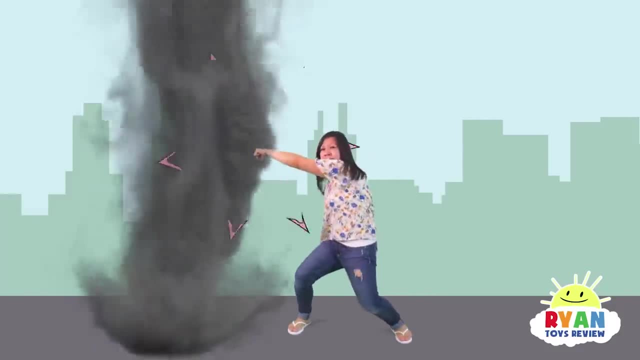 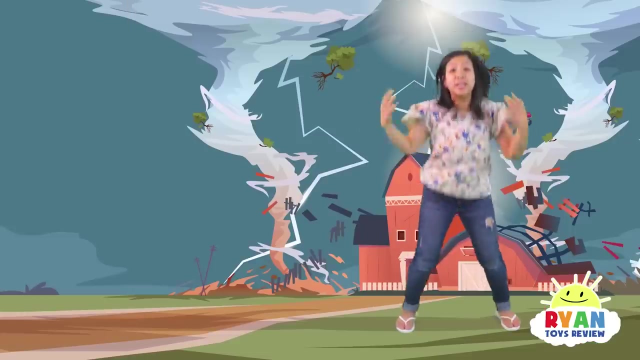 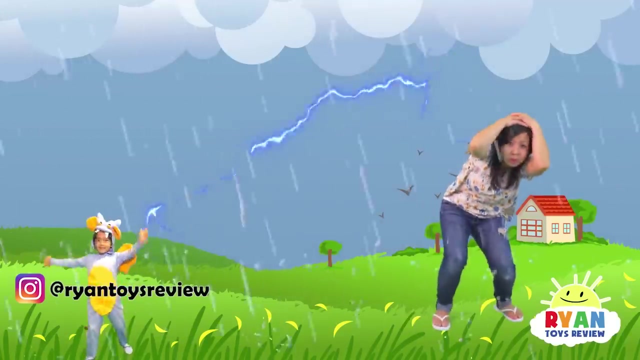 Hi guys, Did you know that a tornado can spin as fast as 300 miles per hour? Whoa? Also, a tornado can destroy buildings, power lines- whoa, look up there and uproot trees. Ah, A tornado is a rapidly rotating column of air that forms during the storm and connects 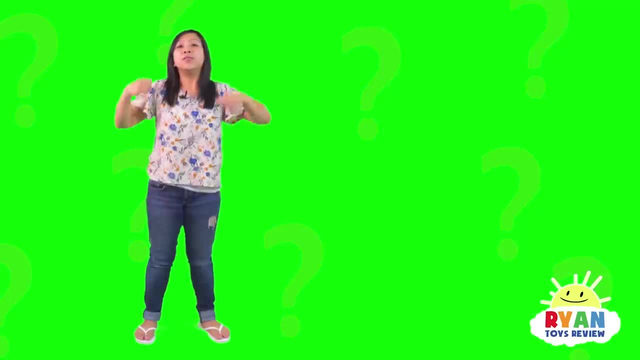 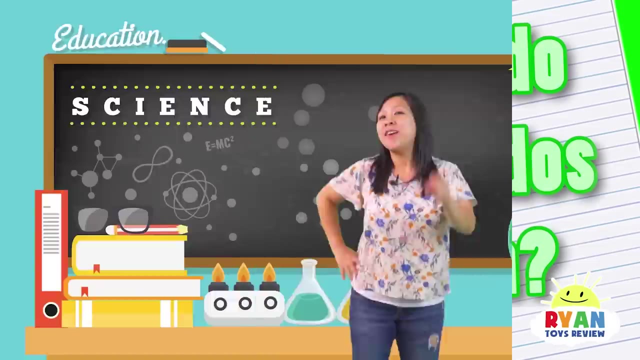 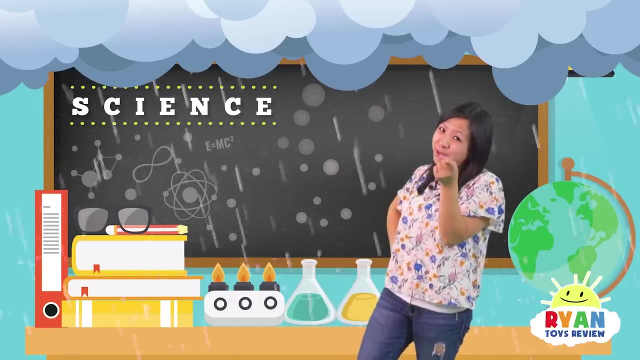 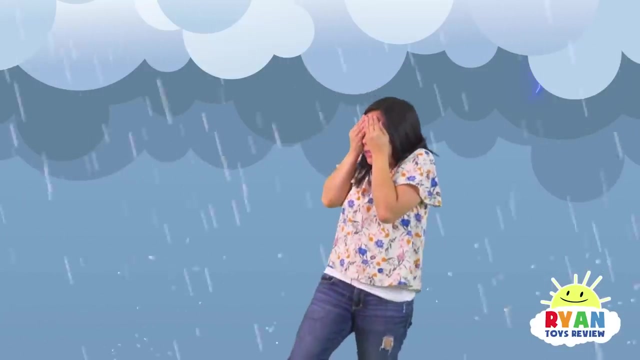 with the ground through a, Through a funnel cloud. So now that we know what a tornado is, we need to know why they form. First, we need a very, very special kind of storm. Can you guess what kind of storm? It's loud, strong and they can be scary. 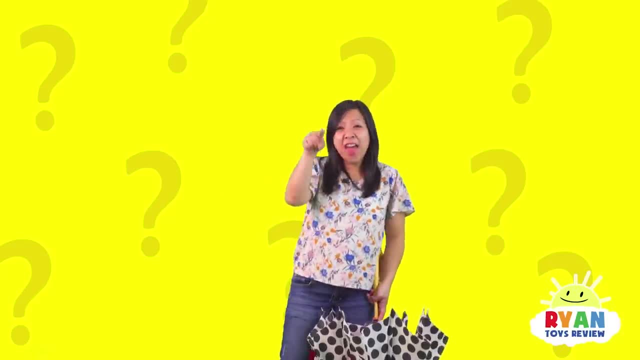 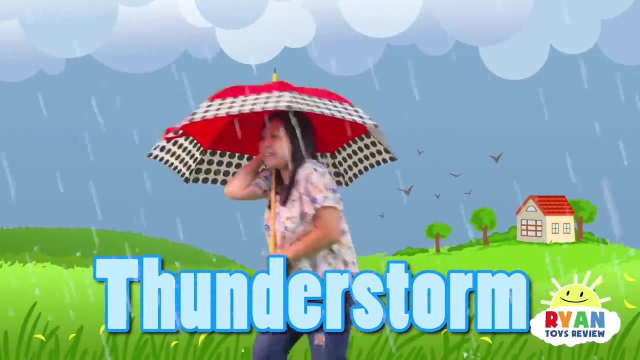 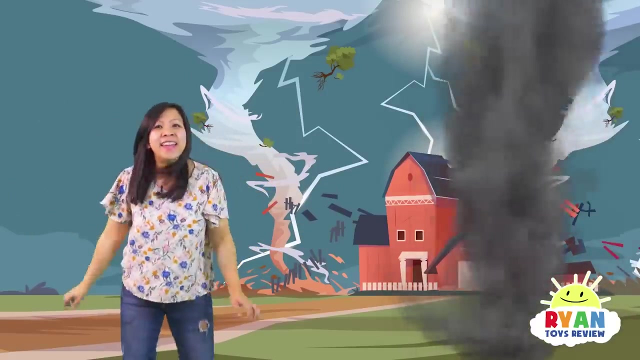 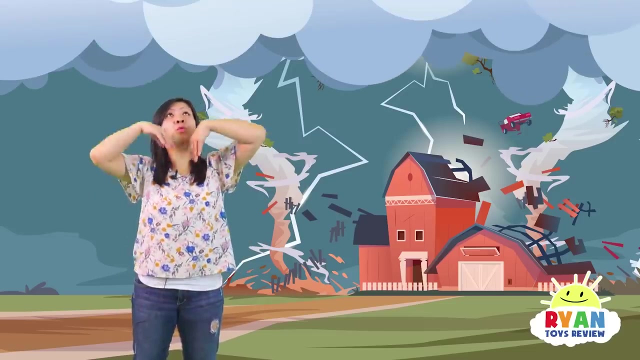 Did you guess what kind of storm That's right, A thunderstorm, Whoa. I'll be right back. But the kind of storm you need to produce a tornado, whoa, is called a supercell thunderstorm. That means it's a storm with rain, hail, lightning and fast wind. 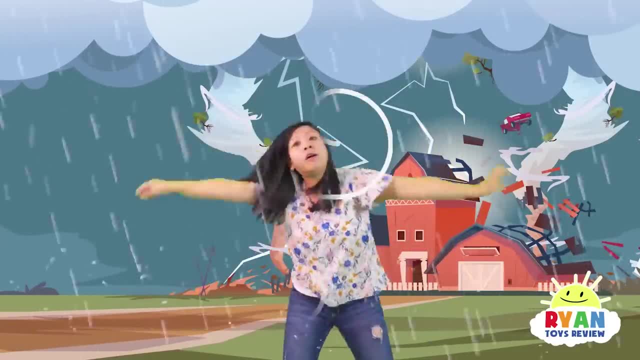 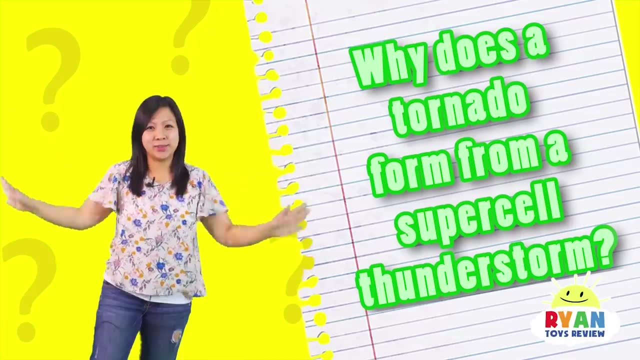 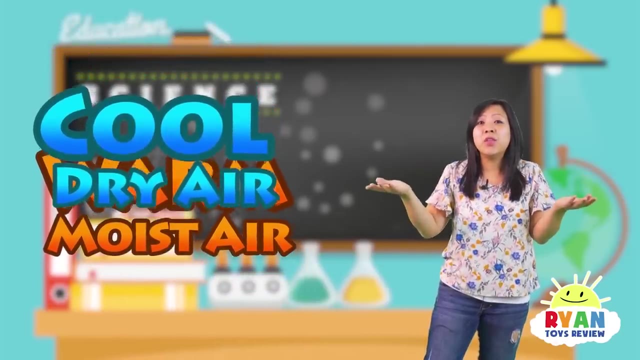 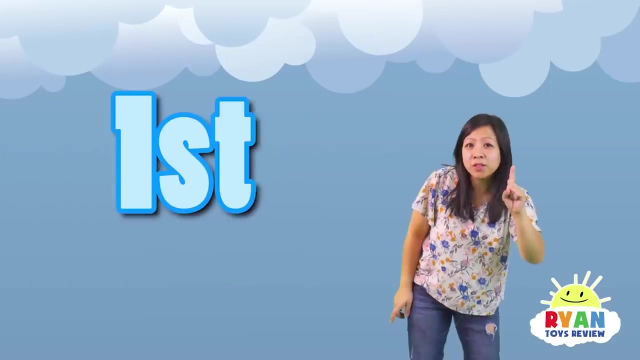 Whoa. Now why does a tornado form from a supercell thunderstorm? It's because warm, moist air meets cool, dry air and the wind's direction change. Now let's check it out. First, we have warm air rising. Ooh, Cool dry air. When the warm air rises, cool dry air sinks. It becomes a vortex or funnel, where the inside is warm but the outside is cold. It gets stronger and stronger and it spins faster and faster. 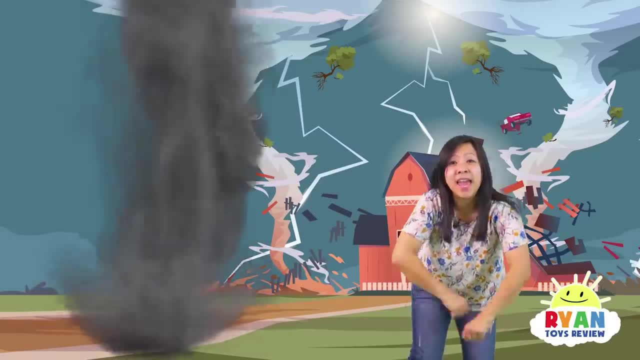 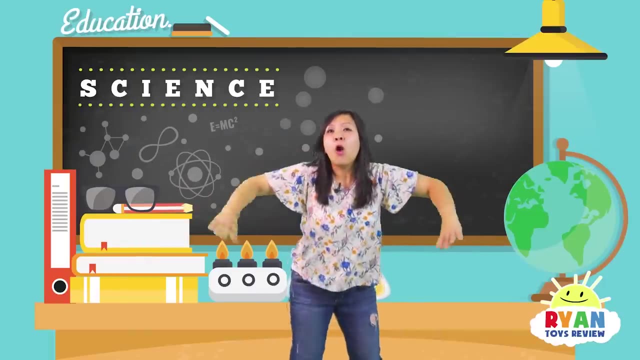 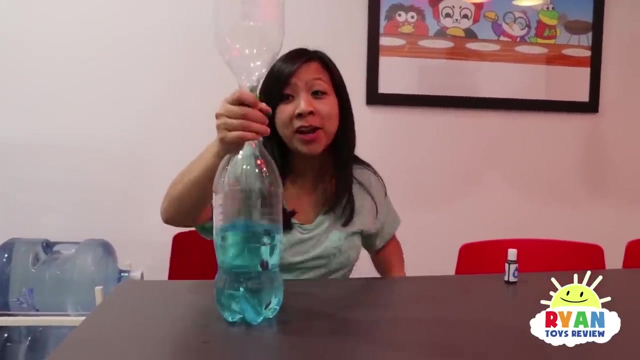 Finally, it touches the ground and it becomes a tornado. Here it is Hi. Now for the fun part. what about we make our own tornado? Are you guys ready to create our own tornado? Look at this. Whoa, so we colored the water blue. 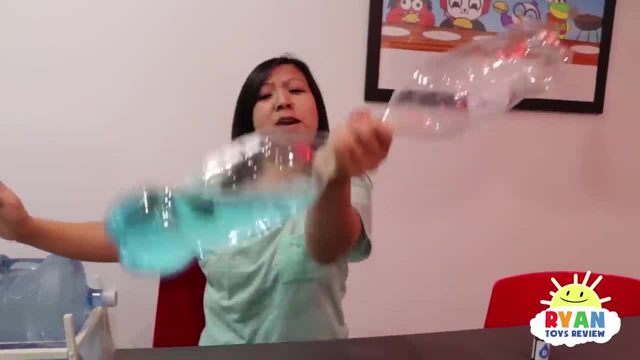 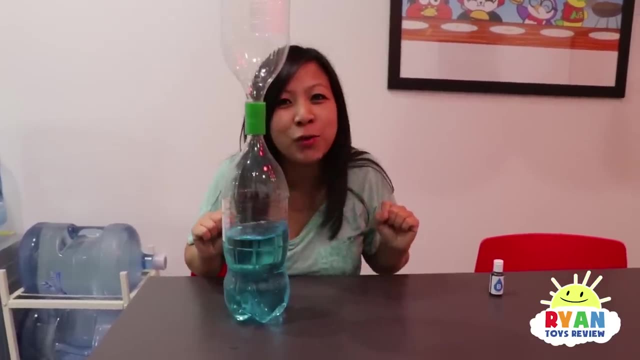 to make it more interesting. This is heavy. it's like ugh workout. Okay, on the count of three, we're gonna flip the bottle over to see if the tornado formed Ready. One, two, three, Yah. 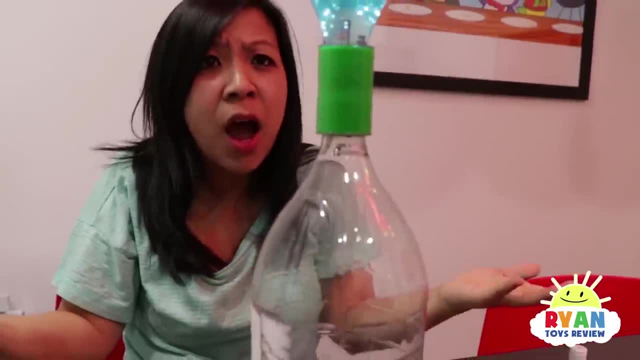 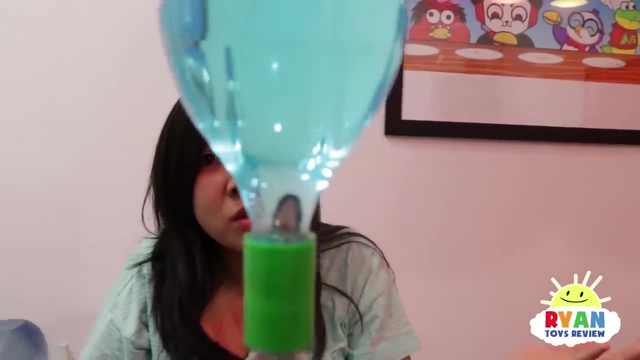 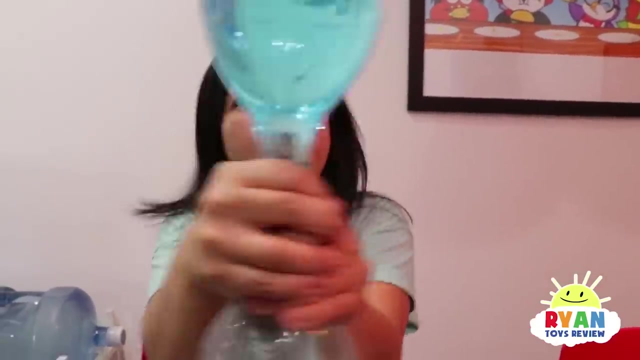 Oh, no, what do you guys notice? What happened? There's no tornado. Aw, do you guys know what we should do? What if we try to just swirl the water, like so, Whoa, Ooh, whoa. what do you guys see now? 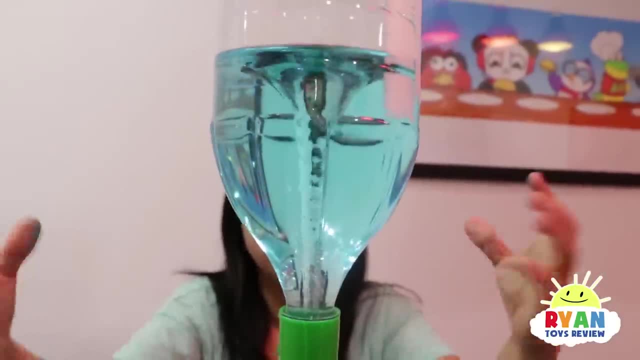 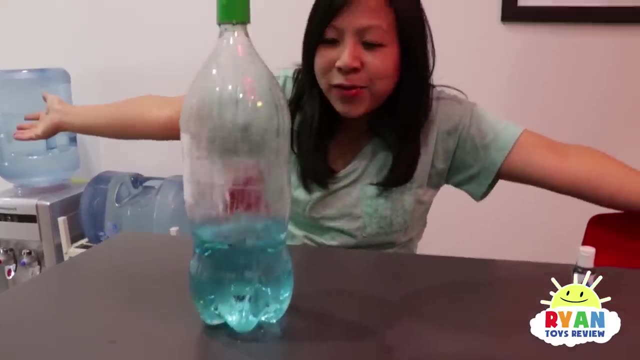 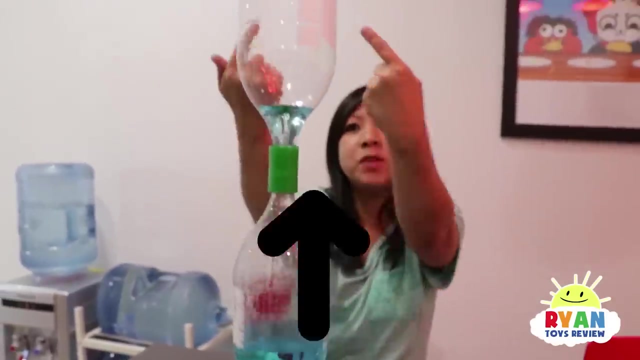 Do you see how, as the water begins to move, it creates energy and it makes it flow downwards. look at that Now. that's a real tornado. And as the water flows down, the air from the bottom bottle flows up to replace it. 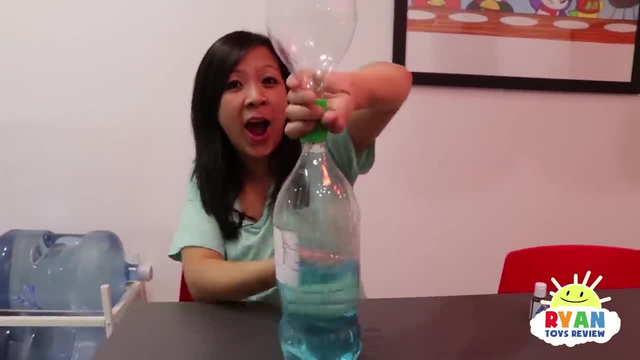 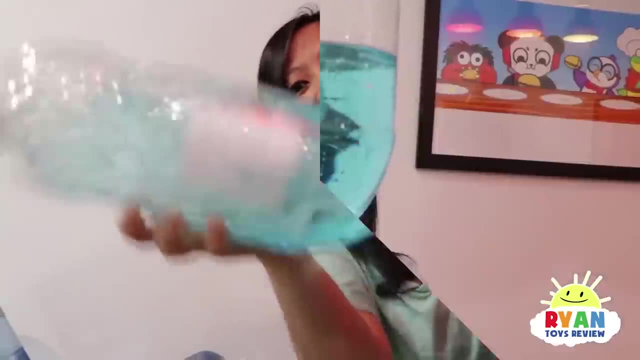 That was so much fun. You ready to see it again? Okay, so what do we have to do? We have to shake it, Whoa, the water's spilling out, but it's okay. Whew, Whoa, look at that tornado go. 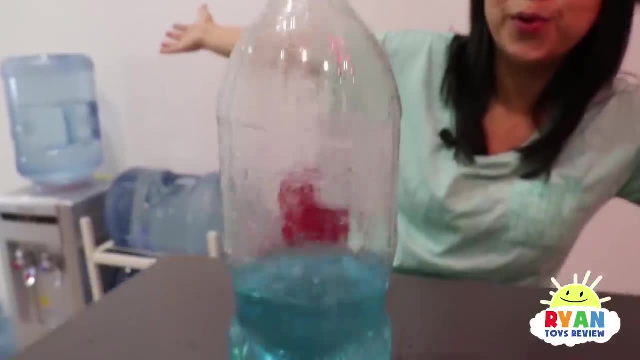 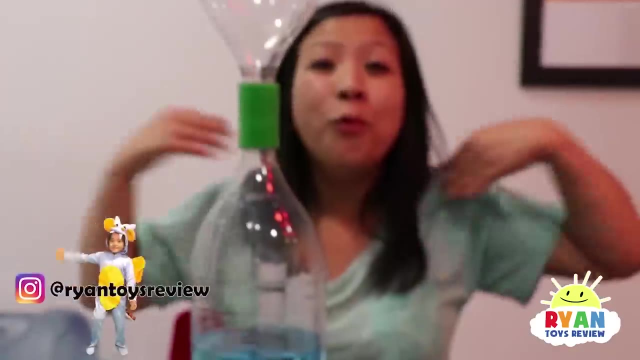 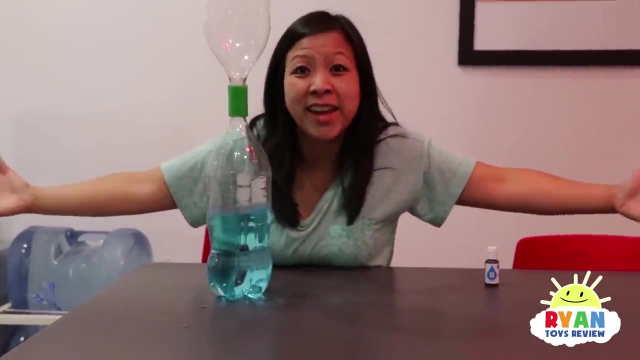 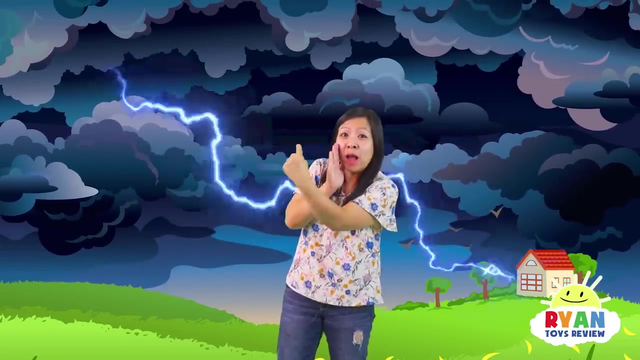 Whoo, Whoo, Hudson. Wow, That was so much fun making this awesome tornado, But now let's go and meet a real live tornado, Let's go. So now we're outside and there's a giant storm happening behind us. 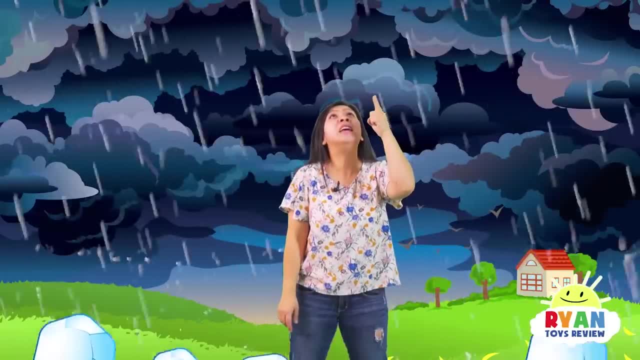 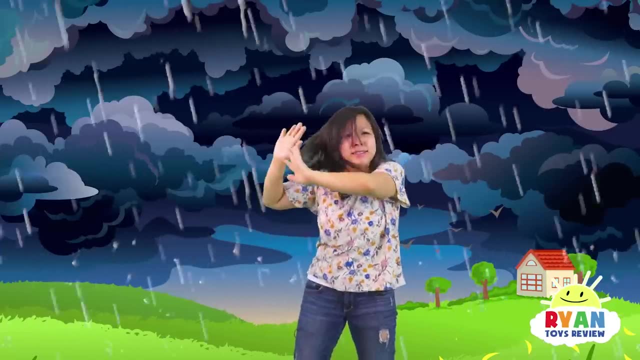 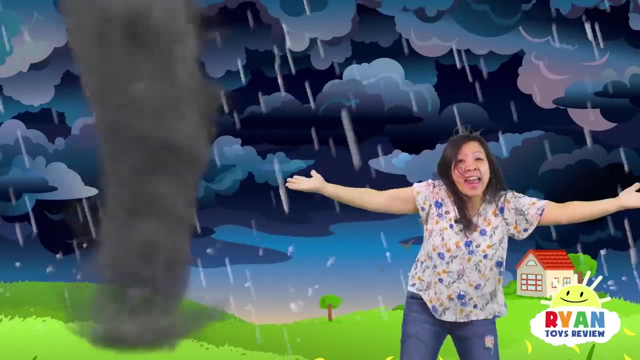 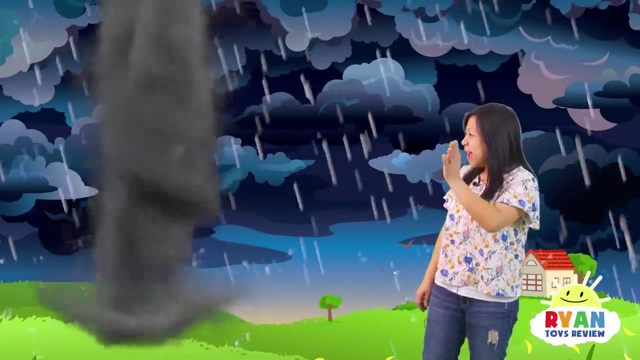 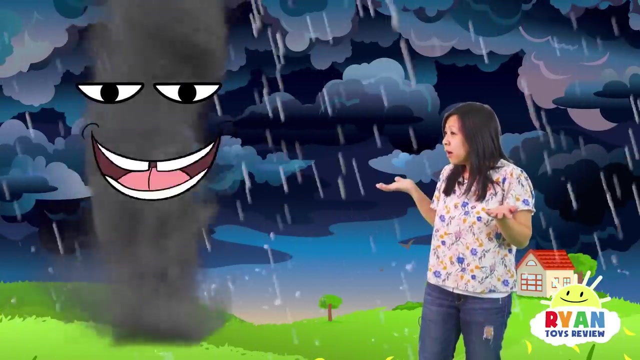 Do you guys see it? There's some big clouds here And it's getting. it's getting pretty windy. these are perfect condition for a a, a tornado. i wonder if it's a nice tornado. let's see. hi, mr tornado. well, howdy there. uh, wait, what are you doing out here? don't you know how dangerous tornadoes are? oh, i'm sorry. 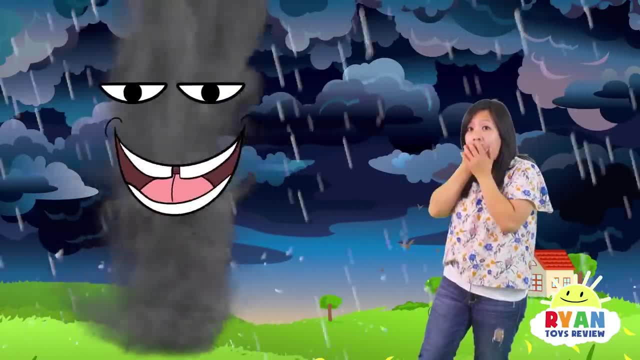 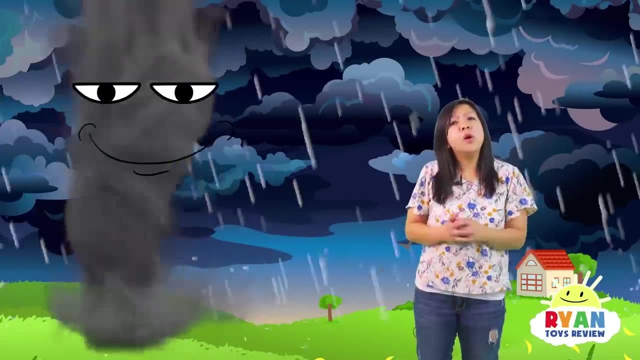 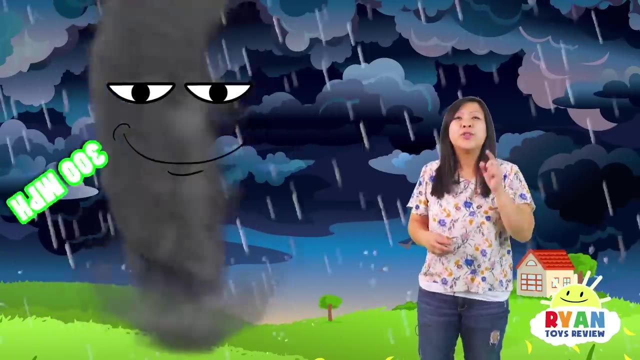 i didn't know. well, i'll warn you a little bit about us, but you have to promise to keep yourself safe if you ever see one of us again. all right, okay. so what makes tornado so dangerous? well, you see, we spin really fast, 300 miles per hour. right, you're absolutely right, some of us can spin that. 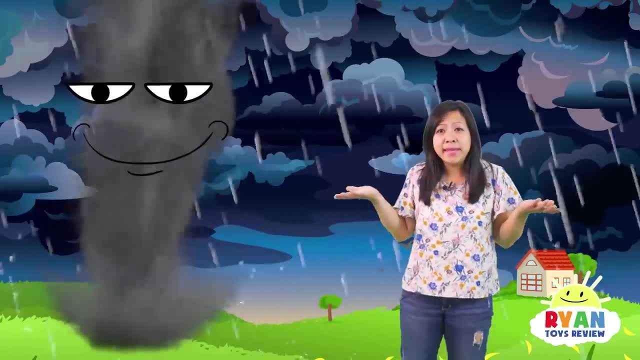 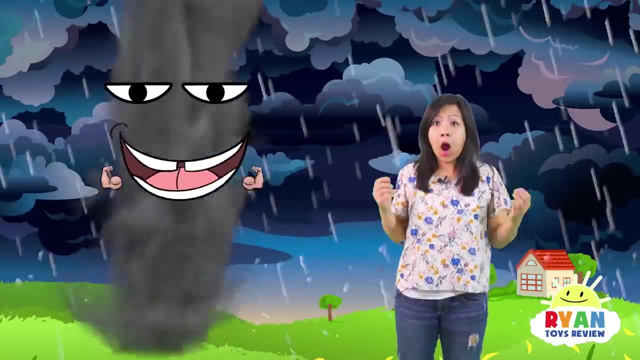 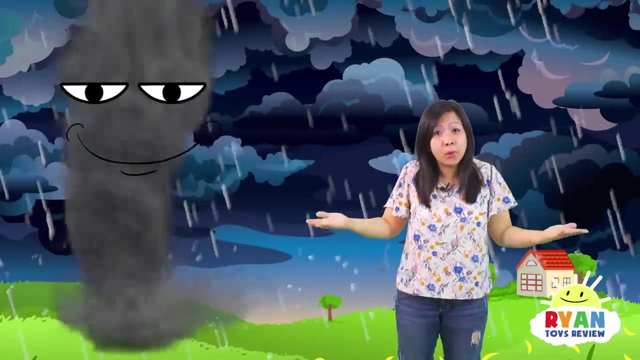 fast. we're also unpredictable too. so what does that mean? that means we can pop out of the storm anytime, at any place, and it can be a weak tornado or a strong one. you don't know. till you know, you know. so what are we supposed to do? if you have a basement, get to it. if you don't, 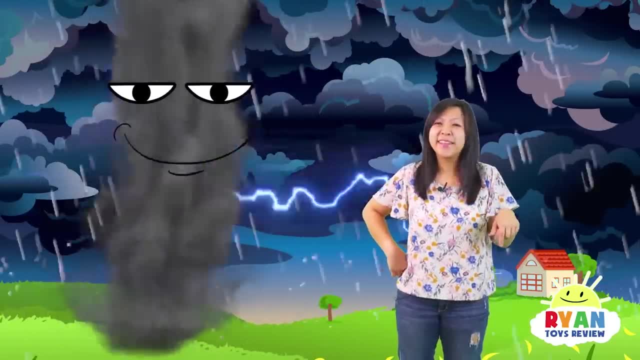 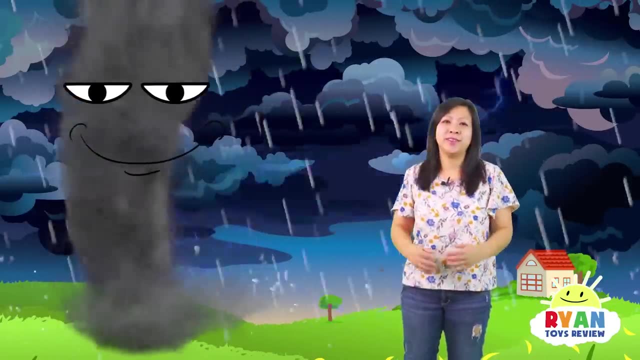 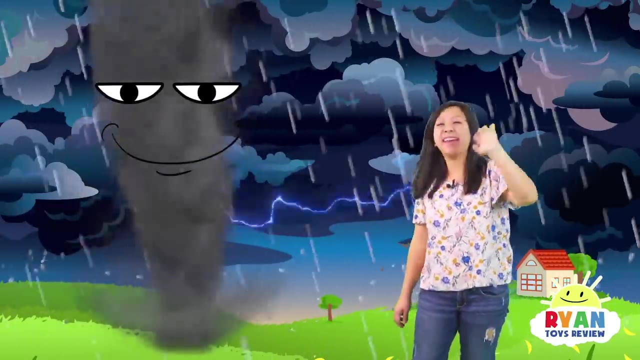 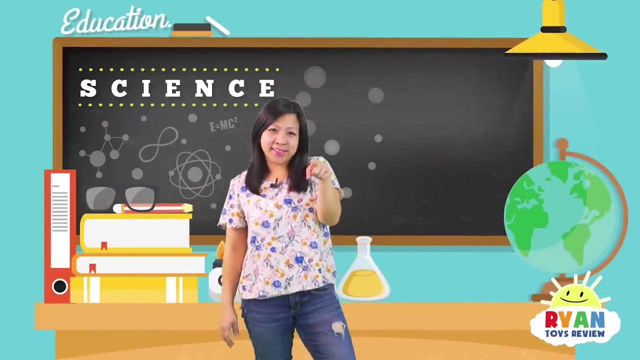 go to the lowest floor and find a safe place in your house that isn't close to windows, like a bathroom or a closet. that's some good advice. thank you, that's right. so get on and get safe, okay, thank you so much, mr tornado bye. so now that we know so much about tornado, let's take a quiz question. 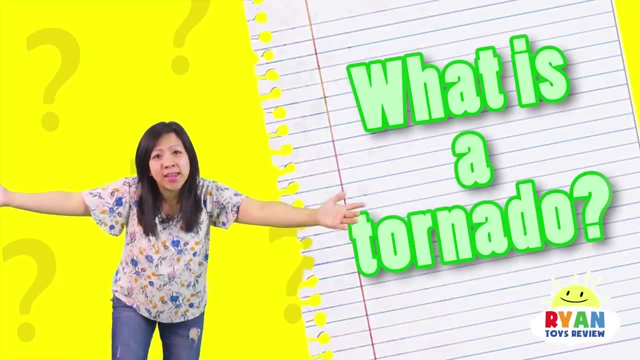 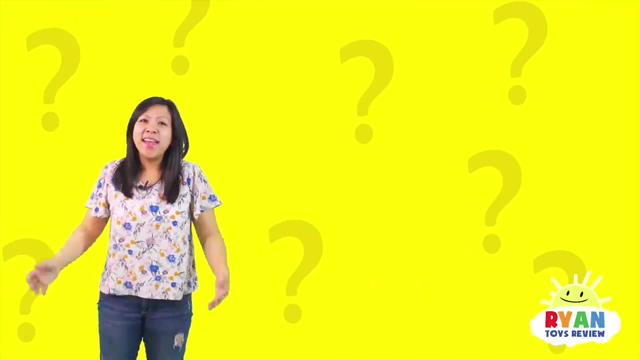 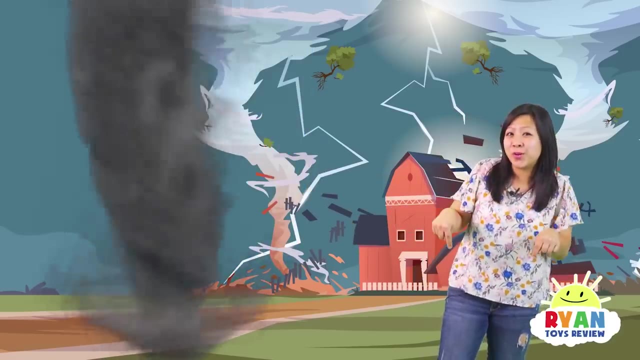 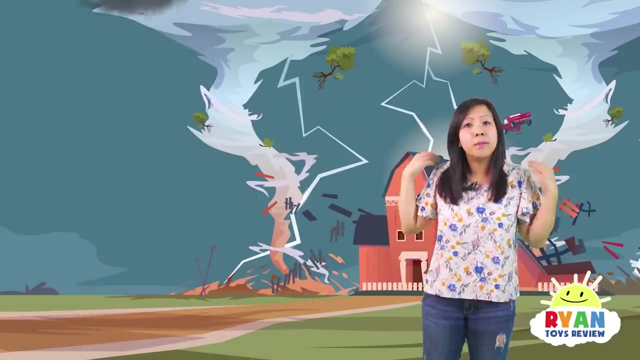 number one. what is our tornado? is it a hurricane? is it your best friend? or is it rapidly rotating columns of air that connect a thunderstorm to the ground? that's right. a tornado is a rapidly rotating column of air that connects a thunderstorm to the ground. next question: why do tornadoes form? is it because warm, moist air meets cool, dry air and wind direction changes? is it because they are late for dinner? or is it because they are looking for their money? that's right. a tornado forms because warm, moist air meets cool, dry air and the wind direction changes. 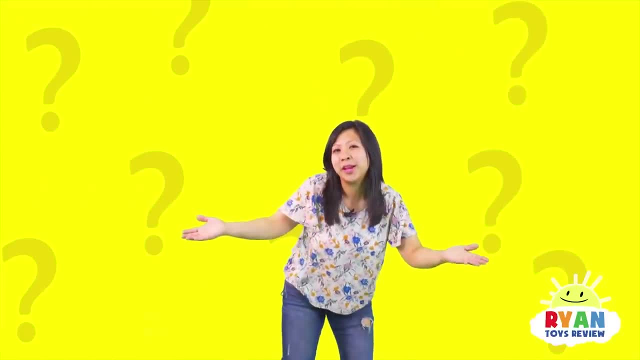 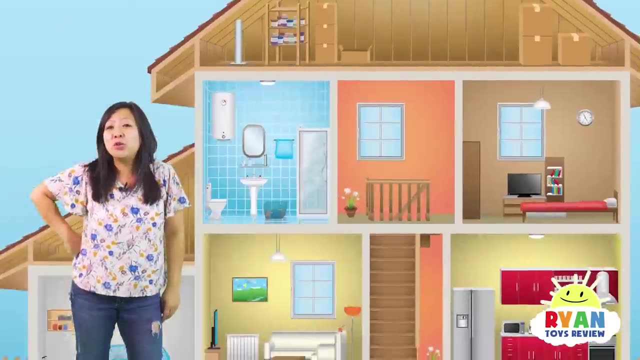 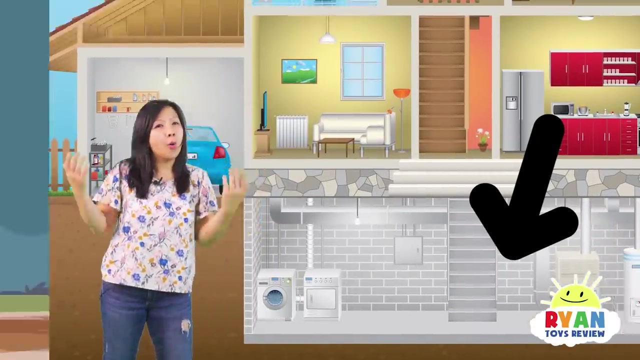 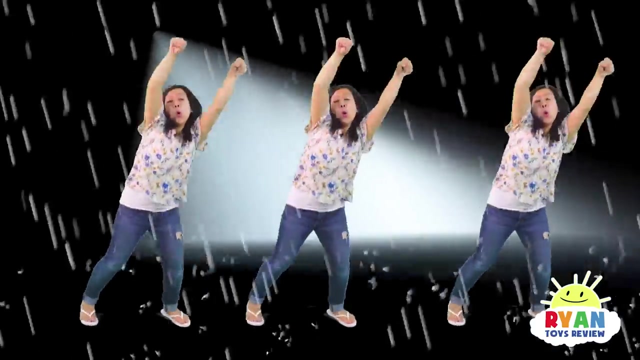 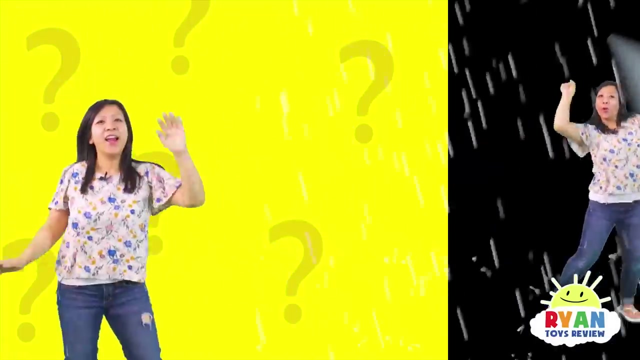 question three: what should you do to stay safe from a tornado? is it let's go to the basement or safe room on the lifts- maybe a newspaper or a book or a book lowest level with no windows? or should we dance in the rain? or, if there's a tornado, should you just eat some yummy candy and watch YouTube? 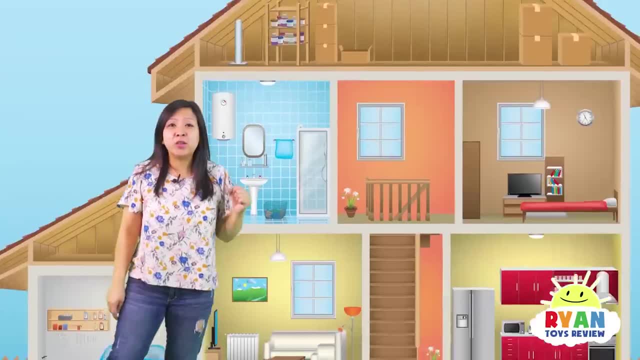 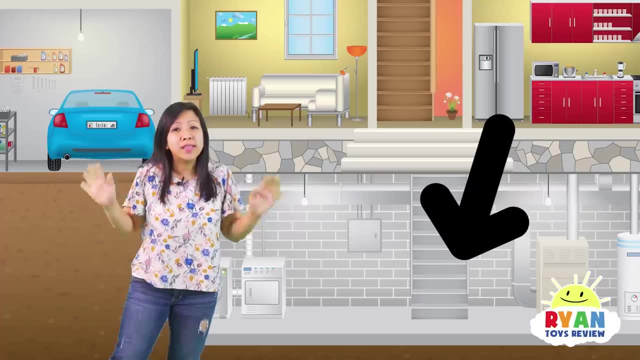 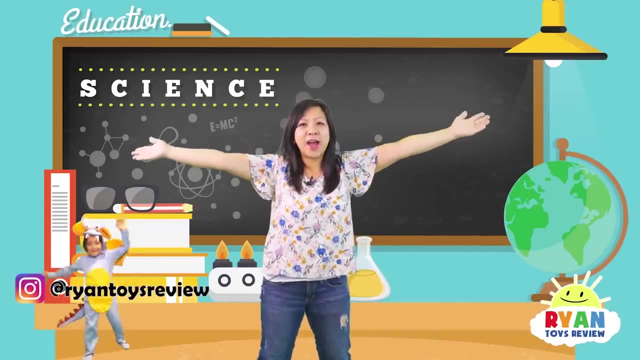 videos. that's right. if you see your tornado, the best way to stay safe is to go to the basement or a safe room on the lowest level where there is no window. great job, now that we learned so much about tornado, let's go back and tell Ryan. okay, let's go whoa. 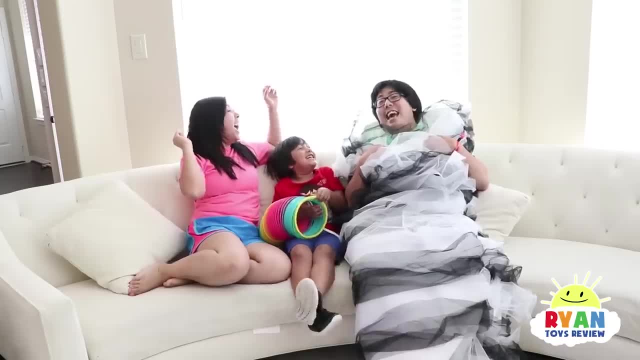 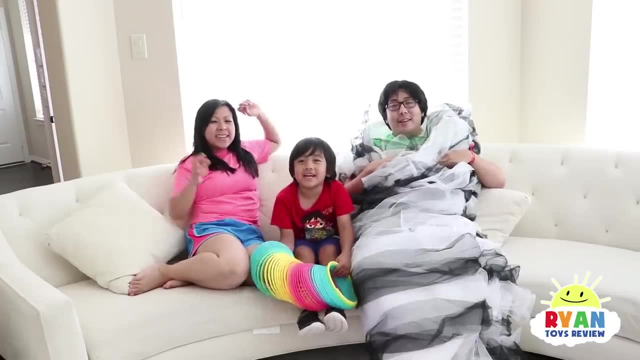 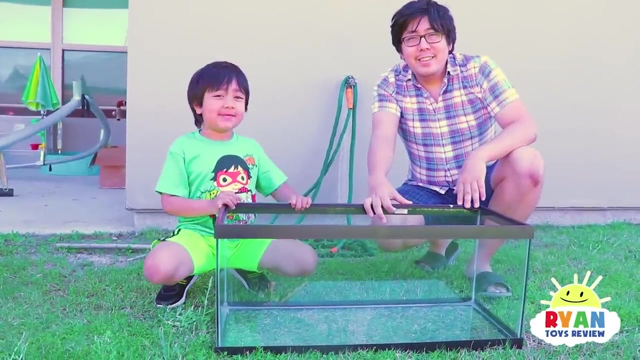 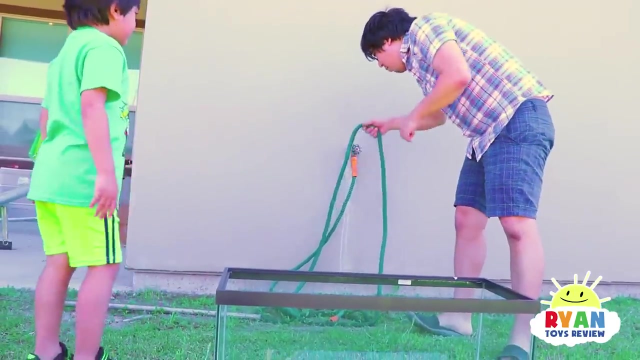 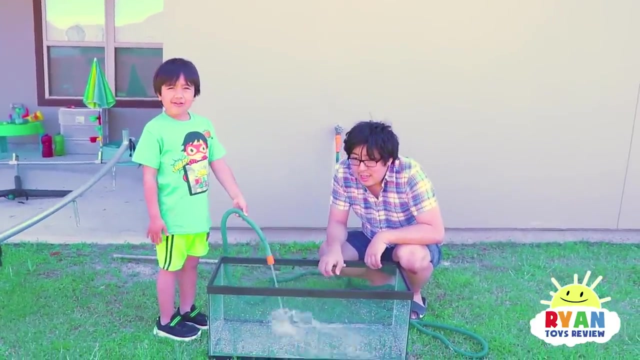 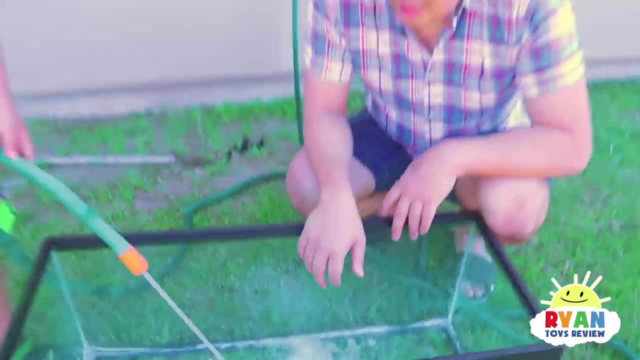 yeah, we're going to test out all the object around the house and see if it floats or sink. so, Ryan, do you know how an object sink or float? no, if the object is less dense than water, because that's what the liquid we're using. if the object is less dense than water, then it will float, and if it's? 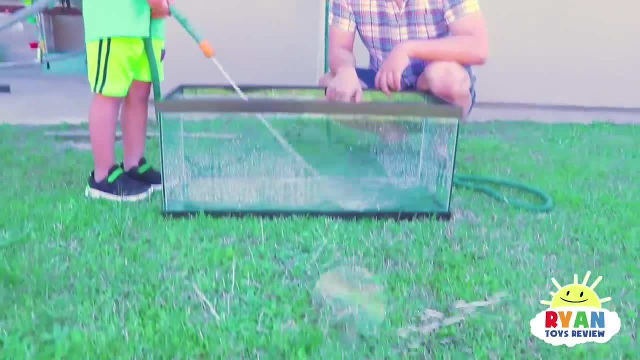 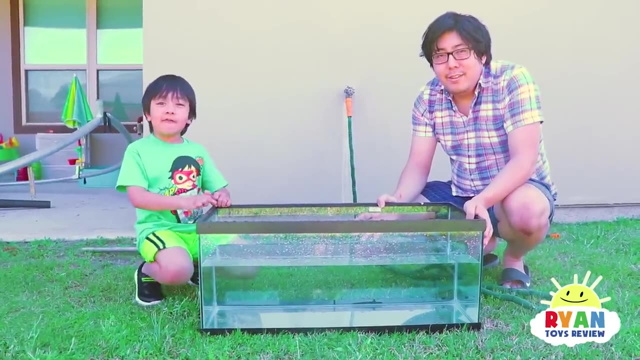 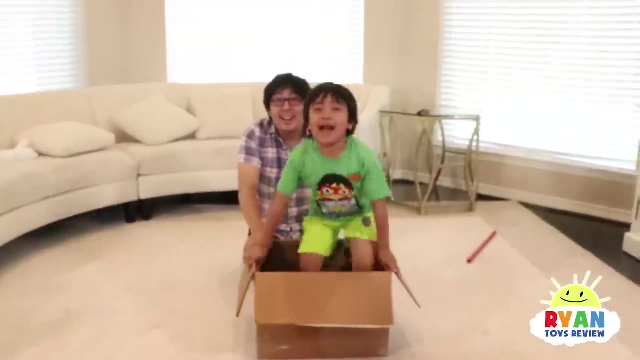 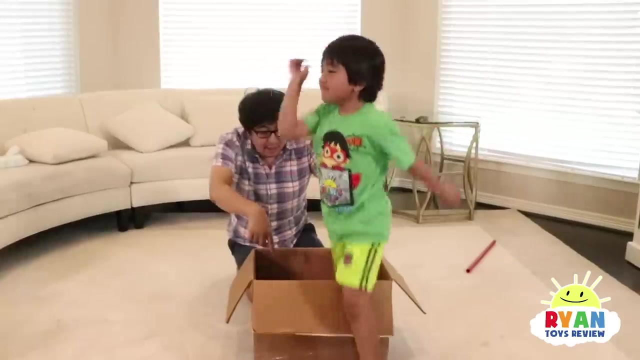 more dense than it will sink. yeah, now that the water's filled up, let's go find some objects. all right, let's go inside and find it now. we're going to look around the house to find some objects so we can see if they sink or float. let's find an item and put it in this bottle. 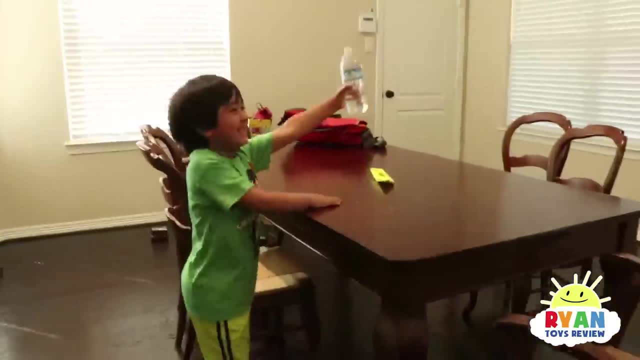 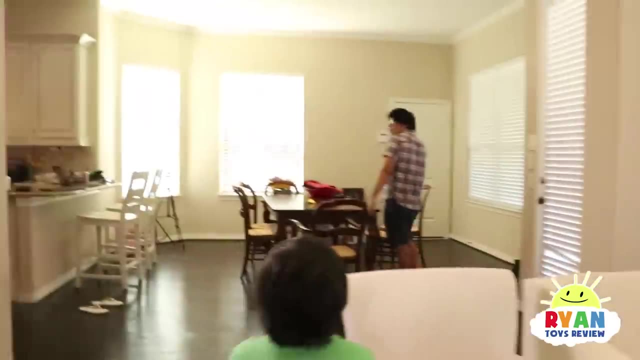 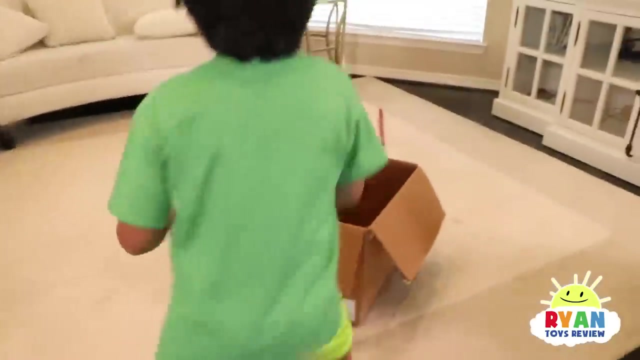 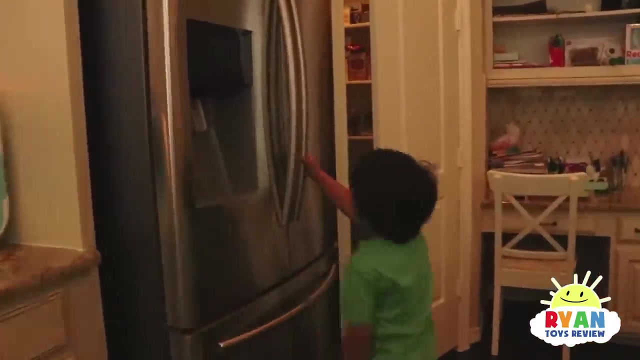 what should we use? we want to see if a water bottle will sink or float. okay, you think a boat's gonna sink or float, float, float. okay, guys, we'll find out. what else? what else you guys? so Ryan wants to get the diet coke in the fridge. 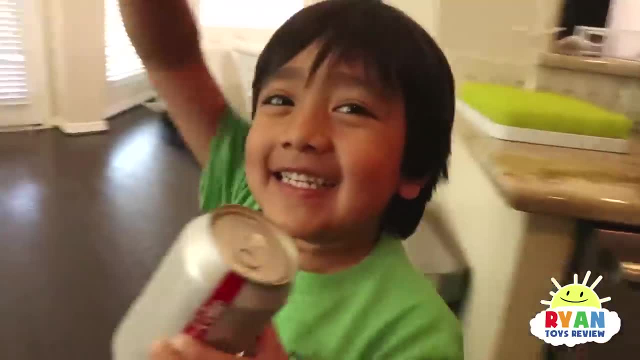 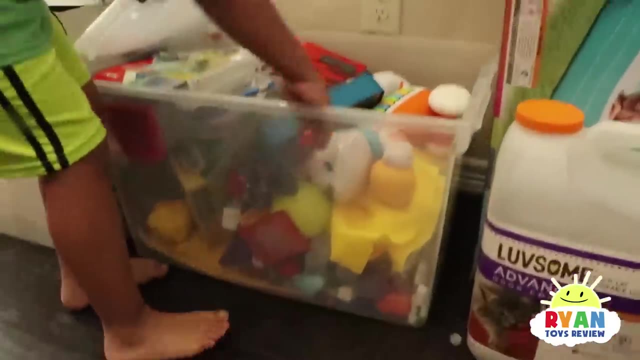 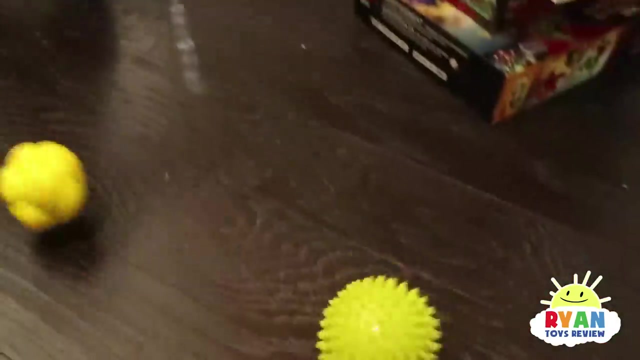 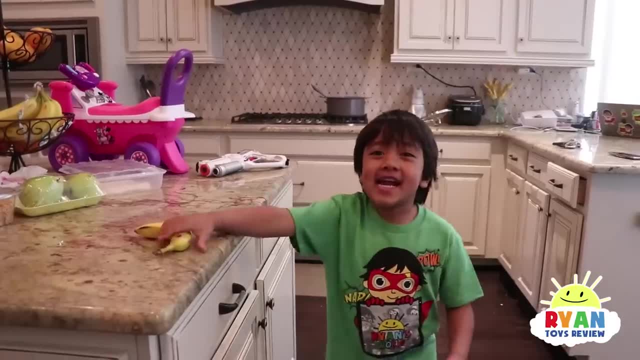 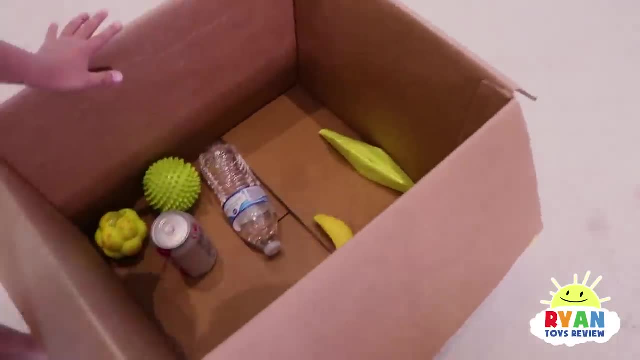 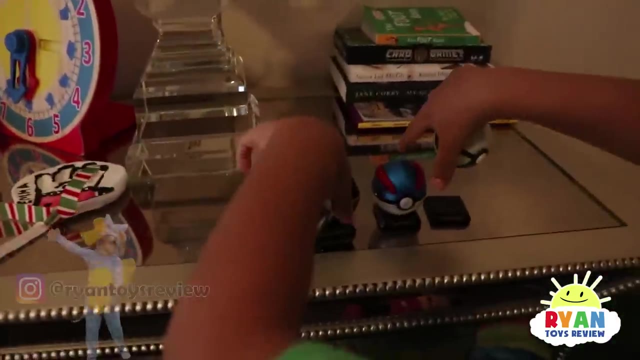 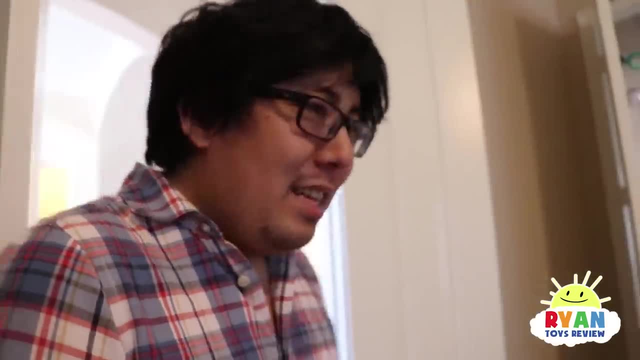 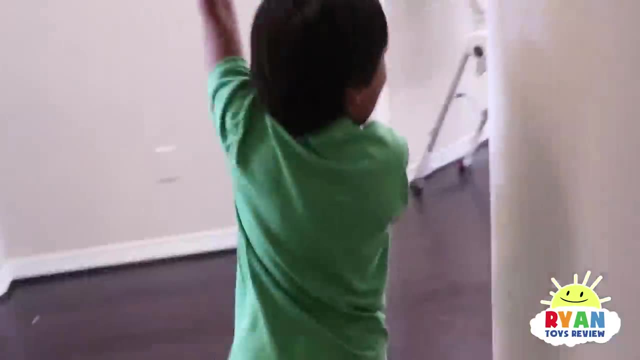 whoa, don't put that in the water. you think they're gonna sink or float? daddy, I think it's gonna float, float, but don't test it sink. Let's go upstairs to look for more toys. A bunch of hot wheels. We have a yellow car. 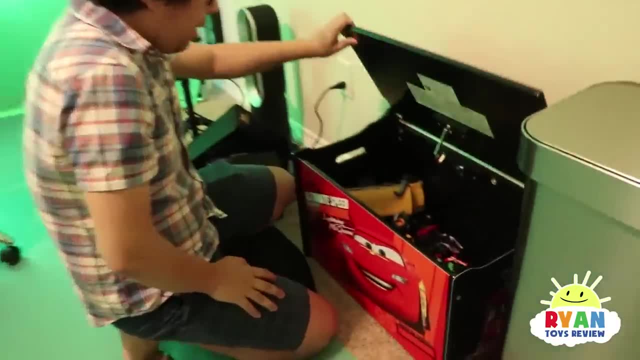 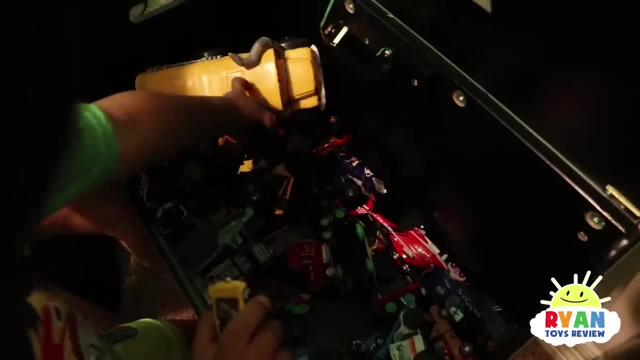 You want to test that one? Uh-huh, Okay, what else should we test? All right, what about some Disney cars, Ryan? which one do you want to bring in? Which one to take? Whoa, That's a big one. 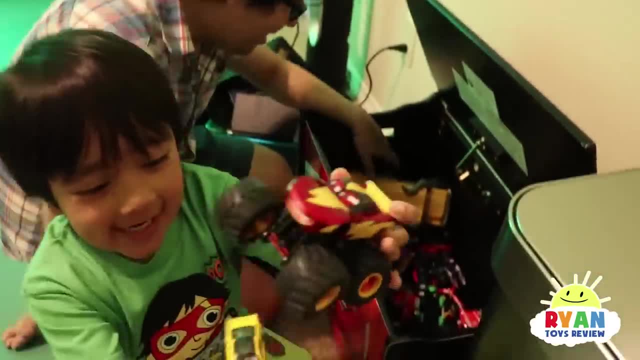 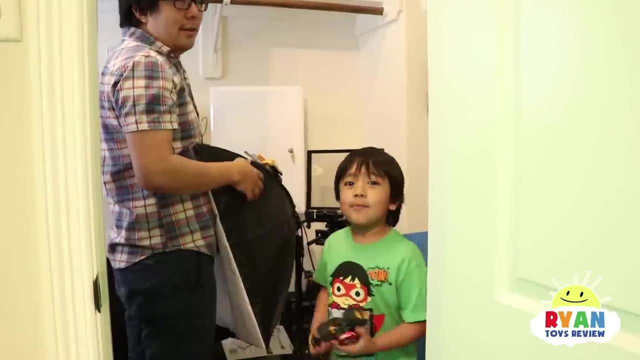 It's a McQueen. Oh, what about this? This is a big bus. Do you think it's going to float or sink? No, All right, let's try this one too. What about the pumpkin up there? Oh, this is a cute pumpkin. 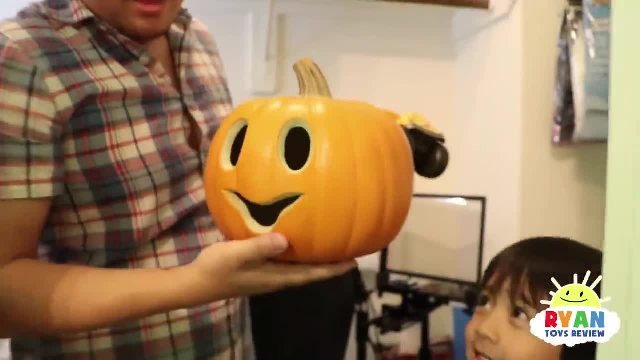 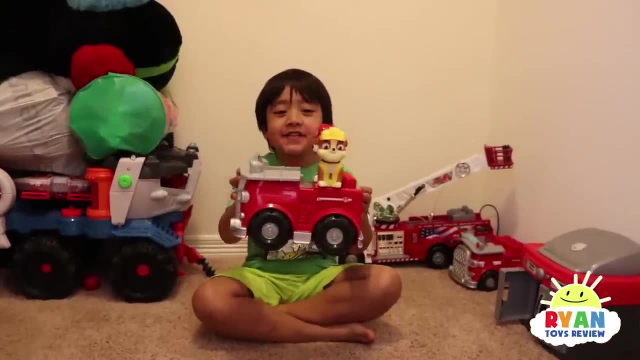 It's smiling. Let's get this. Are you going to sink or float, Mr Pumpkin Head? I'm going to float. So what else are we testing out Blue bats? Now let's test out this fire truck with Marshall and Rubble in it. 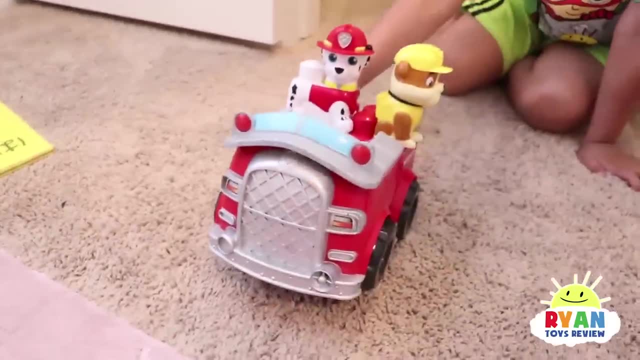 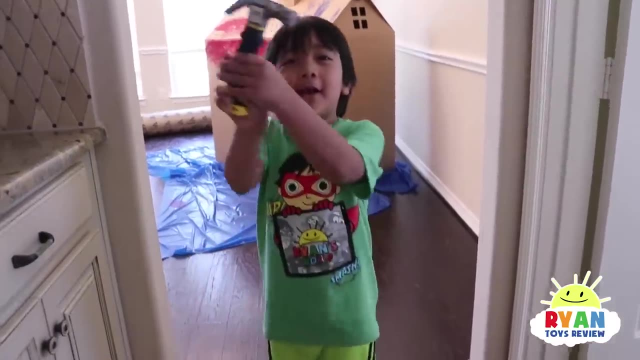 Hi, Are you guys going to sink or float? We're going to sink. We have so many things. What about we test this? Hey, there, We're going to see if it sinks or floats. What do you think Sinks? 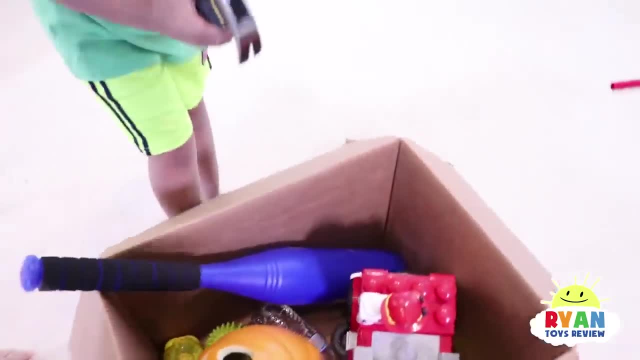 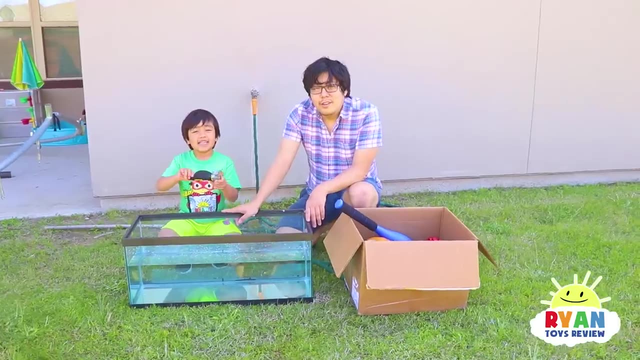 All right, I think we have enough object here, So we're going to bring it outside to see if it sink or float. Here we are, Bounce up, Let's test out the hammer. All right, Do you guys think it's going to sink or float? 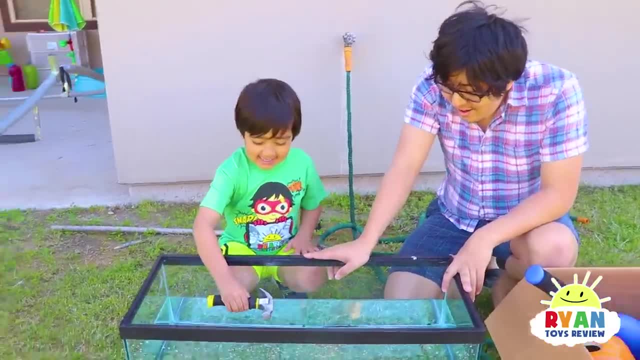 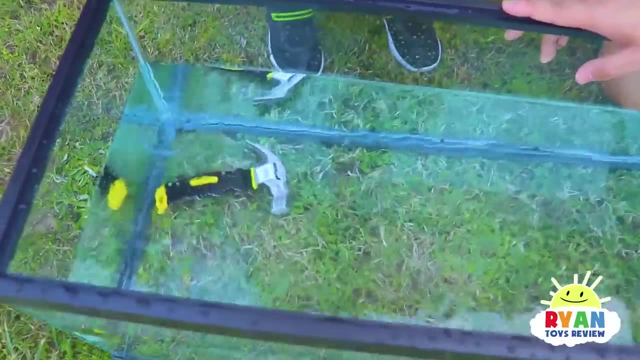 Do you think it's more Sink? Sink, OK. Do you think it's more dense or less dense than water? More dense, More dense, More dense. See, Oh yeah, For sure It's sink. So it is more dense than liquid water. 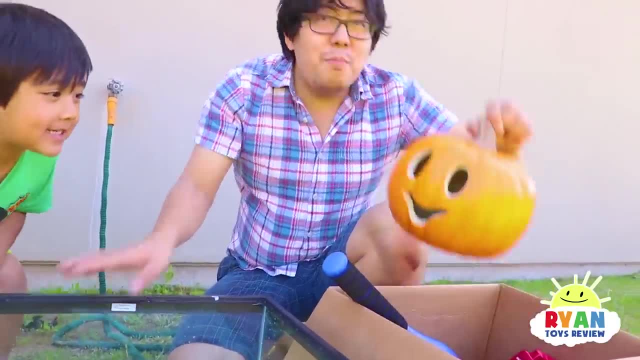 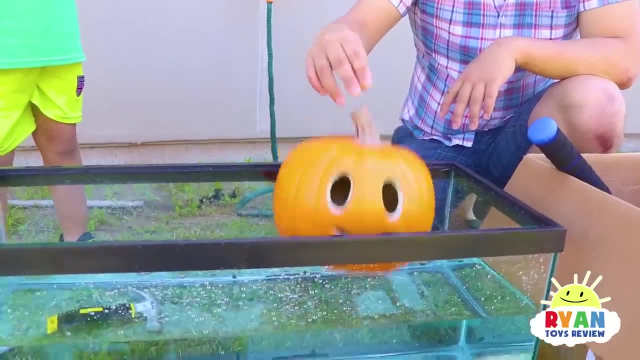 What do you want to try next, Daddy? I will try this cute pumpkin. Aw, What do you think, Ryan? Let's dance, Let's dance. So it's going to float. Yes, Is it going to float? Is it going to float? 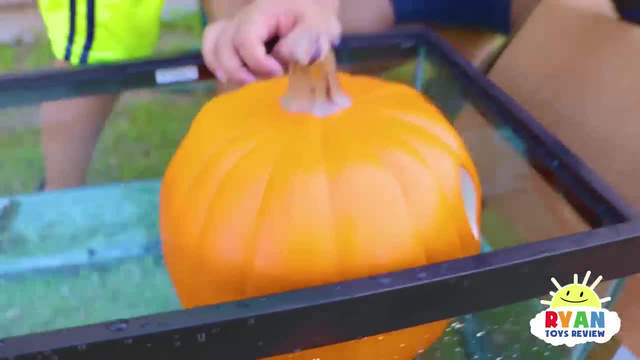 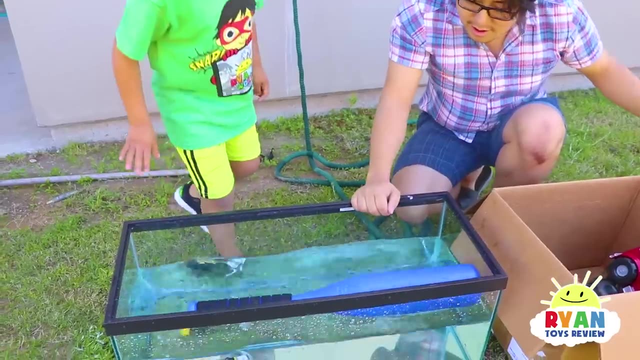 Ah, pumpkin float. It's so cute. I'm going to try this. A bat, A bat Say sink or float, Sink, Sink, Float it. Ah, It floats, It floats. How is it less? It's less dense. 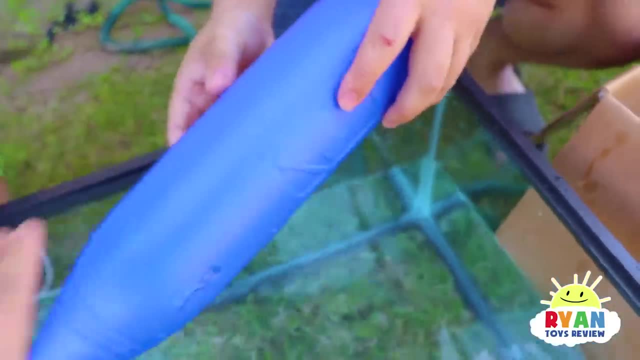 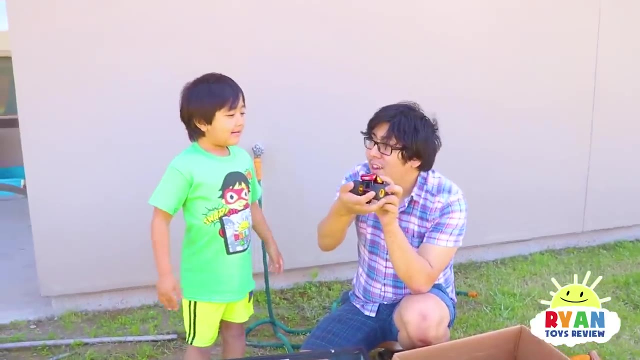 Again, it's probably because it's hollow inside. Yeah, there's nothing inside, Ryan, It's air. Yeah, so there's air. Air is actually less dense than water, so it helps it float. How about McQueen monster truck? 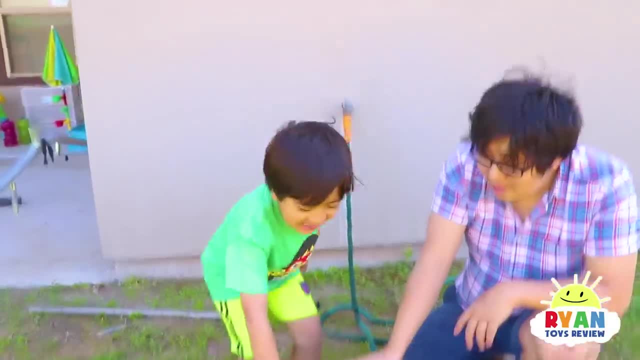 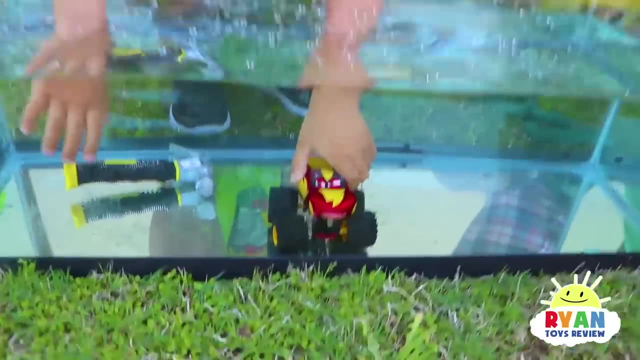 Monster truck McQueen, Sink or float, Sink, Sink, Sink, Sink. More dense than water, More, More dense. Oh you're right, More dense. Hi McQueen, How do you feel being in water? Are you ready to go for a swim? 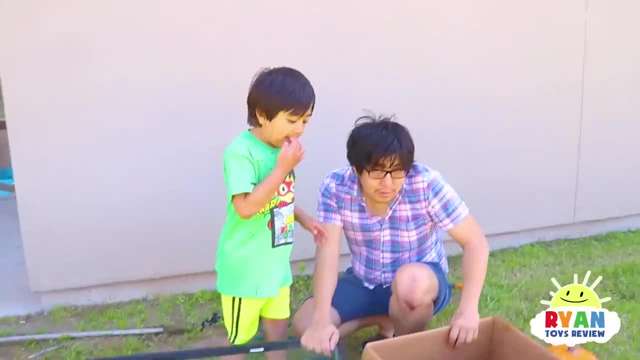 Choo-choo, Choo-choo, Choo-choo, Choo-choo, Choo-choo, Choo-choo, Choo-choo. What object do you want to test next? 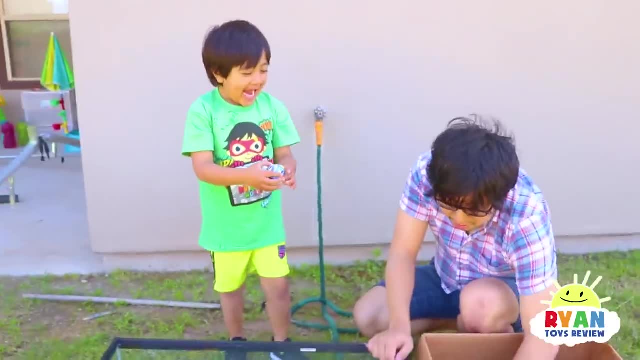 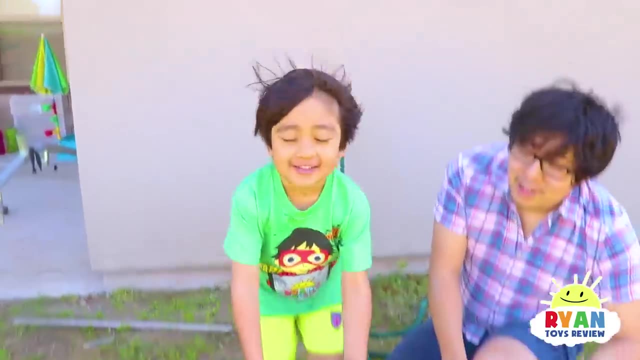 What's next? No, No, My Pokeballs Pokemon Sink or float, Float, Float, Float, Float, Float. It's going to float- OK, I think, because it's hollow. Is there a Pokemon inside My Pokeballs? 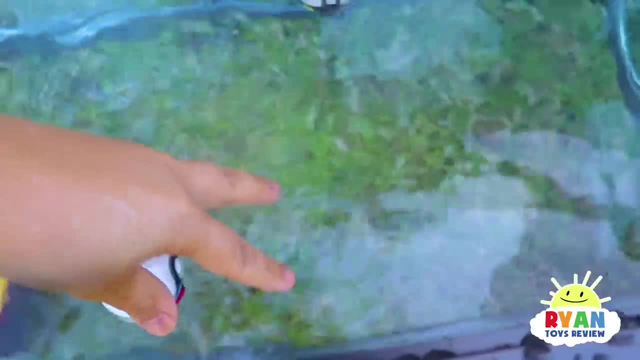 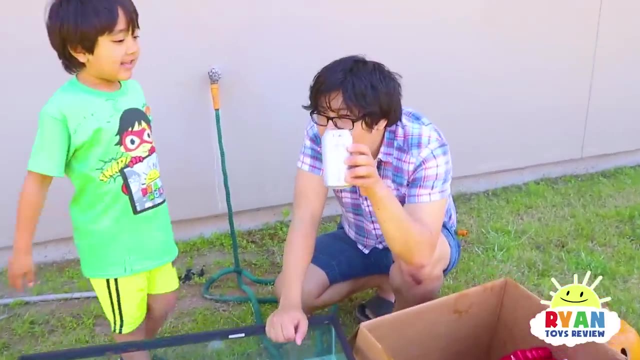 No, It floats. Look at that, Woo Woo. Even if you put it down, it pops back up. Oh, it's my turn. Yeah, I'll pick my favorite drink: Diet Coke. Oh, Diet Coke, Sink or float. 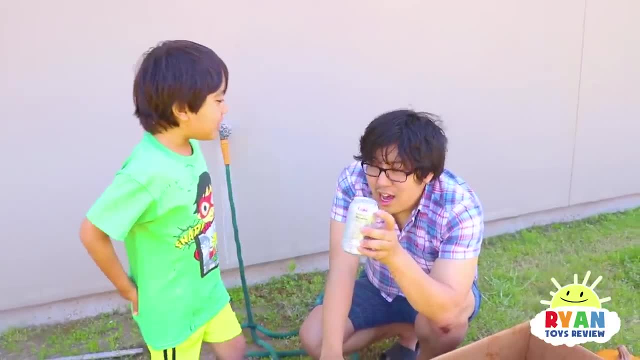 Sink Sink? I don't think it sinks. Wait, Is there anything in there? Yeah, Diet Coke, It's going to open. Sink Sink, Sink, Sink Sink. I think so too. Let's see What's your guess, Mommy. 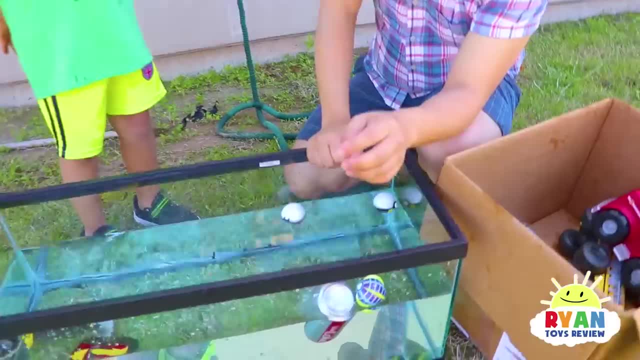 I think it's going to float. It's going to float, Yeah, Why? What did you say Go? Oh, it floats. It floats How I knew it? Because Diet Coke doesn't have the. it has the fake sugar in there. 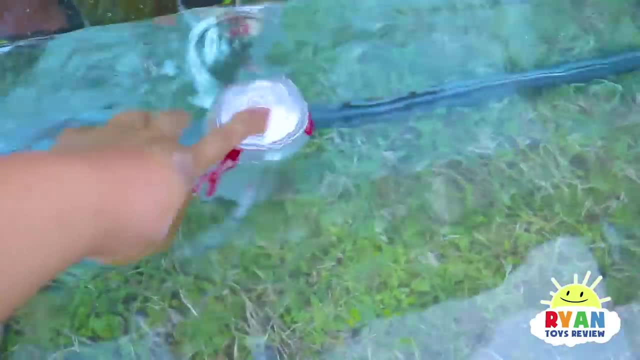 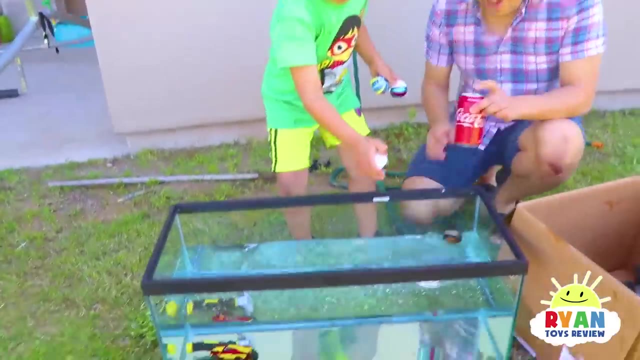 It doesn't have sugar in there to weigh it down. Daddy's going to see if he can find a regular soda that's not diet and see what happens. Daddy found the regular soda. All right, Let's see. So because it has sugar in there, it's going to make it more dense than water. 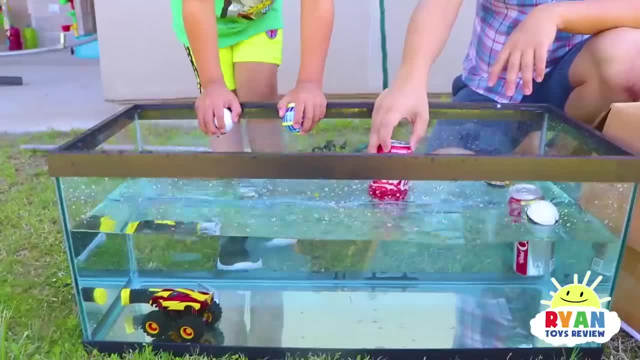 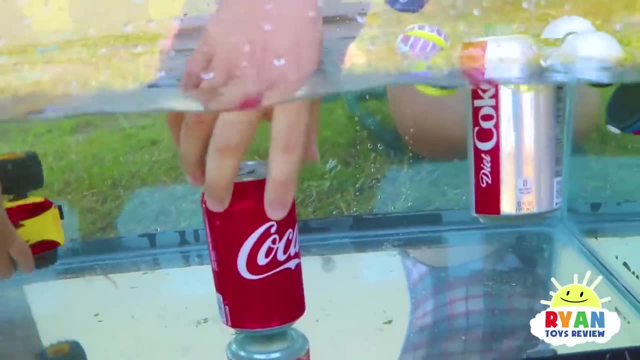 Let's see if it's true. You guys ready, I'm ready. Sink- It is going down more, Maybe it just takes time. Regular soda sinks- It just takes time. Yeah, Woo, I want the banana, Banana sink or float. 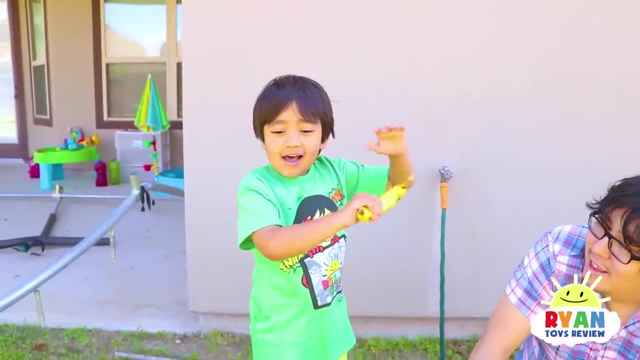 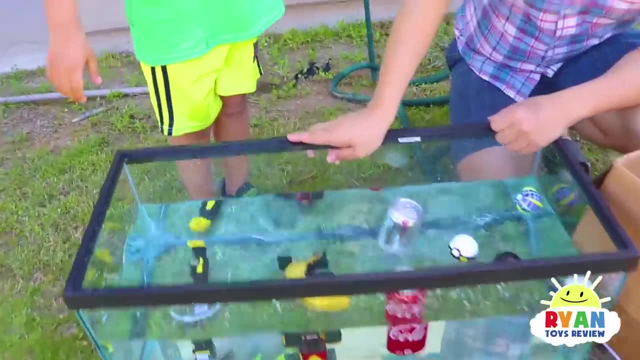 I think it floats More dense or less dense than water. Less dense, Less dense. You guys both think it's going to float. Yeah, Come on Really. Ah, float What? I didn't know that Banana is less dense than water. 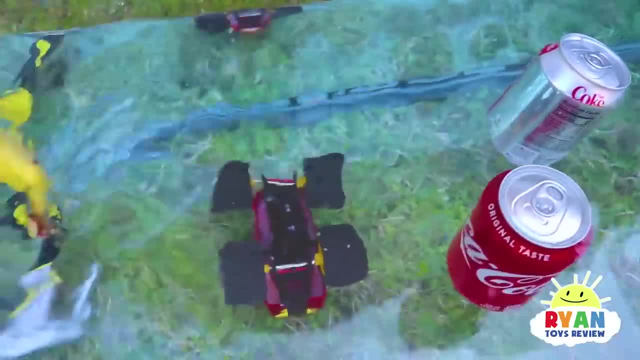 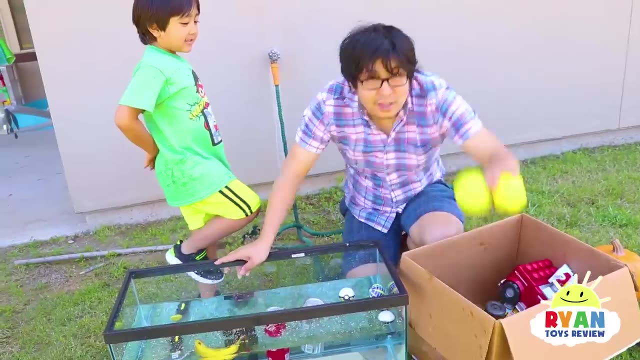 Banana can swim. Ah-ha, Ah, Woo, Oh, like peanut butter jelly. Peanut butter jelly. It's peanut butter jelly time. All right, Daddy, What else should we try? Stress ball, Ooh, Ah-ha. 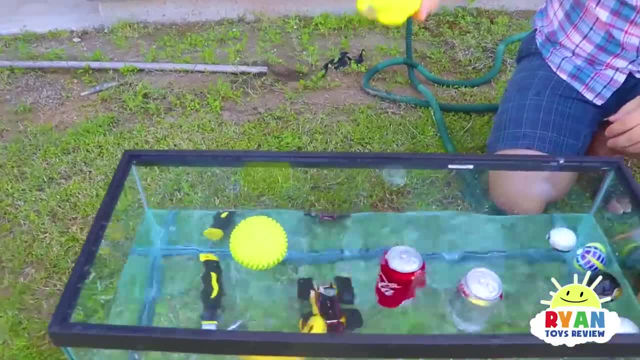 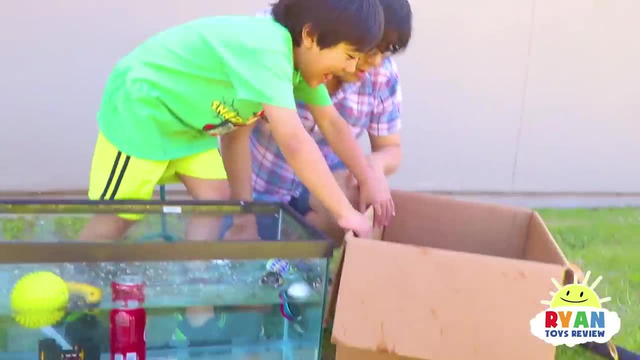 Ah, Oh, Oh, it floats. What about this one? Well, what about that one? Oh, I think those float. Oh float too. All right, Ryan, You're saying what do you want? You know what I'm going to do? 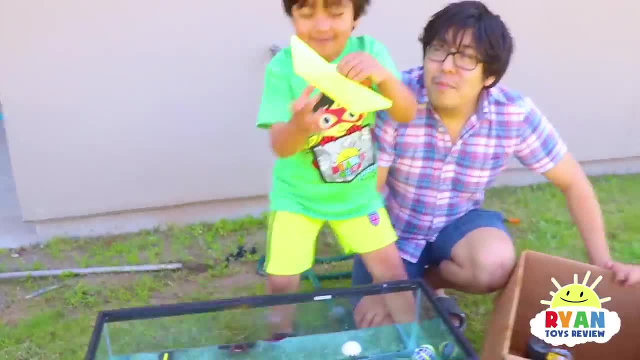 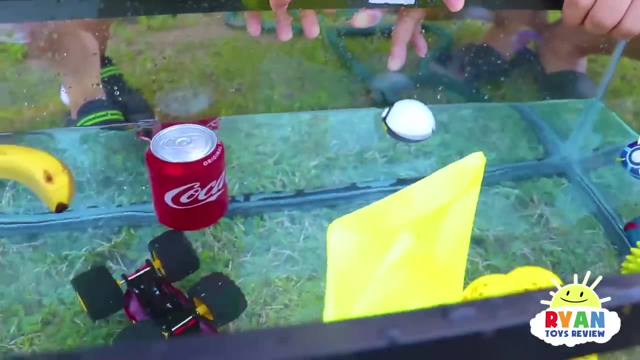 What? Ha-ha-ha? What is that? The boat Ryan made, Oh, boat, Think, or float, Float, Float. OK, Because it's a boat. Yay, Oh, it's floating, Chugga-chugga-choo-choo. 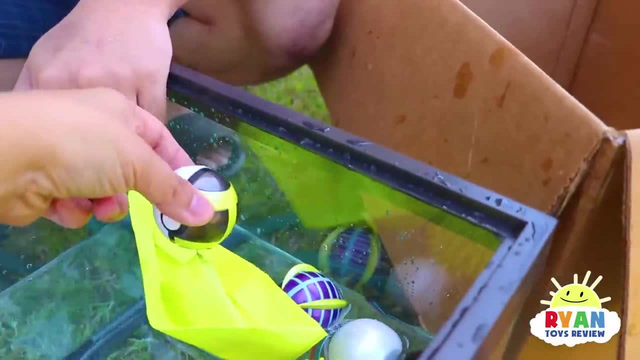 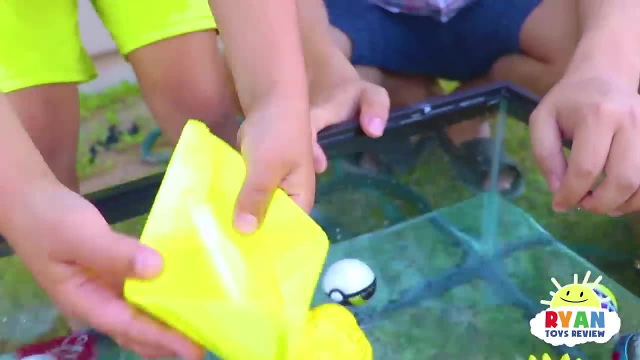 What Is that? a train? What Ha-ha-ha? Why is that sound? OK, What about you think it can hold a ball? Oh no, Honey, it's sinking. There's so much water inside now. 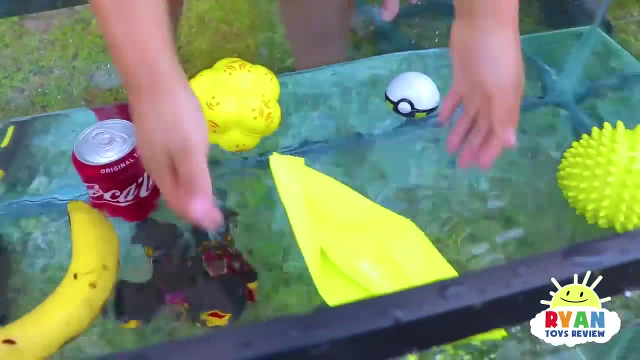 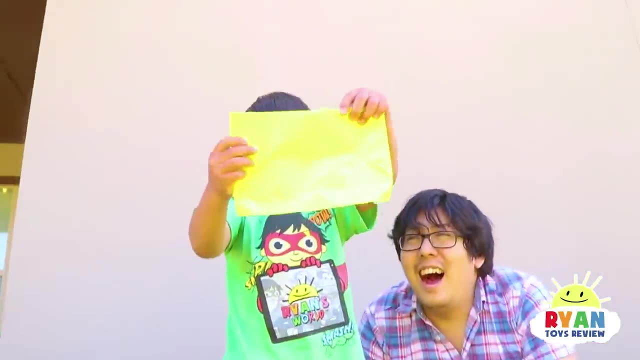 Pokeball overboard? Ah, Oh, no, It's not submarine Ryan. Ha-ha-ha, Is that softball? Ah, it's float. Oh no, no, It's just a sheet of paper. Ah, What about a sheet of paper? 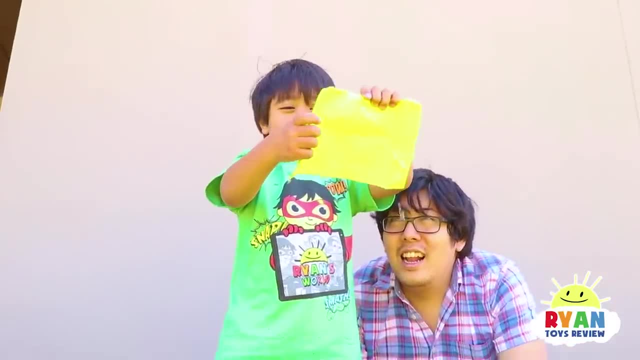 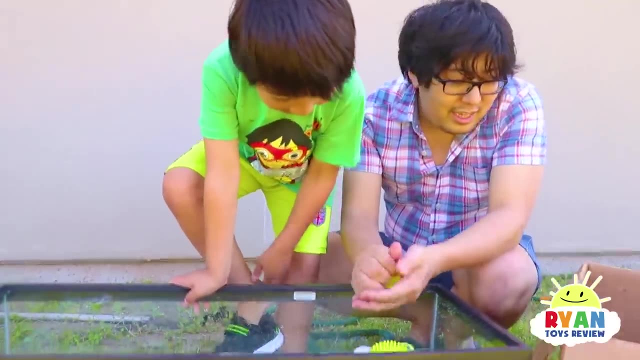 Think: or float. If it's flat, Ah, float, Float. OK, Let's see. Oh yeah, It does float, Ha-ha Float. What about if you crumble it up into a ball Like this? Yeah, 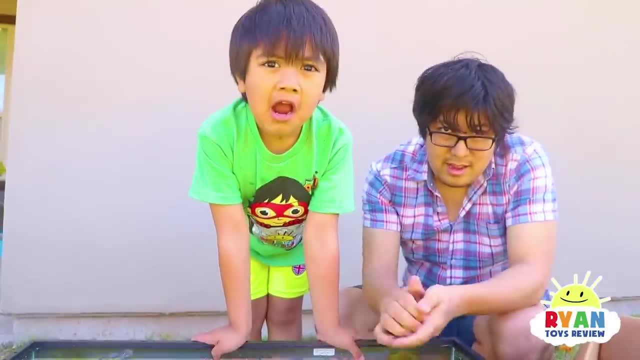 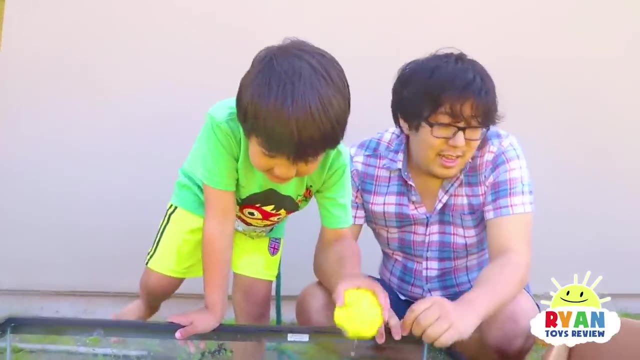 Float, No, sink, But there's nothing in it. Let me see. Oh, there is something in it. Oh, Oh, Oh, It floats. Nope, It floats. OK. What else do you want to try, Ryan? How about this one? 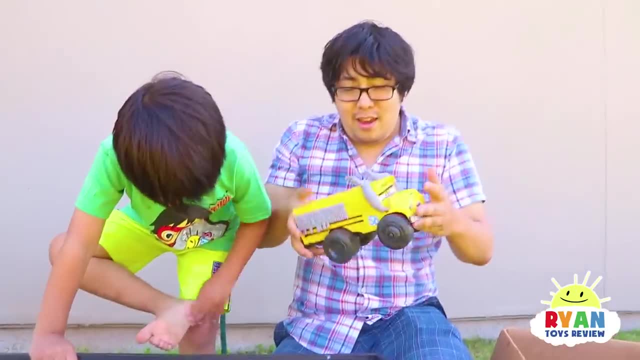 Yeah, Ms Frizzle, All right From Disney Cars. Looks heavy. Let's see, Looks heavy. Sink, sink, sink, sink, sink. It floats, Oh it floats. It's a water toy, Oh, it's a water toy. 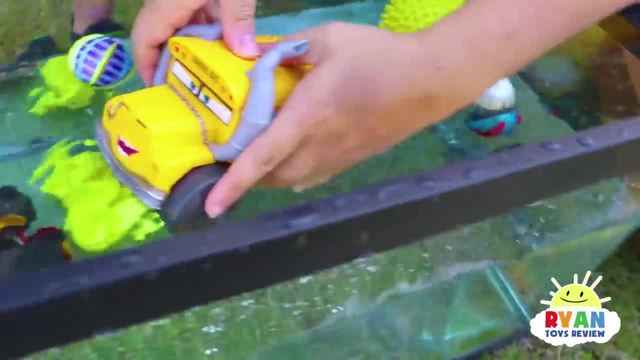 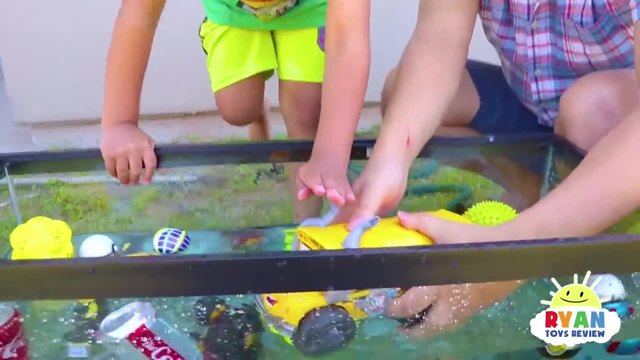 That's why. Oh, so it's meant to float. I forgot. Oh, what's this button? do I think you put it in the water? Let it soak up some water And then it squirts. Ha-ha, You guys see the squirting from the horns. 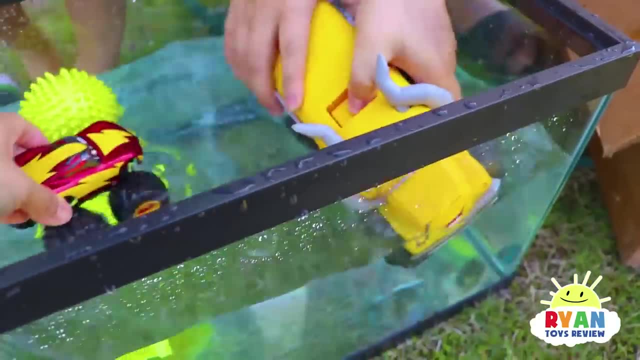 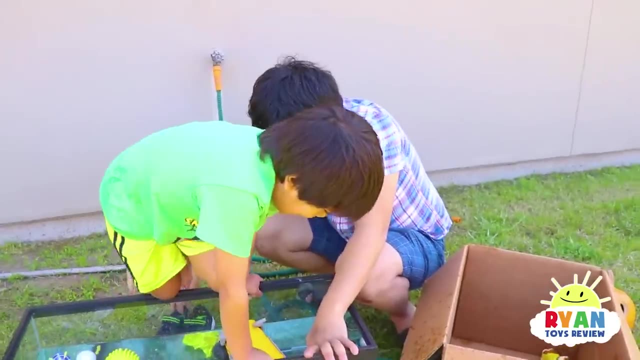 Yeah, The race is on. Whoa, I'm going to splash you, Hey, Hey. no, Don't splash me, No, It keeps splashing my face. What do you want to try next? I want to try Yourself. 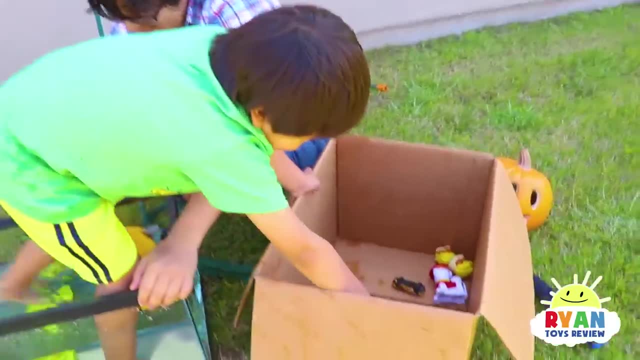 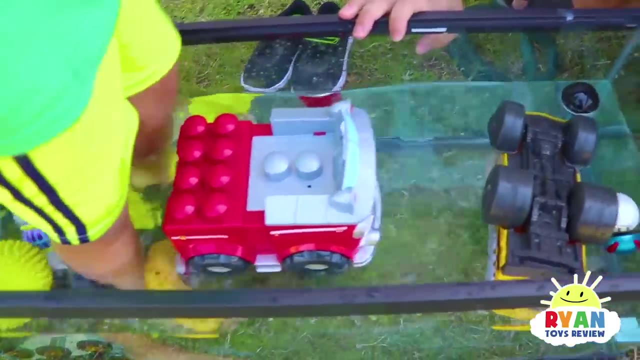 Ryan, Myself Ha-ha, I want to try this. Whoa Got a Paw Patrol fire truck And it floats. Oh, It floats, Even if the Marshall and Rubble here Floats, Still floats, Still floats. 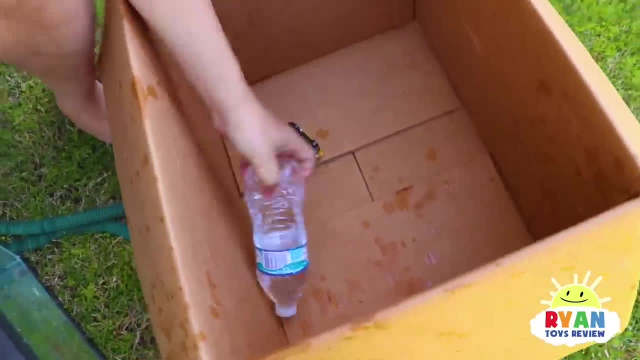 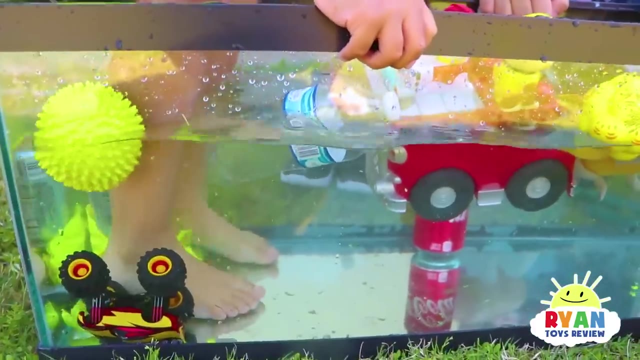 Oh, puppy overboard. What else do we have here? We have water bubble. Take a float, Ryan. Nope, It floats Because there's air inside. Yeah Well, there's a tiny bit Woo-hoo. Last thing: 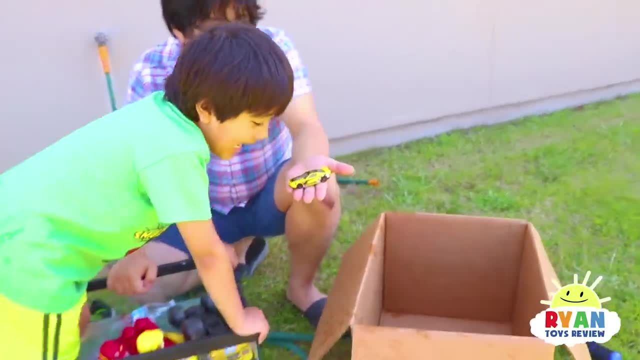 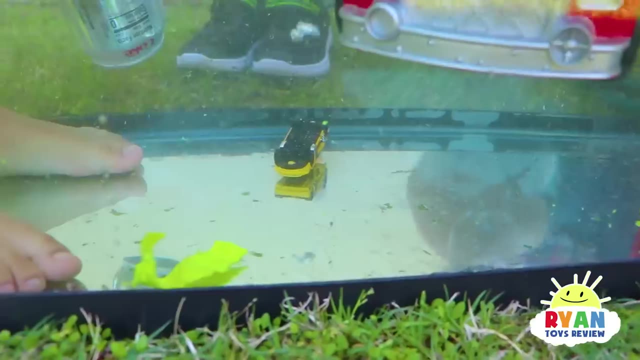 Last thing Is the Hot Wheel. Hot Wheel car Sink or float, Mr Ryan, Uh, Sink, Sink. OK, Ryan says it's going to sink, Ha-ha-ha. Oh, Oh, you're right, Definitely sink. 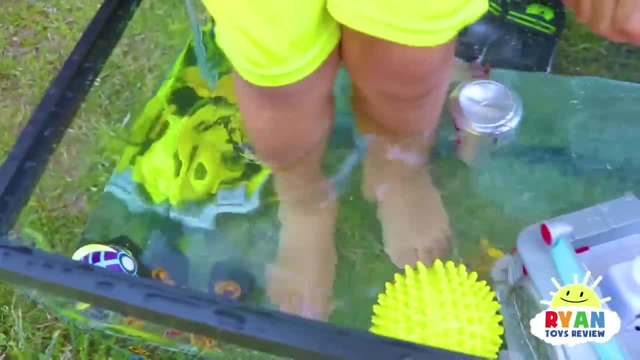 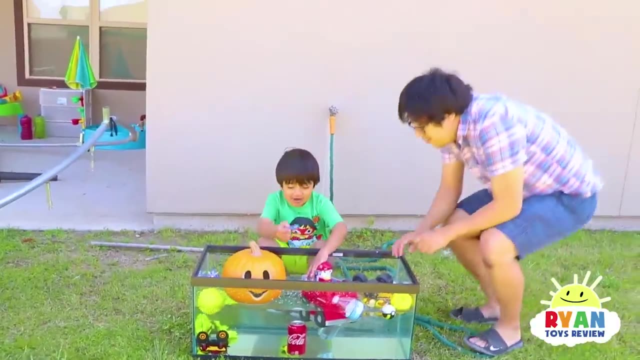 All the way to the bottom. Did you guys guess which one's going to sink or float? I'm a toy. You're also a toy, Ryan toy review. Right toy, Right toy. Now we're going to make the water blue. 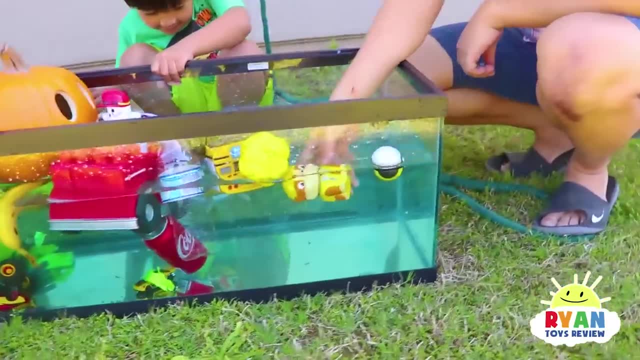 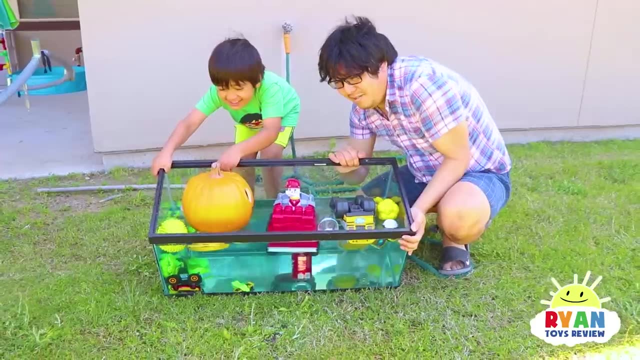 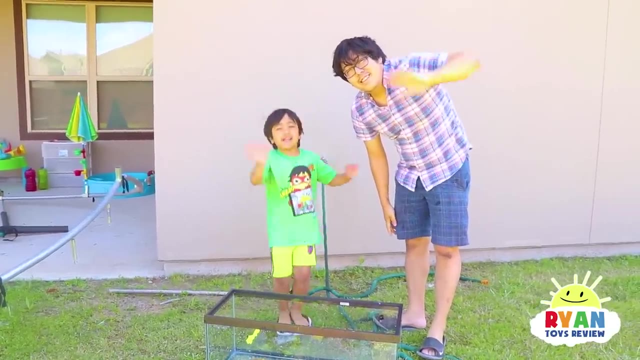 So blue? Yeah, Whoa, Looks like a Rubble at swimming. Rubble, are you swimming, Having a swim? That was such a fun experiment. Now let's dump out the water, Woo Woo. Thank you for watching our science experiment video. 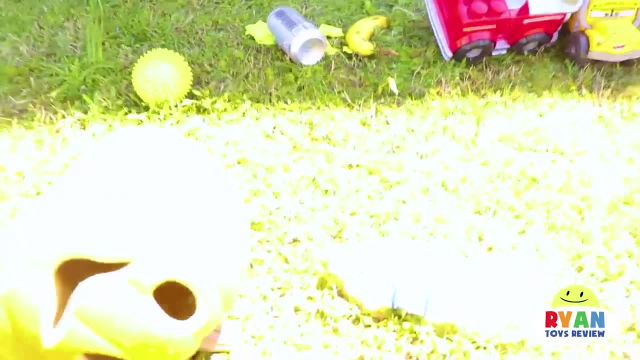 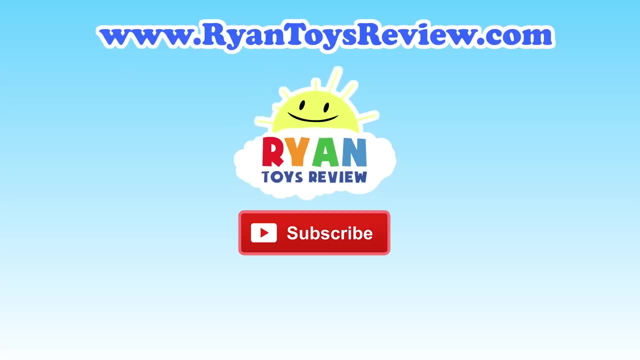 Bye, Bye. We're going to go clean up now And Mr Pumpkin also says bye. Please click on one of these videos for Ryan toy review- more fun. Bye, Bye.